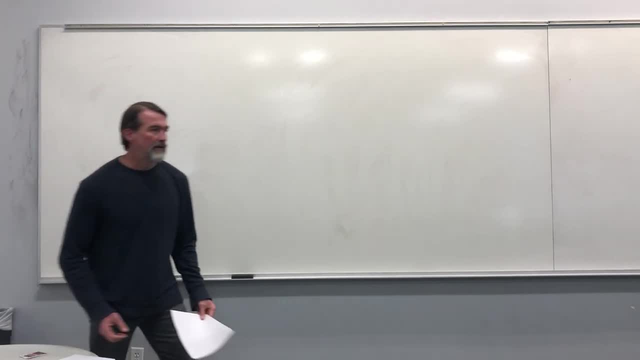 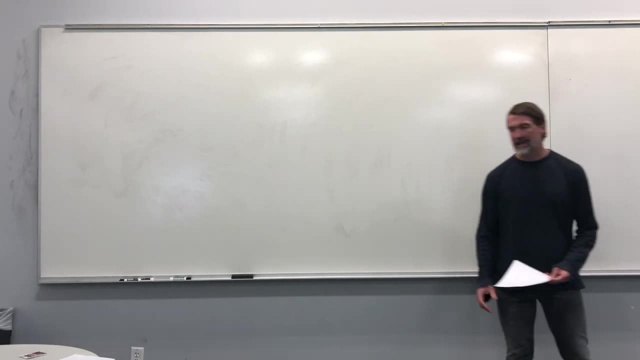 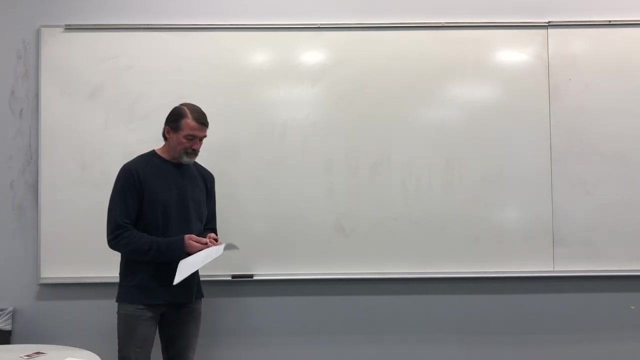 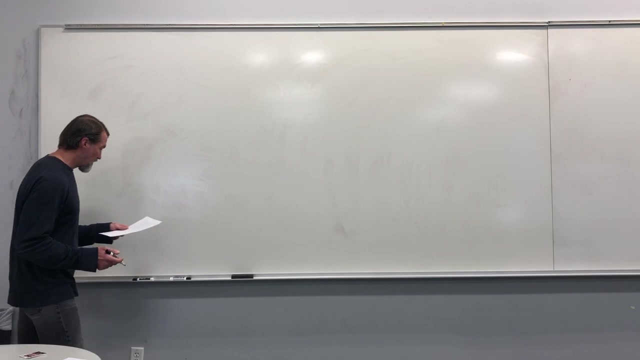 And you know we're going to have some nitty gritty detail. Try and follow it the best you can, but there is going to be sort of a narrative behind it all, So you should understand, at the end of the day, what the issues are and how the Higgs mechanism or what we're going to need the Higgs mechanism to do. Okay, Are there any questions? before we get going? This could be a long one, so I just want to go ahead and get started. Okay, the weak interactions: These are what we're going to talk about today. 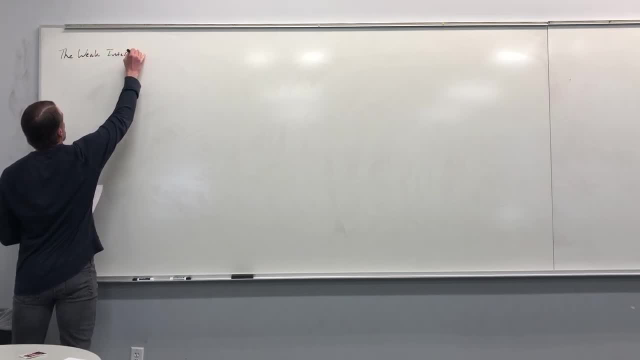 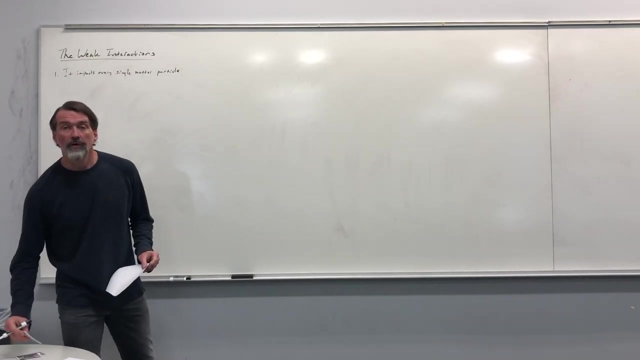 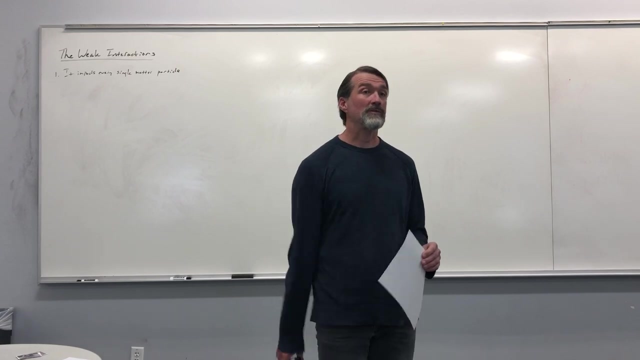 The weak interactions have several characteristics which set them apart from the other interactions. The first quality of the weak interactions is that it impacts every single matter, particle. Let me ask you, Jared, which particles does the electromagnetic interactions impact? Charge particles, Charge particles, And there are neutral particles, the neutrinos- Okay, Quarks are charged. They're electrically charged. We'll learn about that later And 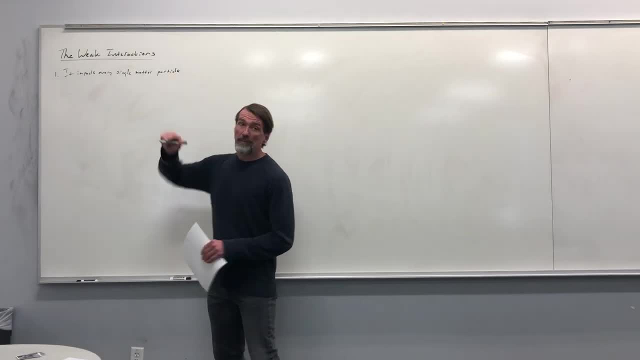 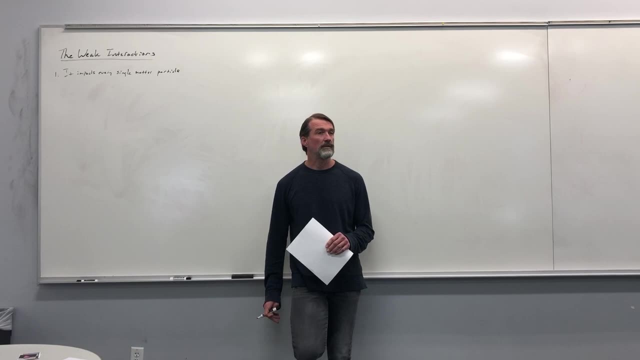 we have three charged leptons, but we also have three non-charged leptons. What about the strong interaction, Shaylee? what particles do the strong interactions impact? Axon particles, Say again, Axon particles. I don't know. 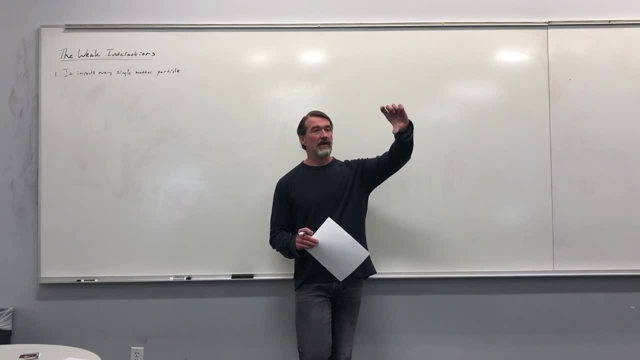 So the particles include the leptons, which are the electron, the electron, the electron neutrino, the tauon, the tauon neutrino, and the muon, the muon neutrino. And then there's the quarks up down, strange top, bottom. 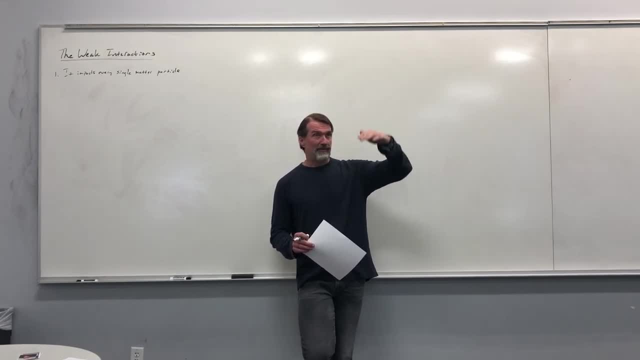 So there's, Okay, 12 particles. Which of those particles do you think experience the strong? the color interactions? strong color interactions? Oh, the quarks, The quarks. yeah, Maybe it was me saying strong versus quantum chromodynia. 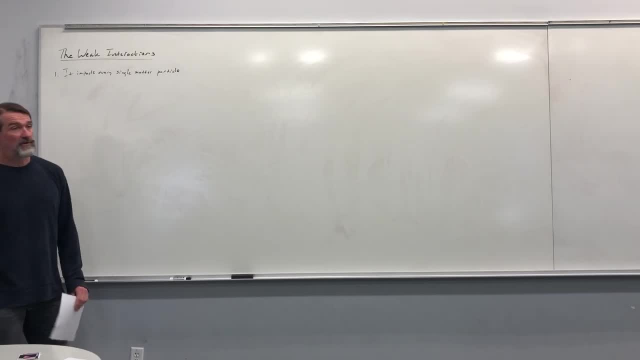 Yeah, so notice, electromagnetism only affects a handful of particles. QCD, the strong interactions, only affects a handful of particles. The weak interaction- that's what's so damn funny about it. it's called the weak interaction. it affects them all. 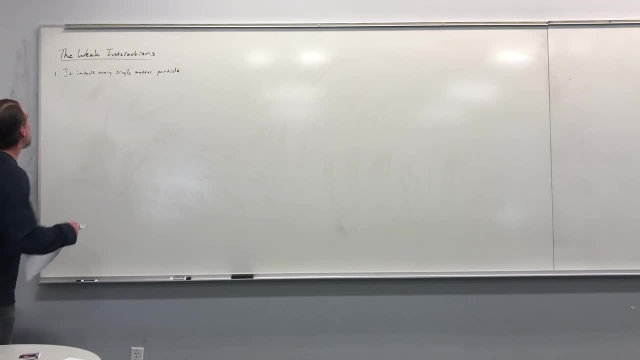 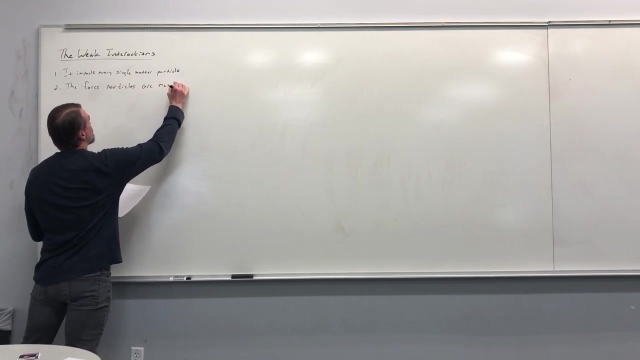 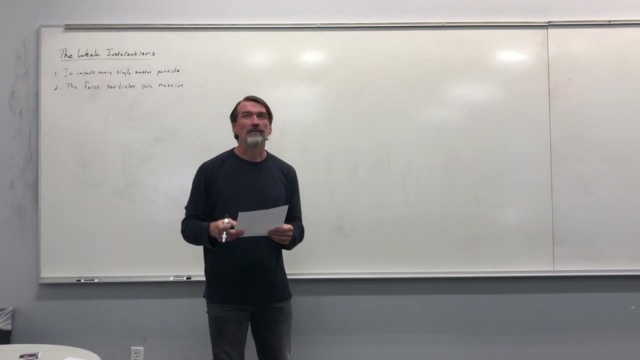 That's what's so weak about it, Not Okay. Second interesting quality of the weak interactions: The force particles are massive. Okay, So wait a minute. hold on. The photon is the electromagnetic force particle. Is that massive? No, it's massive. 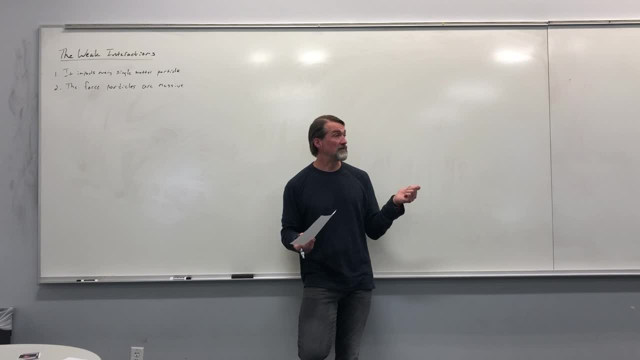 Okay, The gluons are the force particles for the strong interaction And, even though I didn't talk about it last time, they are massless as well. Okay, And again, the argument is that the Lagrangian for the mass, for the force particles, is the Proca-Lagrangian. And the mass term in the Proca-Lagrangian breaks, whatever symmetry you're trying to impose. So the only way the symmetry could be true is if the force particles are massless. Okay, But for the weak interactions the force particles are actually massive. It violates a bunch of symmetries. It violates parity, charge conjugation and the combination of those Cp, charge conjugation and parity And, perhaps most importantly Okay, the weak interactions can change the flavor, ie particle type. 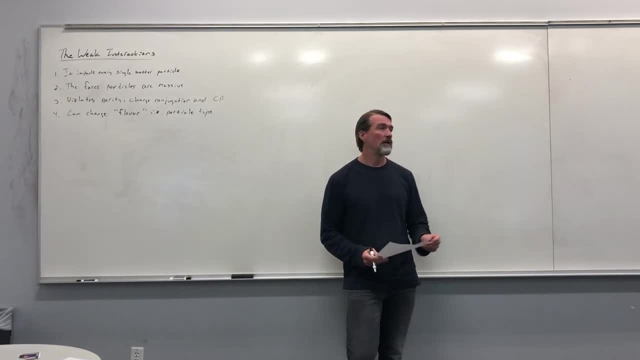 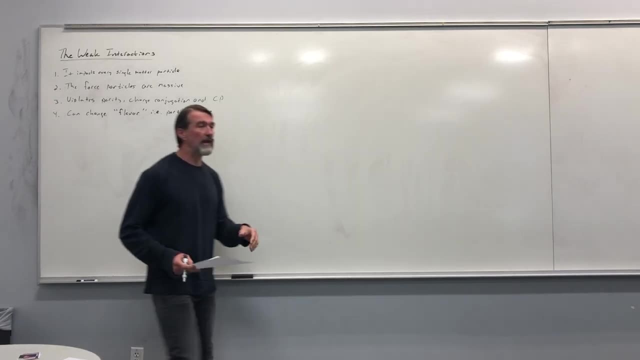 Okay, That is, we can start off with an electron and that through the weak interactions it can turn into an electron neutrino. Okay, With some other stuff in the game, But the importance of that is that this is what leads to decay. Because when we talk about decays, we're talking about particles which are there And then they go away by turning into lighter weight particles, So you actually change which particles are there when you have a decay process. The weak interactions are the only thing that can do that. 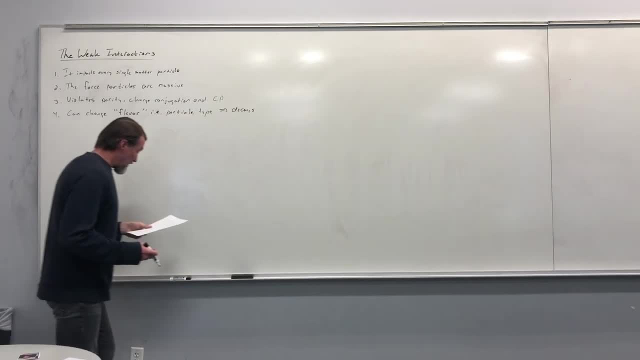 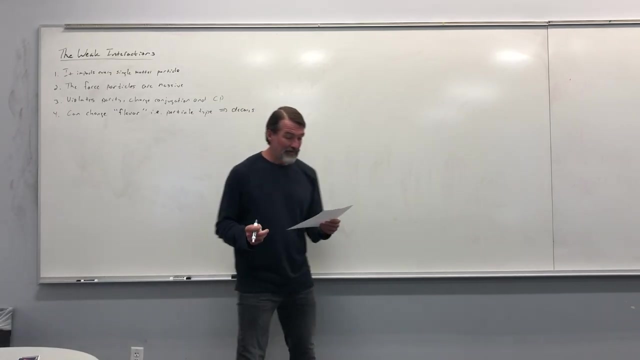 Okay, All right, These are four really interesting aspects of the weak interactions, But by no means is any of them as important as the weak interactions. But by no means is any of them as important as the fact that the weak interactions are not based on a symmetry of the standard model. 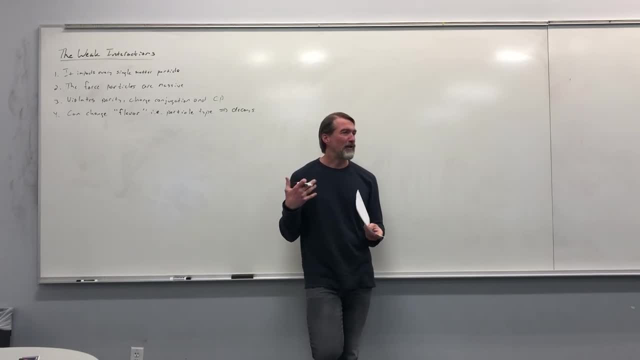 Wait a minute. I was blowing smoke up your nose over the last couple of lectures where I was claiming that every interaction in the standard model comes from a symmetry principle. right, You start with a global symmetry and then you basically localize it And that gives rise to the interactions. 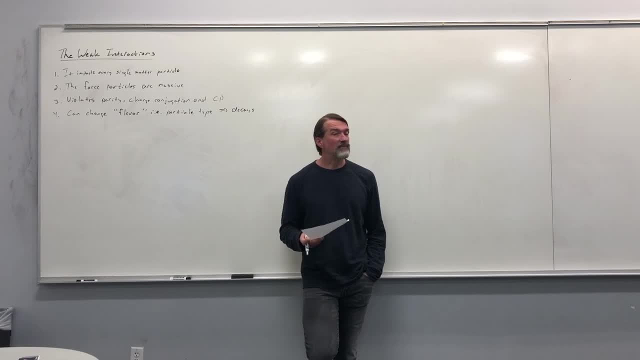 Okay, We did electromagnetism, We did the strong interaction. Both of those stories worked out. I would now argue to you that the weak interactions do not represent a symmetry of the standard model. Does that suck? It doesn't follow that same story. 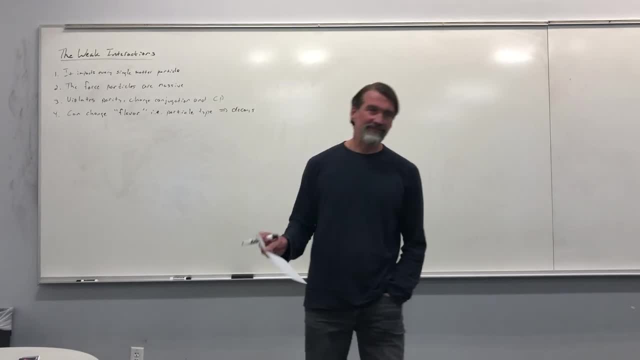 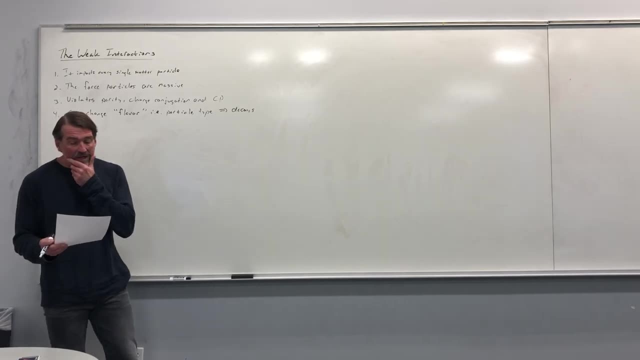 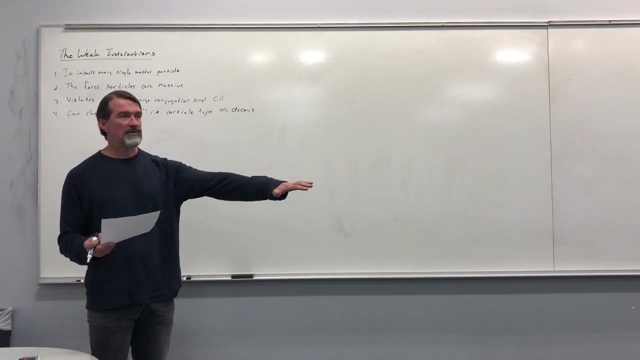 But it turns out that there's a little bit of conditions that I have to say Okay, Right now, at room temperatures, the weak interactions do not express a symmetry. However, earlier in the universe, or at high temperatures or high energies, there is a symmetry underlying the weak interaction. 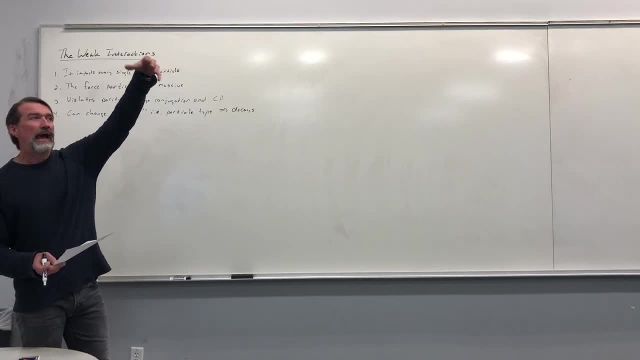 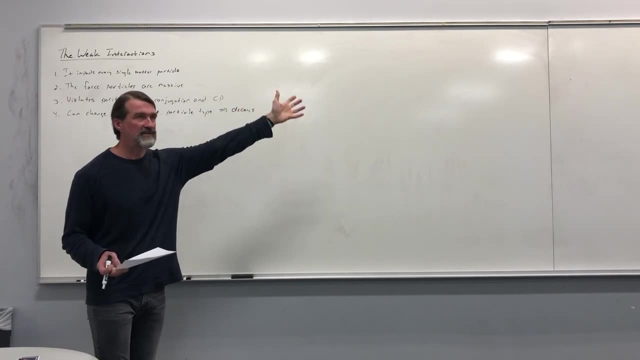 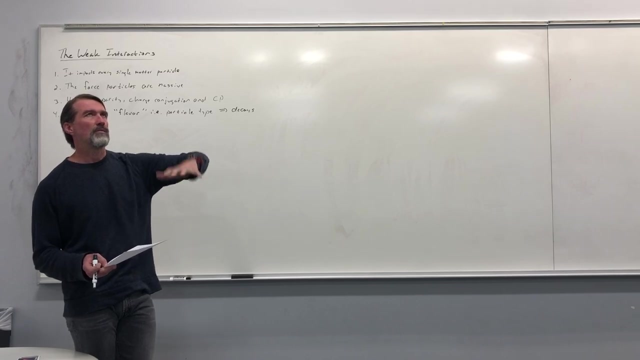 Okay, So we have a symmetry at some scale, Energy scale basically, Back in the early universe it was a high energy scale as well. We have a symmetry argument, but now we don't What I mean. the symmetry there had to disappear. 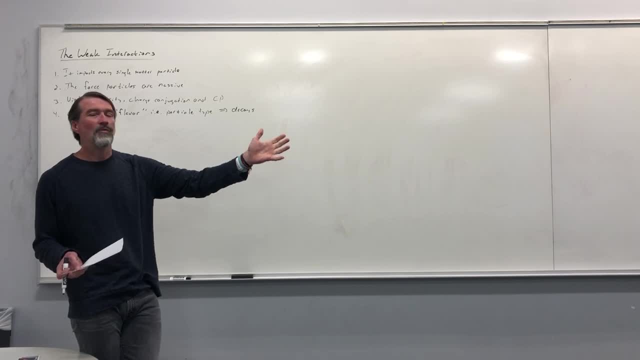 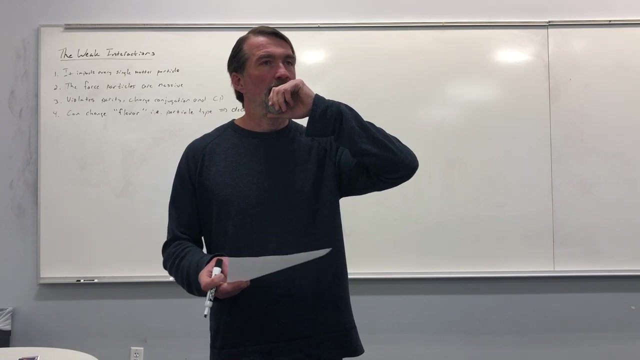 What? That's something called the Higgs mechanism, which we're going to talk about next time. Okay, But that's going to play an incredibly important role in the elimination of this symmetry. Yes, Do the energies of the strong interactions and the electromagnetic depend on any type of temperature or anything? 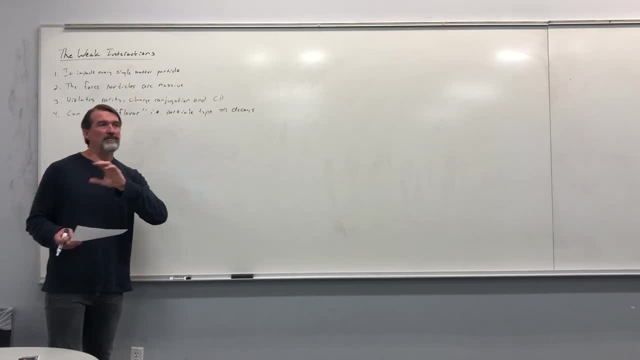 No, Well, actually electromagnetic will in just a moment, But the strong interactions don't Okay. Well, I mean, everything depends on the energy scale. That's a topic called renormalization, which we'll learn later on. But the symmetry underlying the strong interaction seems to go to high energies. 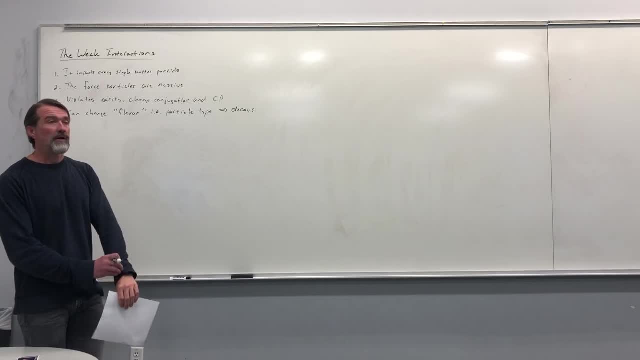 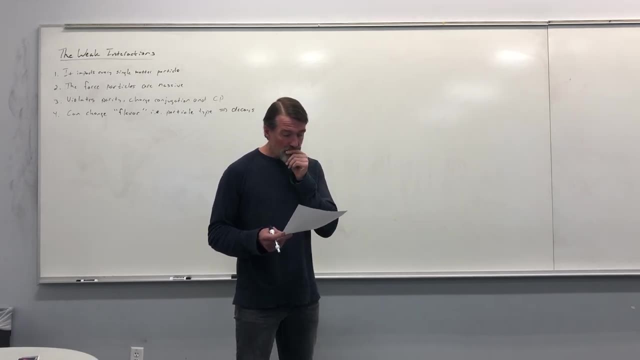 The features of it will change as you change the energy scale, but the symmetry is still good. But just wait on electromagnetism, because that's going to be part of this story. Okay, Okay. So here's what we're going to do. 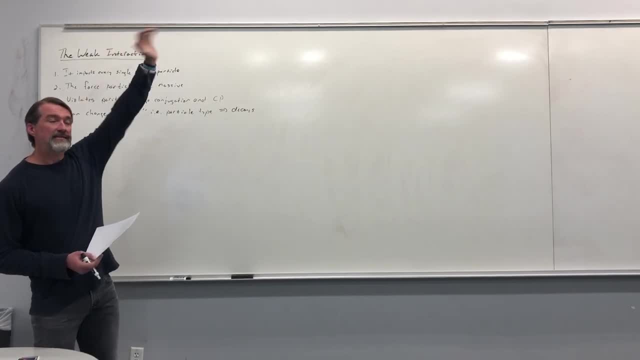 Since the weak interactions start out at a symmetric thing in high energies, we're going to go ahead and approach this at the high energy level, so we can use our symmetry argument- the same symmetry argument we use for electromagnetism and strong interaction, And we'll just formulate what it looks like. 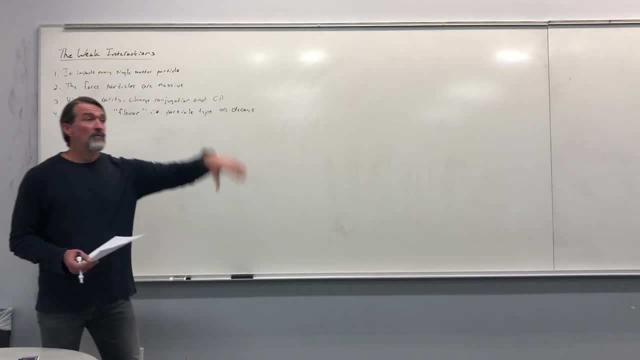 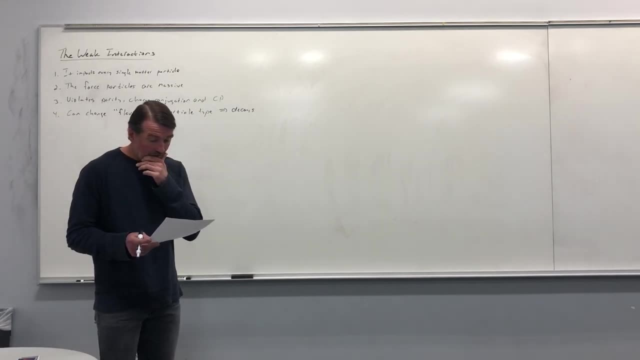 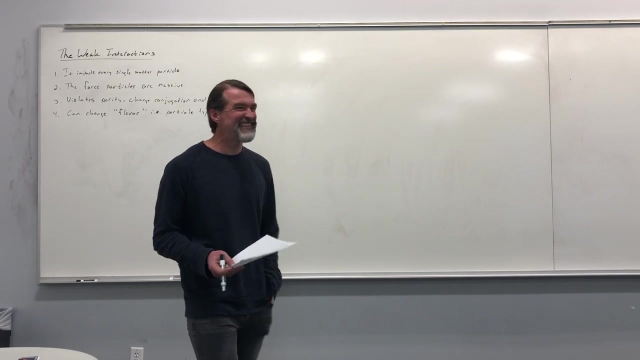 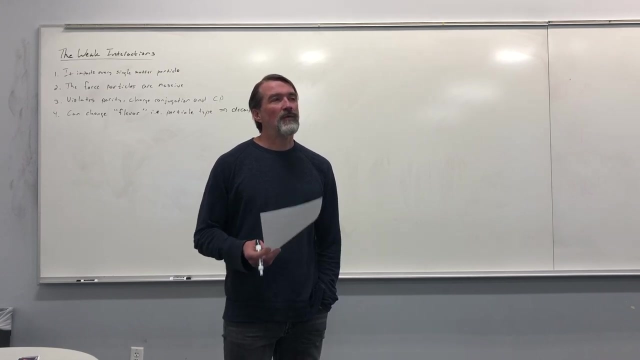 Then, when we bring in the Higgs mechanism, we'll figure out how that symmetry is broken and you know the result and so forth. Okay, Oh wait, There's something else amazing. This is such an awesome topic. It turns out that if you want the weak interactions- 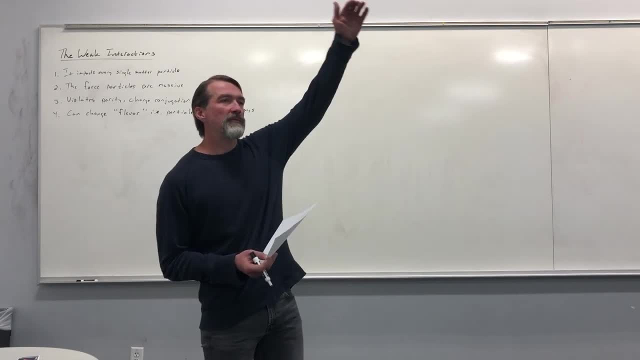 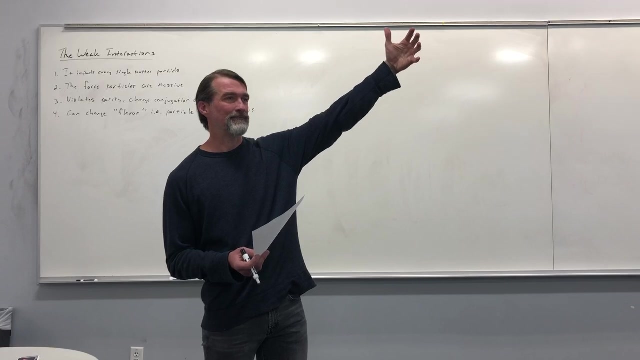 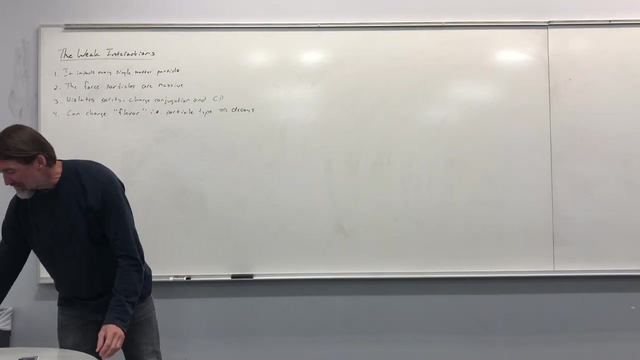 to be the result of some symmetry at higher energies. the weak interactions have to be unified with the electromagnetic interactions in a very non-trivial way, And we're going to talk about that today, Okay, So what the hell do I mean when I say electro-weak unification? 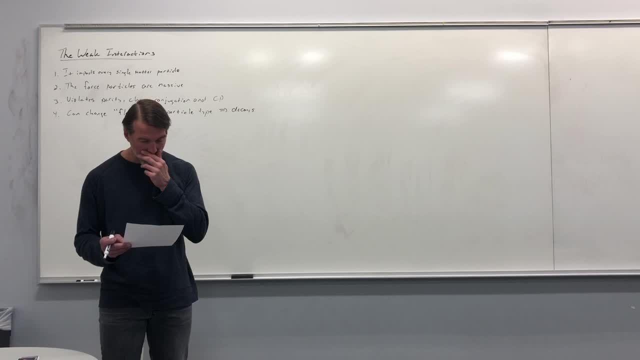 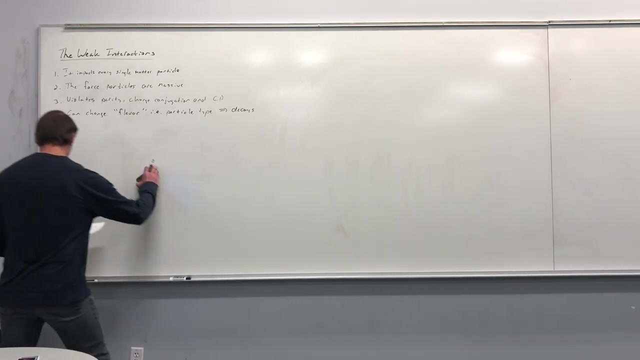 That is, the unified force, The force of electromagnetism and the weak interactions. Let me just make sure there wasn't something else I wanted to say: Yeah, Okay, So electro-weak unification, Okay, So we're just going to forget about the weak interactions by themselves. 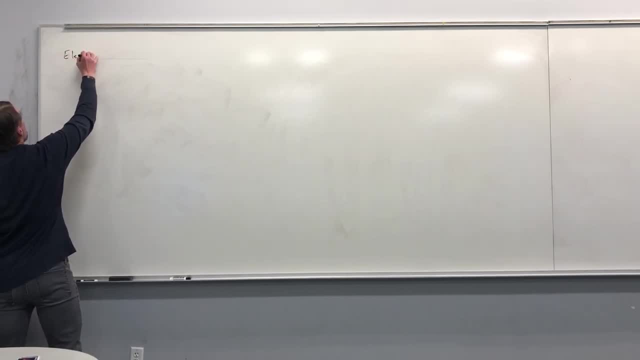 and we're going to talk about electro-weak unification. Okay, Now, many of you have heard it. I've probably said it, but I just want to be more careful. It is often said that the symmetry group of the standard model 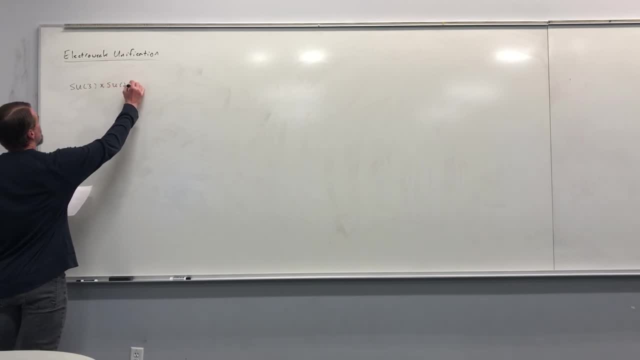 is SU3 cross SU2 cross U1.. Okay, Where, when we look at this, as we've already gone over, magnetism is built on localizing the U1 transformation, So we might say that that's E and M. 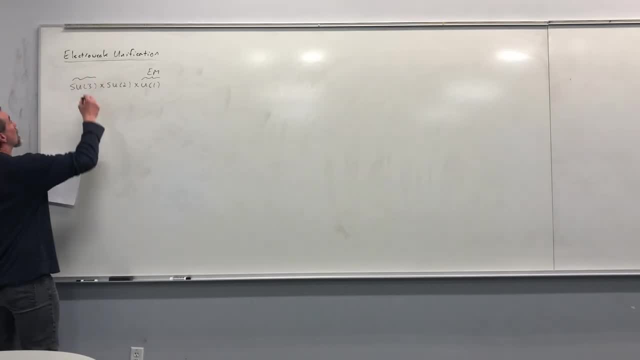 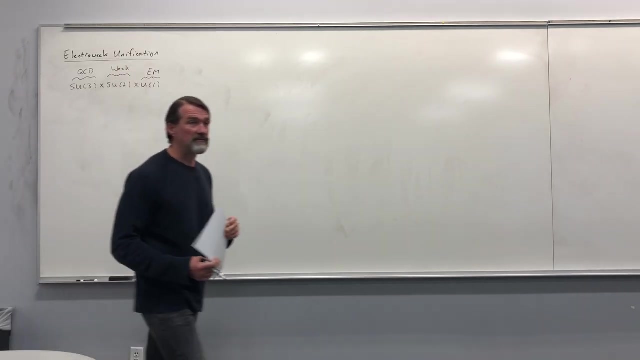 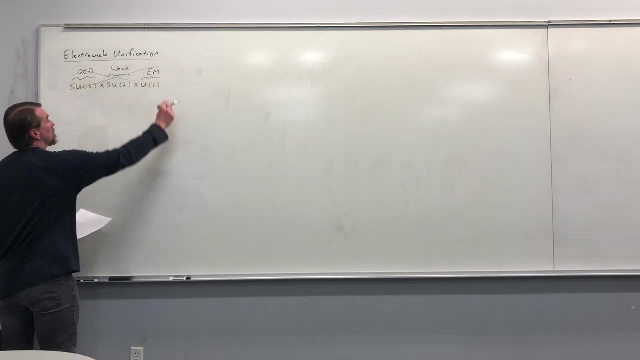 And then SU3 is the symmetry group underlying quantum chromodynamics. So this is the strong interactions. Okay, That leaves as a natural candidate for the weak interactions. this, right here, Okay, Makes sense, right? Okay, This is crap. 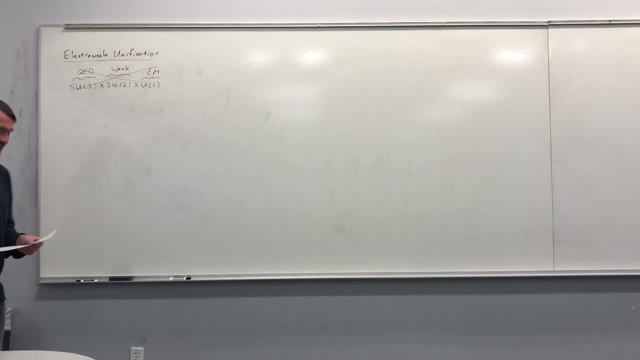 Any questions? Okay, So this is actually the correct group, Any questions? Oh, I forgot a couple of things. Okay, We're going to talk about what that L means and we're going to talk about what that Y means. 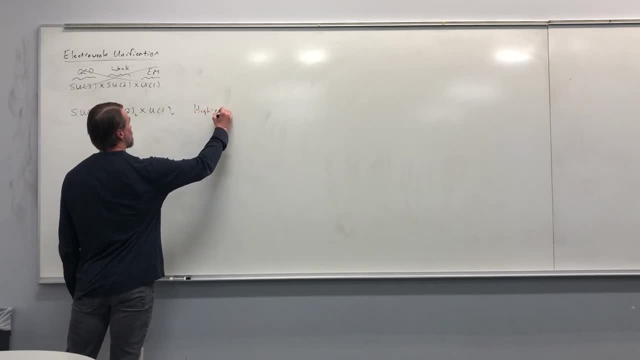 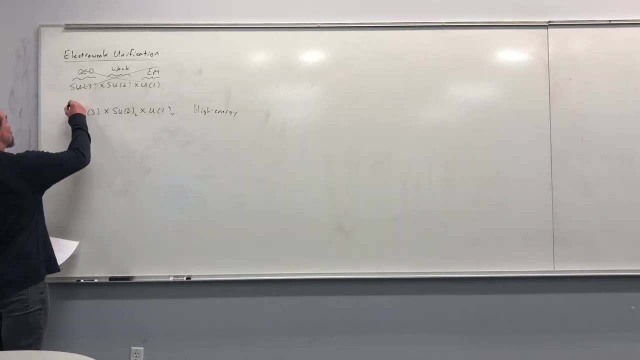 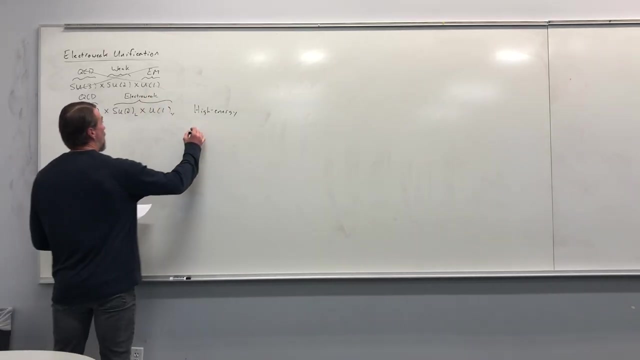 But this is the high-energy group structure which underlies all of the standard model. This is the underlying group for quantum chromodynamics. as we expected, This is the underlying group structure for the electroweak interactions. Okay, When we go to low energies? 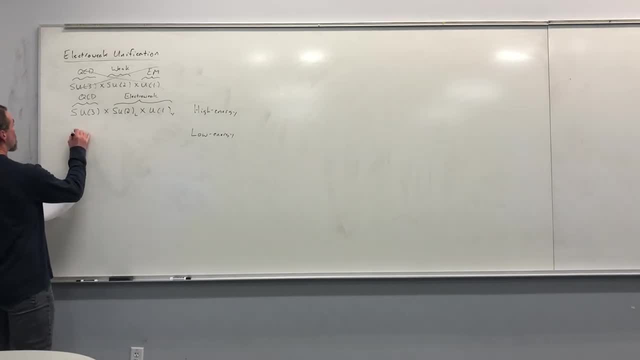 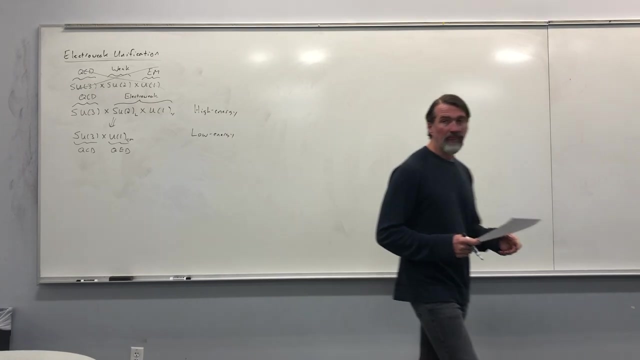 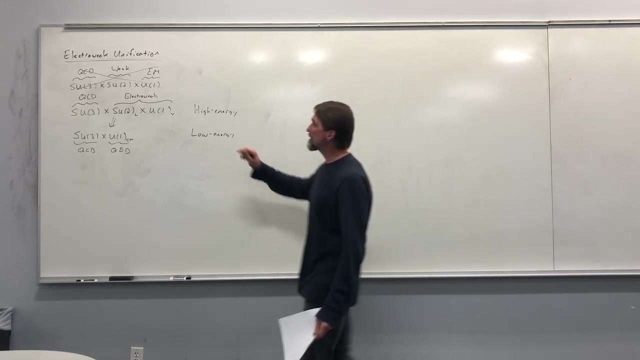 like a room temperature. this gets broken into SU3, cross, U1, where this is the electromagnetic U1.. Okay, So again we have QCD and then QED. So in order to figure out the weak interactions, we have to start with this electroweak unified group. 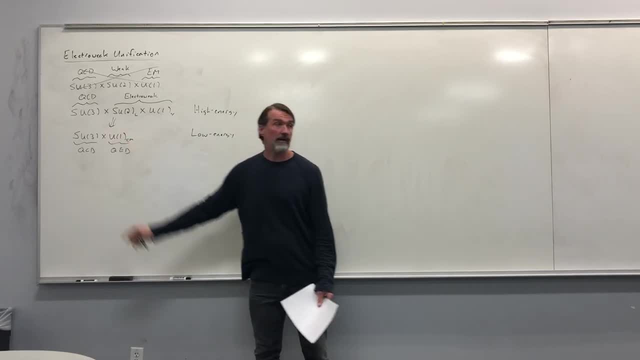 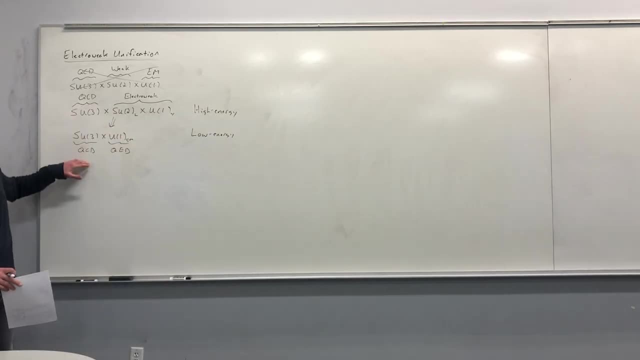 And then the Higgs part of the story will tell us how it gets down to here. Okay, So we don't need to worry about QCD in today's talk, because you know this is just a completely independent thing, All right. 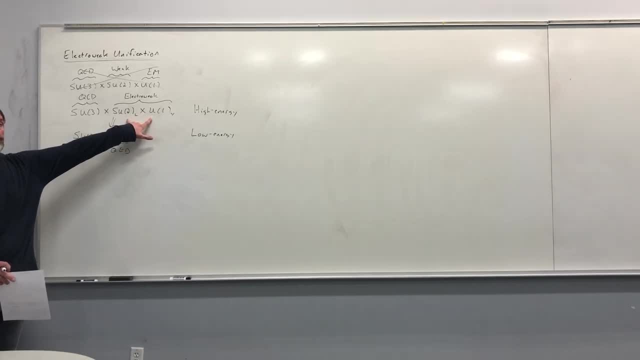 So we're really going to focus on SU2L cross U1Y. All right Now. PJ, PJ, Sergio, Sergio, What do you think the L means Right? Yes, It means left. Good, That was a good answer. 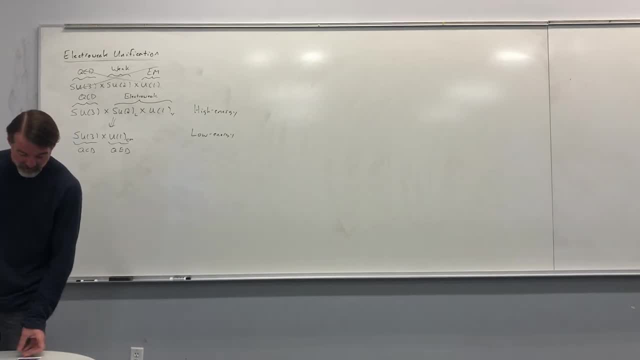 This is regards to chirality, which we'll talk about in a minute. Sean, What do you think Y stands for? Well, this is L for left. This is Y for Hypercharge. Awesome, It's the second letter of hypercharge. 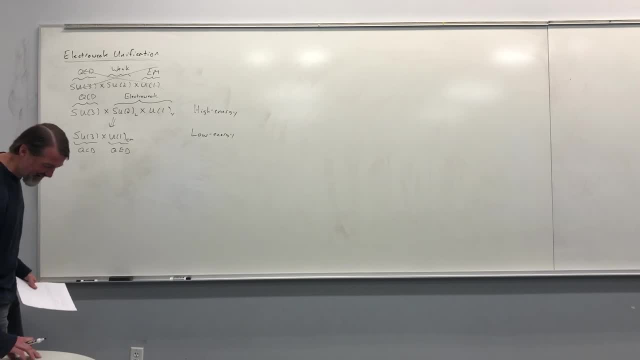 It's obviously Y Dang man. You guys are tearing it up today. No, I'm just kidding. Okay, So the L here stands for left-handed fermion states. Wait, What is a left-handed fermion state? 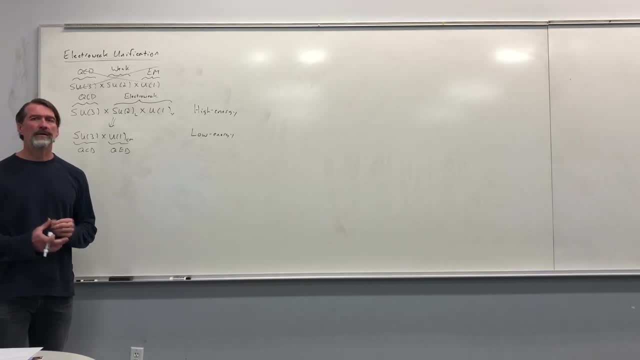 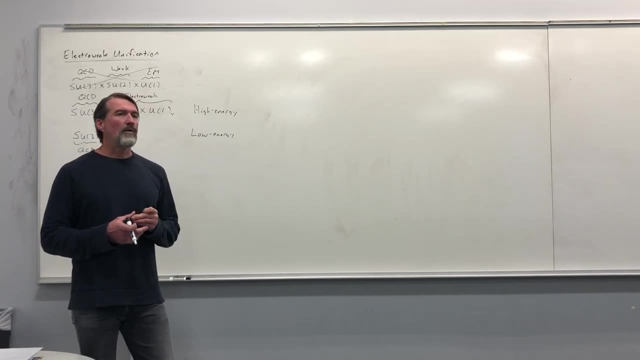 What do you think left-handed means? Anybody, It's a twisted electron. Well, what have I talked about over the last few lectures, where I talked about the handedness? Is it a left-handed? Well, there's right and left-handed coordinate systems. 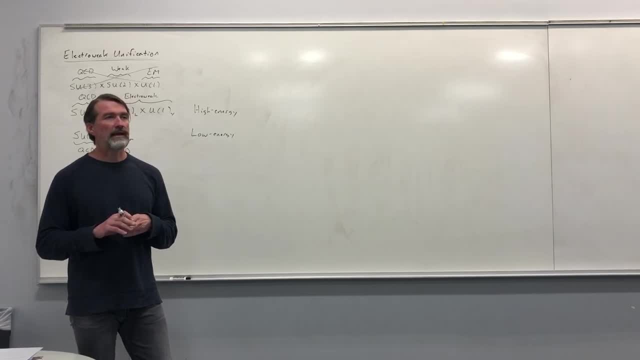 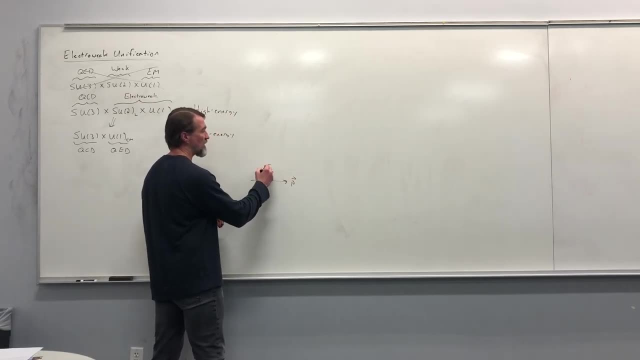 but we're talking about particle properties. Does anybody remember my helicity story? You know, if I got a particle that's moving with some momentum P and its spin is a long P, then it's got a right-handed. And if the spin is anti to P or, sorry, anti to P. 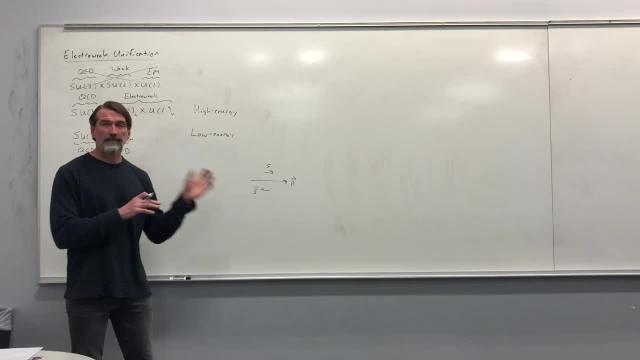 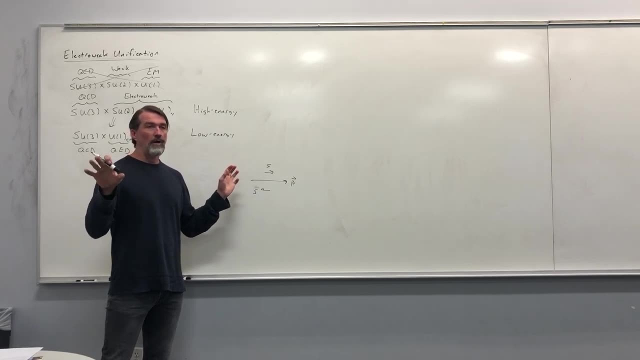 then it's left-handed. Do you guys kind of remember that? Doesn't that only like matter for massless particles though? Well, so that's the interesting thing. This notion is fine for massless or massive, but if for massive particles it can be the – okay. 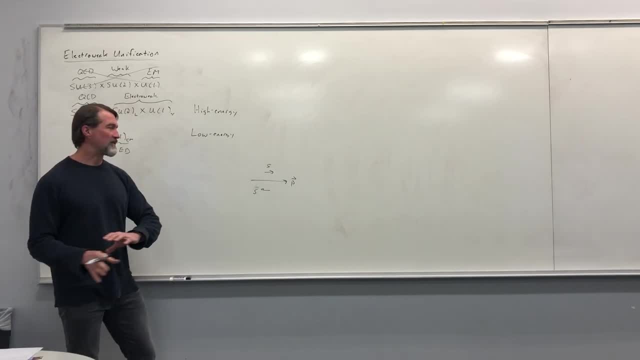 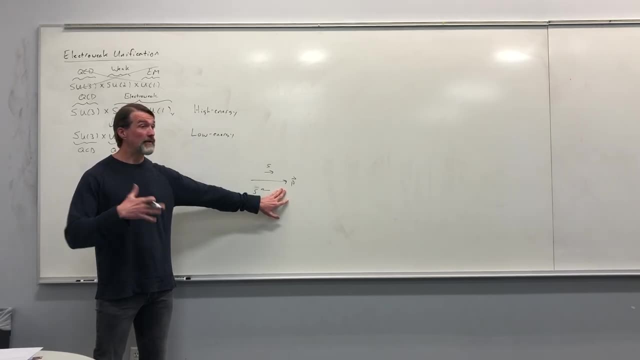 So let me just give you the words, and then I'm going to go back to their distinction. What I'm talking about here is helicity. It's how the spin aligns with P, How the spin aligns or anti-aligns with the momentum. 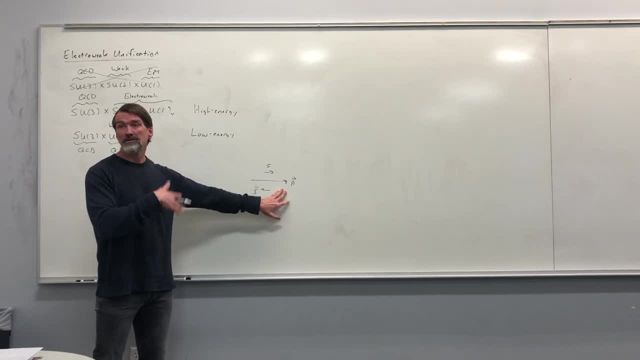 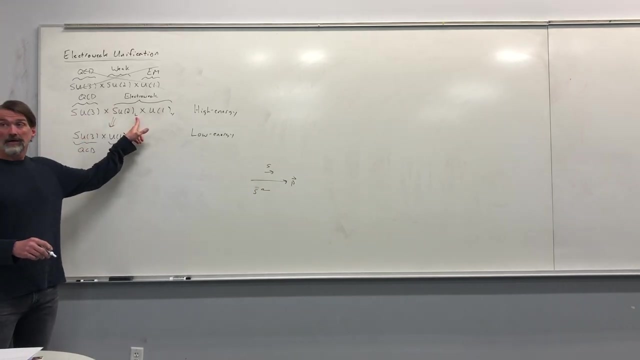 For massless particles it's invariant For massive particles. you can always change the direction of the helicity. okay, And we use left-handed and right-handed to describe this. Does this make sense? We're using left-hand here out of tradition. 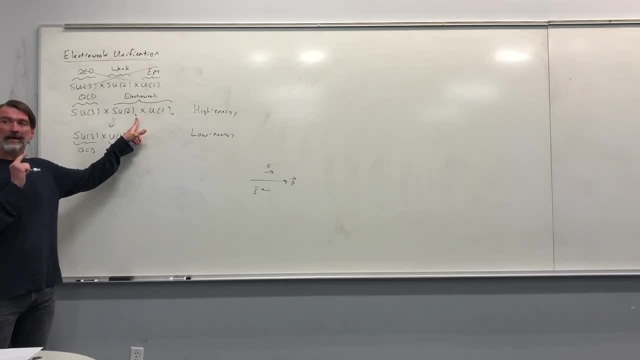 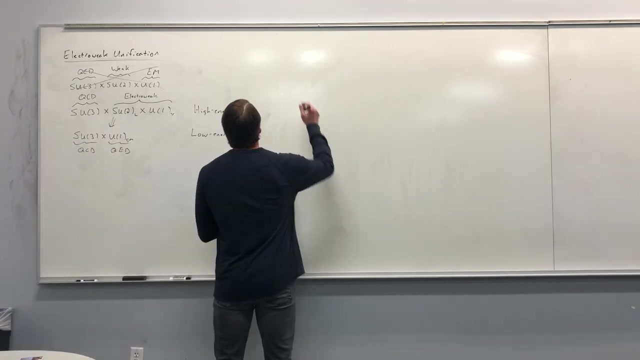 It has nothing to do with helicity. This is actually chirality, not helicity. Okay, Now that could be a little bit confusing, so let me revisit and clarify the difference between helicity and chirality. So if we started with a spinner psi –. 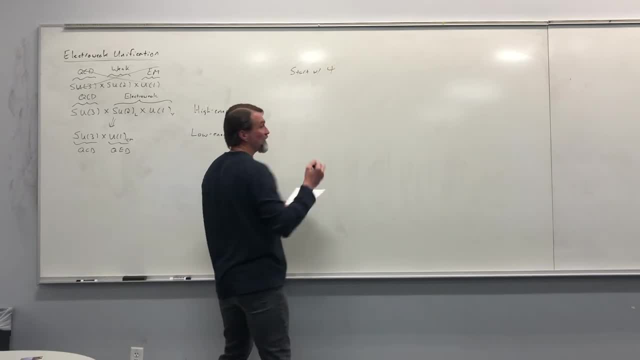 okay, this is just an arbitrary spinner – then we can do two different projections on it. We can do one-half one plus s – or plus-minus sp on psi, and that's going to give us something which we could label with a plus-minus. 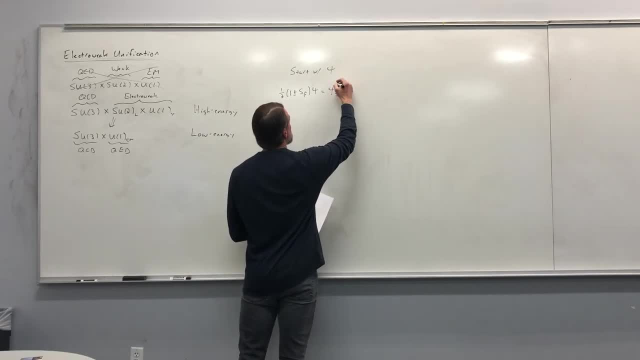 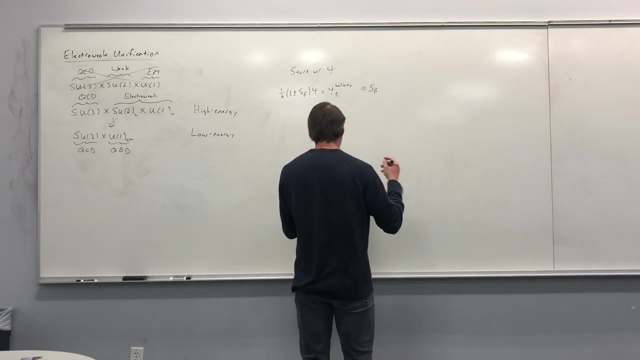 which corresponds to the choice there, And this is a state of definite helicity. Okay, That is, if I act on a state with definite helicity, with the spin – this component of spin along the momentum – then I'm going to get back plus-minus h-par over 2 psi-helicity plus-minus. 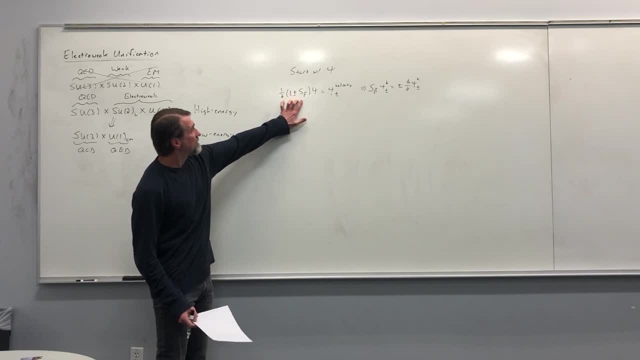 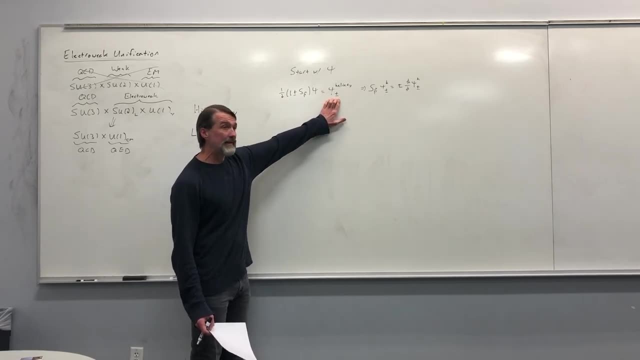 So if I take an arbitrary spinner and I project it with this operator which you built in your homework last time, then you're going to get helicity eigenstates plus or minus, which are basically the eigenstates of the spin operator. 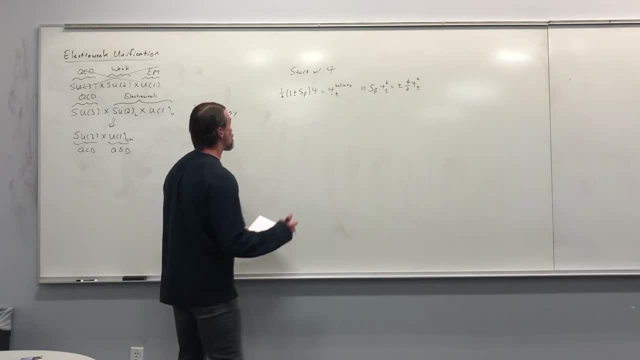 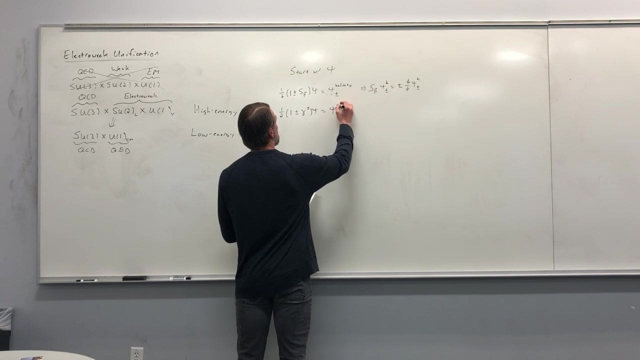 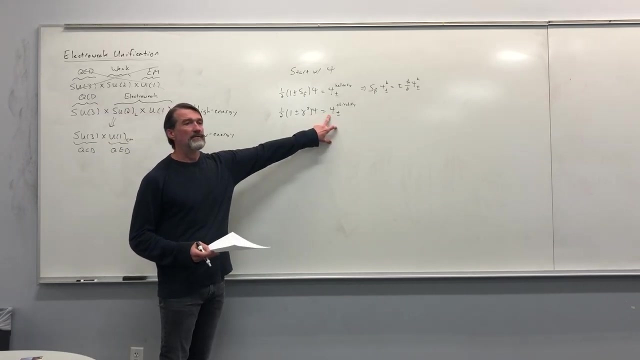 with eigenvalues plus or minus h-par over 2.. Okay, Alternatively, I can take this same generic spinner and I can project it with the gamma-5 matrix. Okay, In this case, what you get after that projection are different states of chirality. 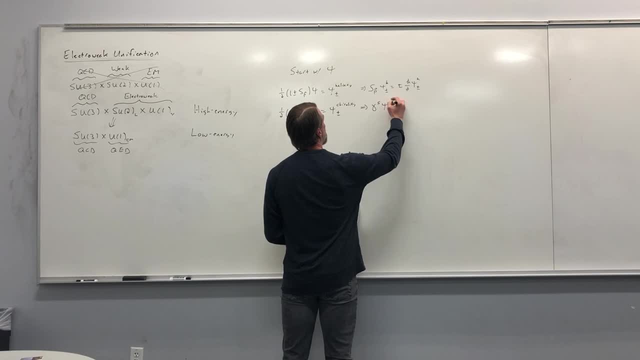 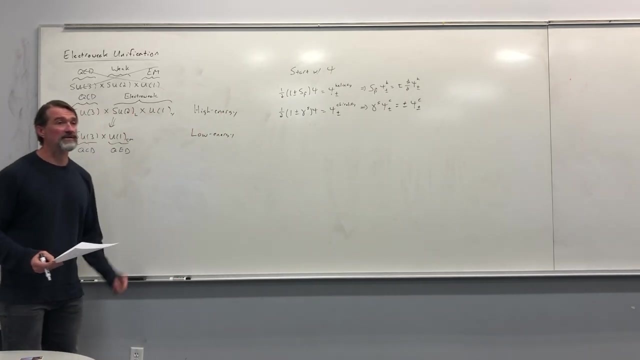 Hence, if I act on a chiral state with the gamma-5 operator, I'm going to get plus or minus the chiral spinners back. So these are eigenspinners of the gamma-5 matrix. Okay, So just notice. 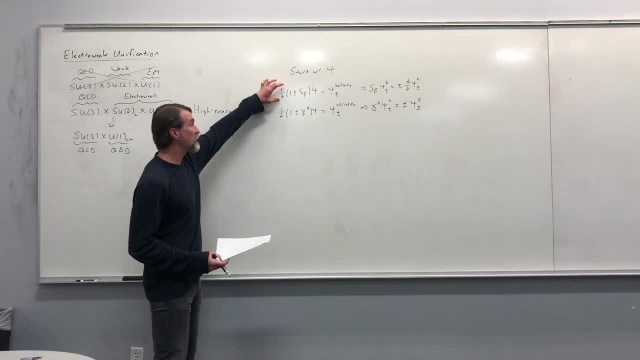 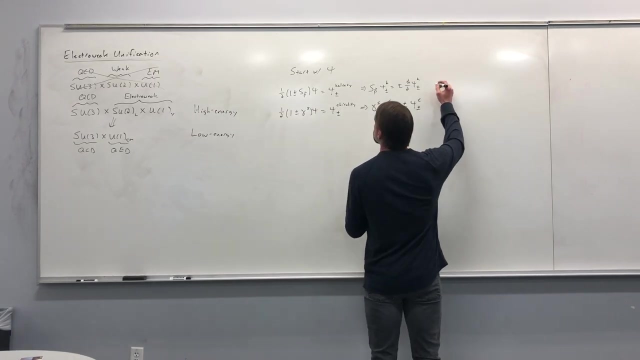 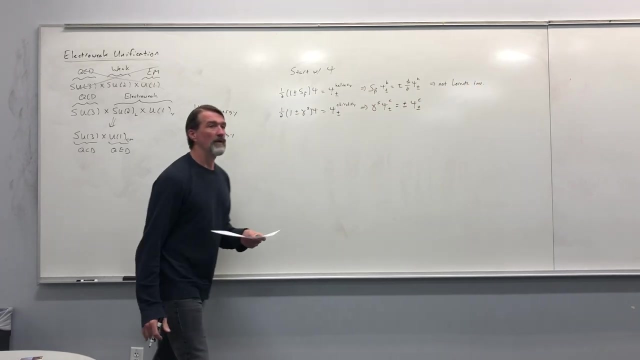 helicity is defined in this way with this projection operator. Chirality is defined in this way with this projection operator. Okay, There are even more differences. Okay, If I consider helicity, then helicity is not Lorentz invariant. 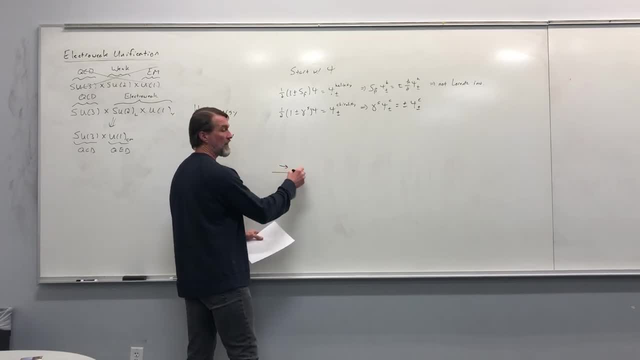 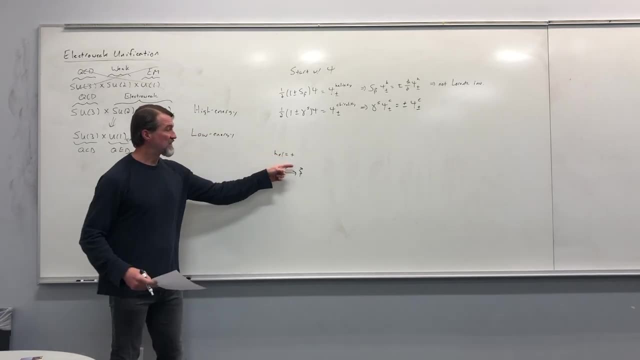 But remember, when we talked about helicity, we said: oh, that's the spin and its alignment with the momentum. And so if you have a plus-helicity state where the spin is aligned with the momentum, you can just do a Lorentz transformation. 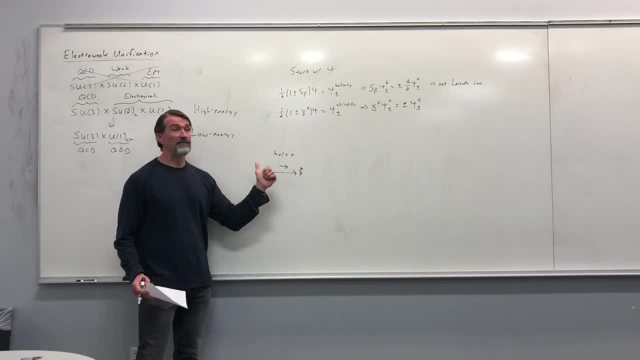 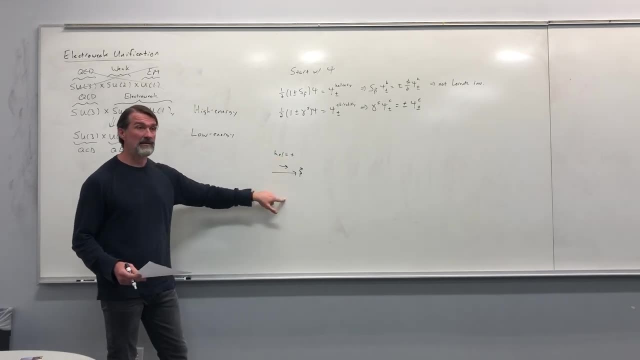 and reverse the direction of the momentum by boosting to a frame such that this motion is backwards. That doesn't change the direction of the spin. So you can do a Lorentz transformation to change the helicity to minus. Okay, So helicity is not Lorentz invariant. 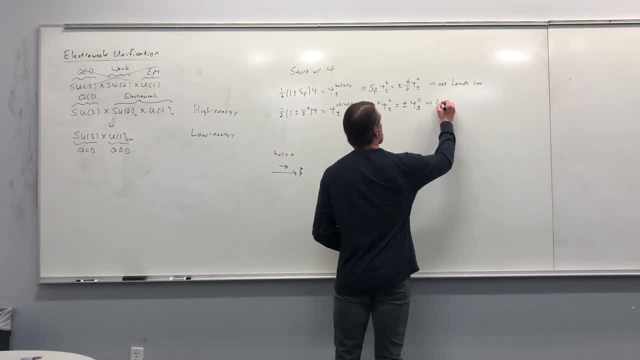 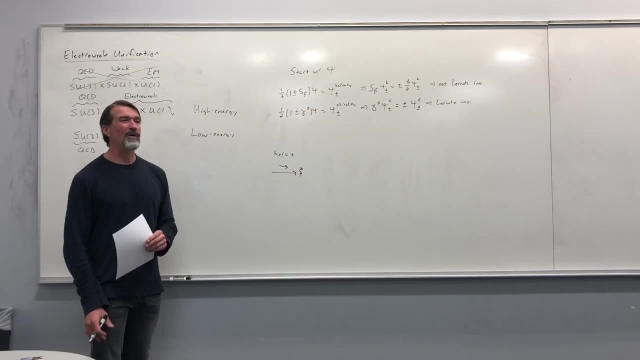 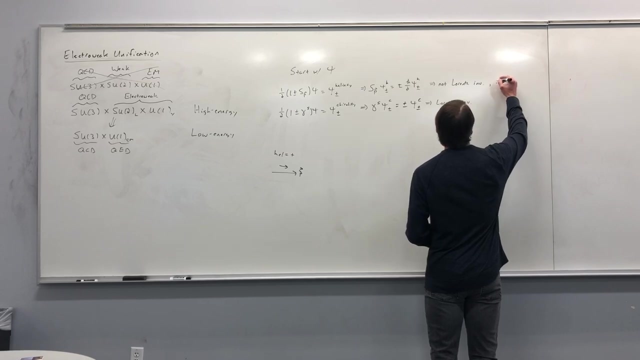 Chirality is. Now you might say, oh, chirality wins. Well, not entirely. Whereas helicity is not Lorentz invariant in a frame, it is unchanged. That is if I just pick a reference frame. 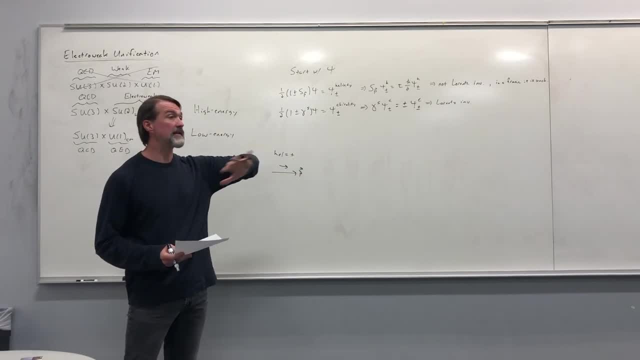 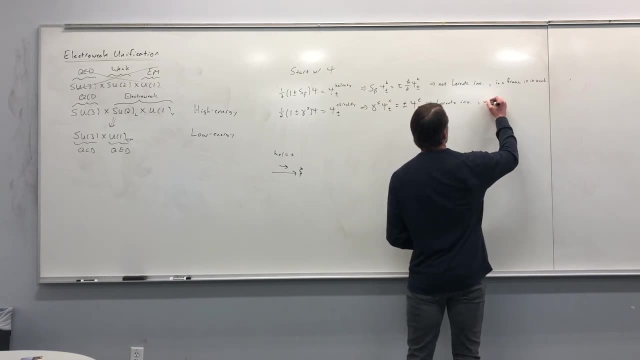 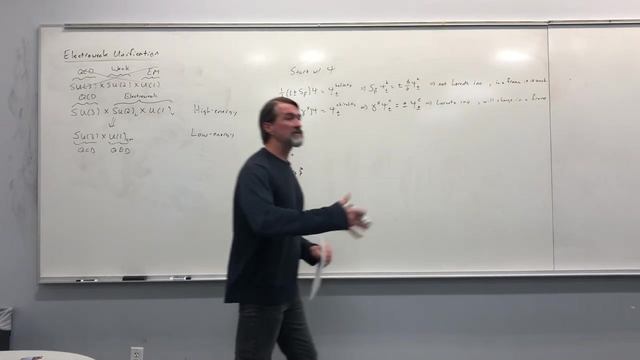 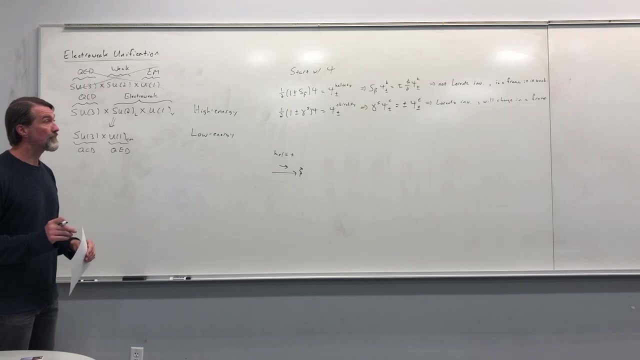 and watch the motion of the particle and look at its helicity. its helicity will not change, Okay, Whereas the chirality will change in a frame. So the chirality can actually change its value without touching the reference frame, Okay. 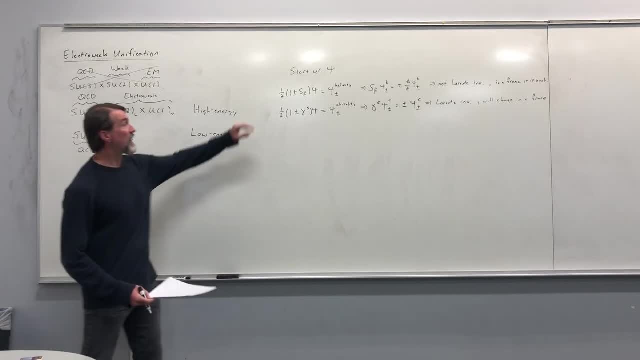 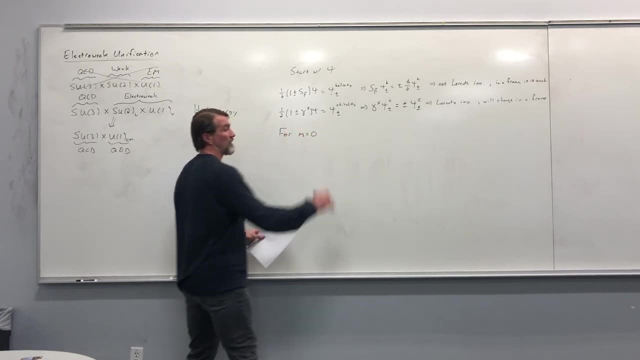 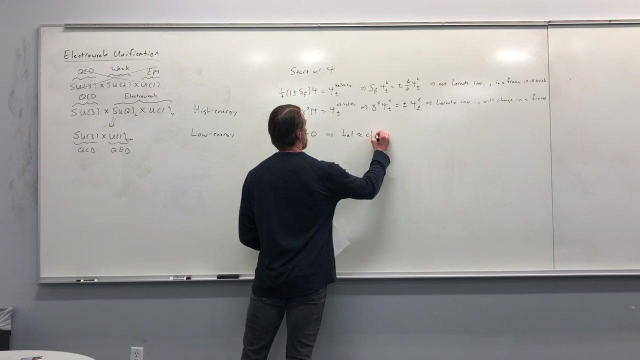 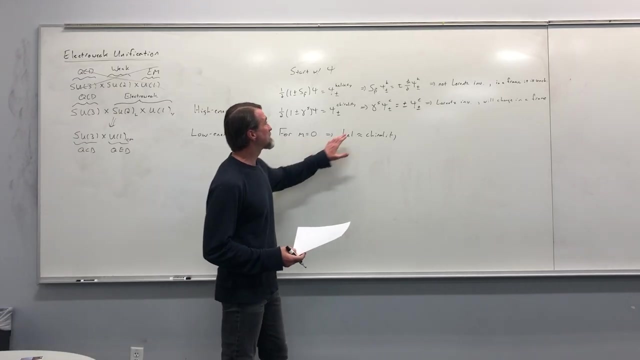 Now, here is where it can get a little confusing. but I just wanted to start out with these very different stories first. Okay, If a particle has zero mass, then helicity is basically the same as chirality, It turns out. if a particle has zero mass. 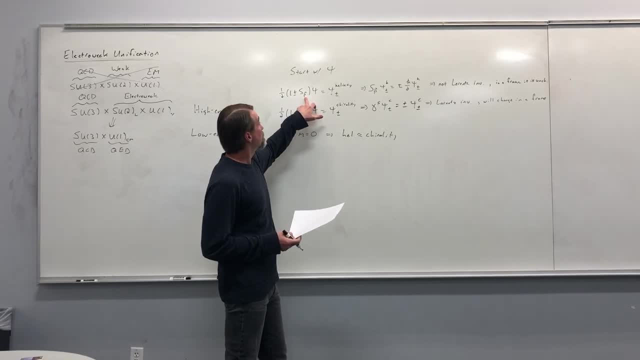 and you use this projection to the helicity, then you'll get an eigenstate of spin and this will also be an eigenstate of gamma-5.. I argued this in a couple lectures ago. I actually wrote down the spinner that's projected. 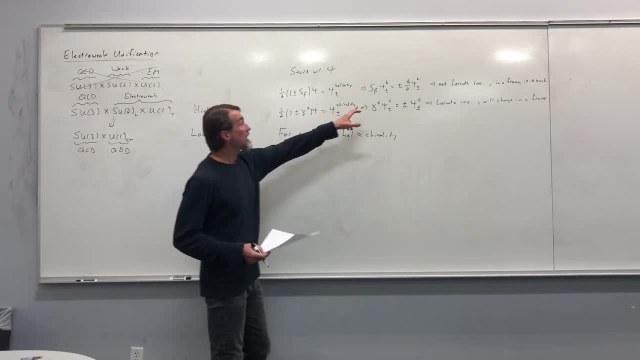 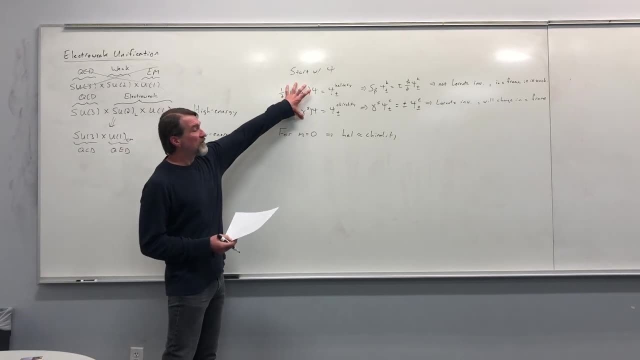 and then showed that in the massless limit it's an eigenspinner of both of these. Okay, So for the massless case you have both of these properties, which of course means that the helicity becomes Lorentz invariant. 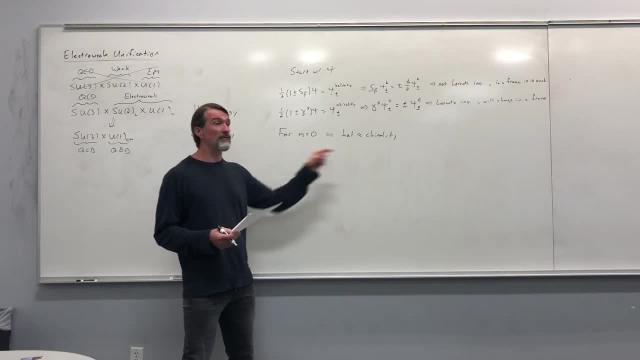 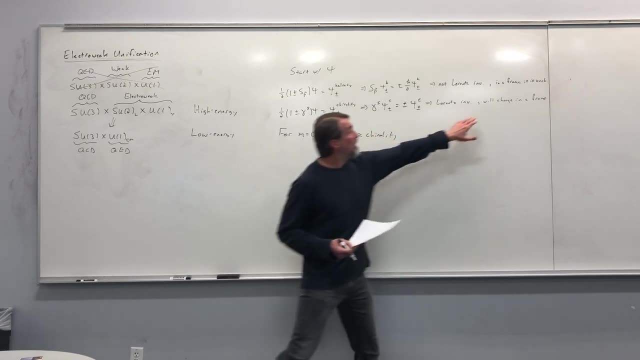 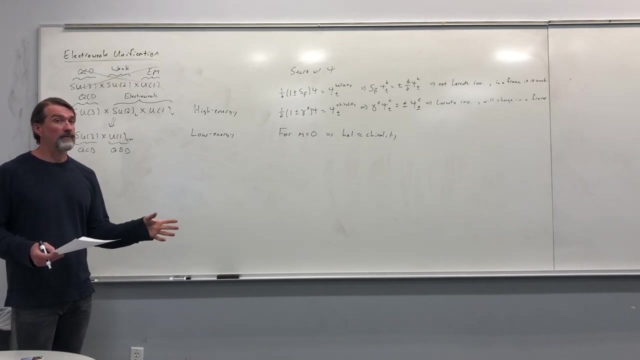 But remember we said that if you're massless, there's no way to reverse the helicity, because you can't boost past the thing. Okay, Similarly, the chirality won't change for the massless case. Does this make sense? 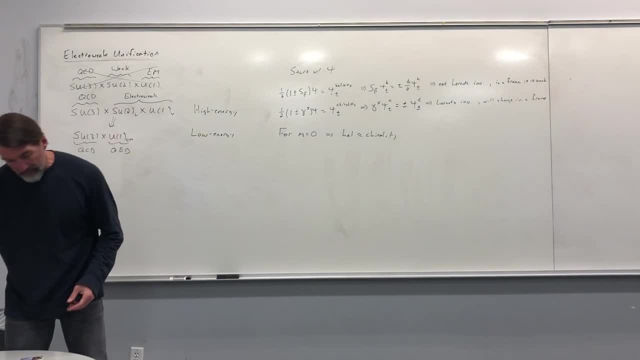 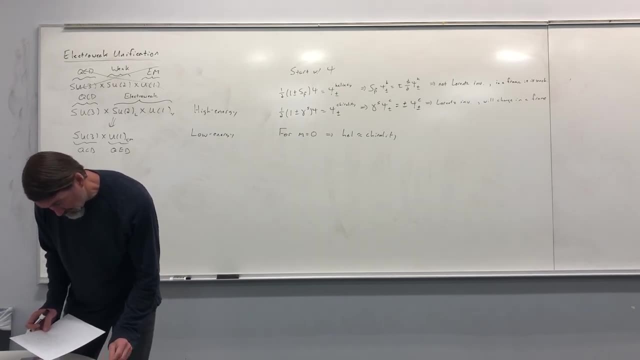 All right, Okay, So. Okay, It's about to get ugly. Fasten your seat belts, folks. A little bit ugly. It's not going to be that bad. It's going to be pretty bad, Okay. So let me get rid of this. 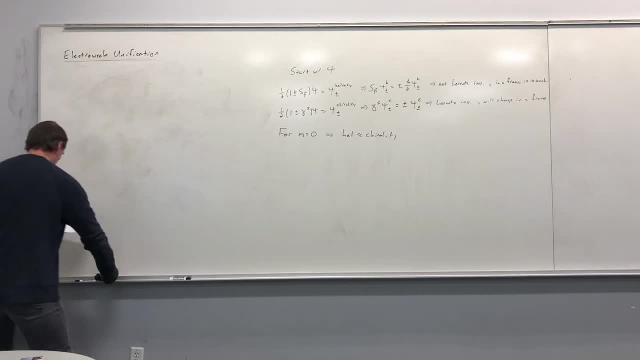 Okay, All right, So recall the Dirac Lagrangian Okay, Where we actually took this and rewrote it after our definition of chirality as: minus h bar c i psi minus dagger d mu, sigma mu psi. minus. plus i psi plus dagger d mu, sigma bar mu. 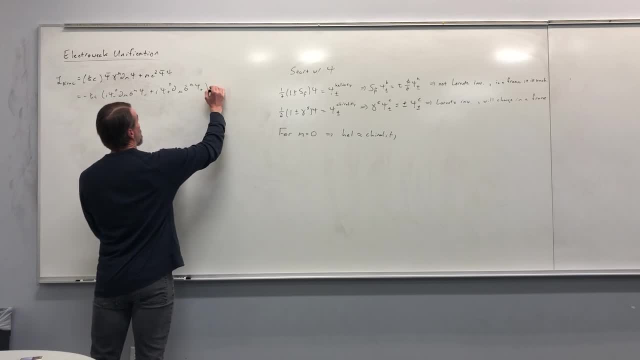 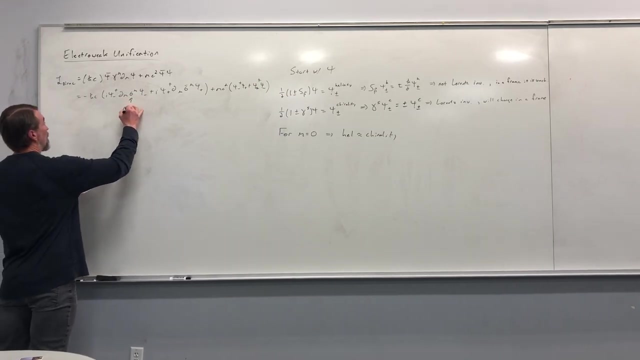 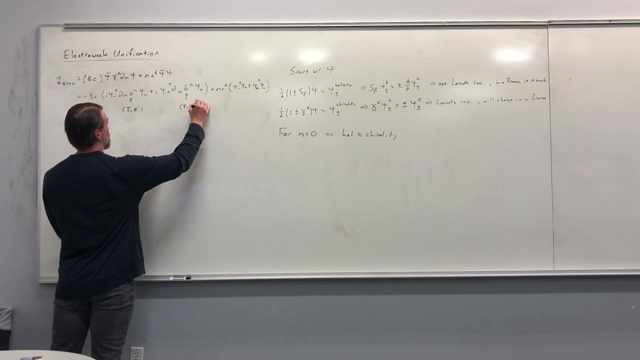 psi plus m plus mc squared Psi minus dagger psi plus plus psi plus dagger psi minus. Okay, Where the sigma mu here is i and sigma i and the sigma bar mu is i and minus sigma i. Okay, Now, this was the Dirac Lagrangian. 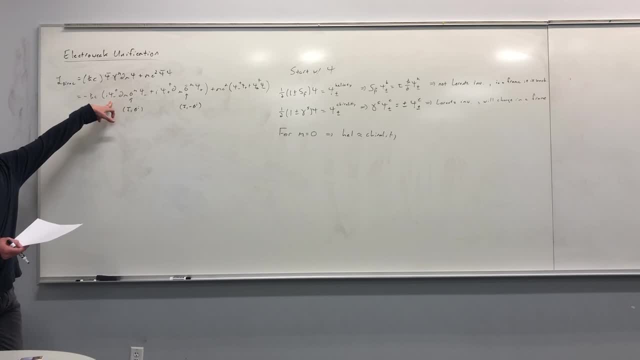 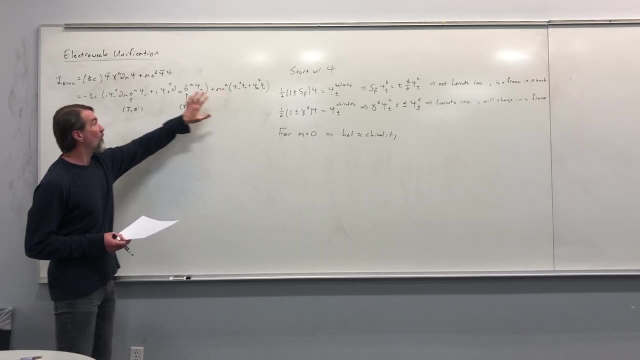 written. in terms of these two component objects. These sies are two components, These sies are four components, But these are two components And we made the observation that if the mass is zero, then we can get rid of one of the components. 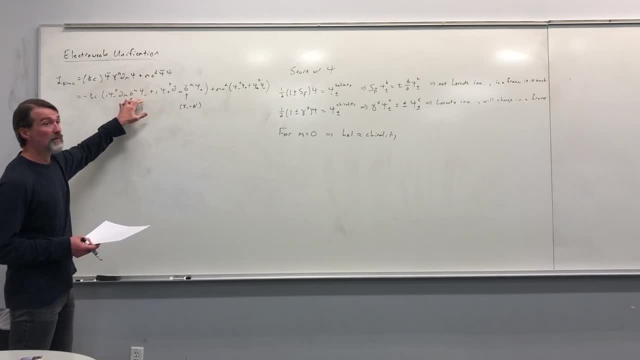 We can just do psi minus if we want, Because if the mass is zero we don't have this term. We could erase this and just be left with this. If, however, the particles are massive, then there's no way we can get rid of them. 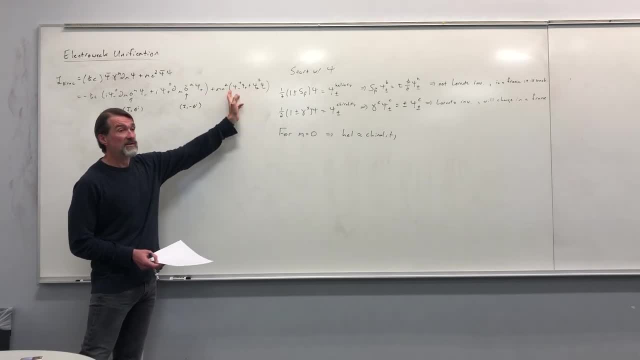 Then there's no way you can erase either psi plus or psi minus, because they're both required for the mass term. Okay, What we'd like to do is go back to four component objects. Okay, So to go back to four component objects. 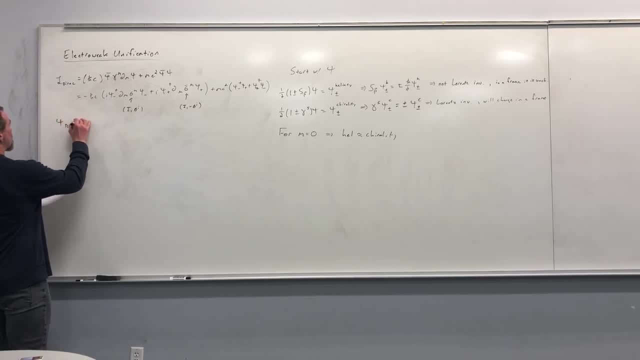 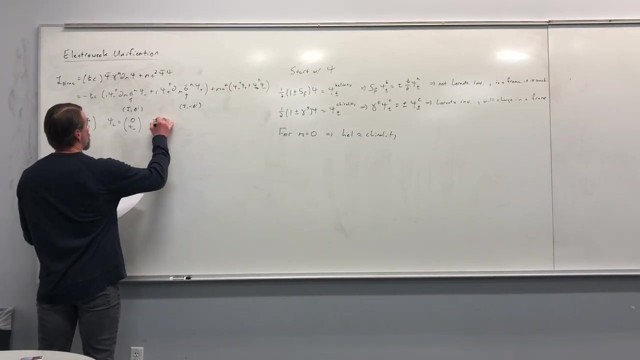 what we can do is we can define a right-handed state as basically psi plus zero and the left-handed state as zero psi minus. So each of these are two components. So this is overall four components and four components. All right. Then of course we have that psi is psi plus psi minus. 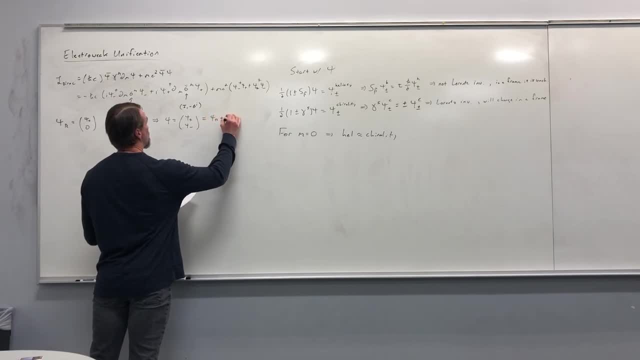 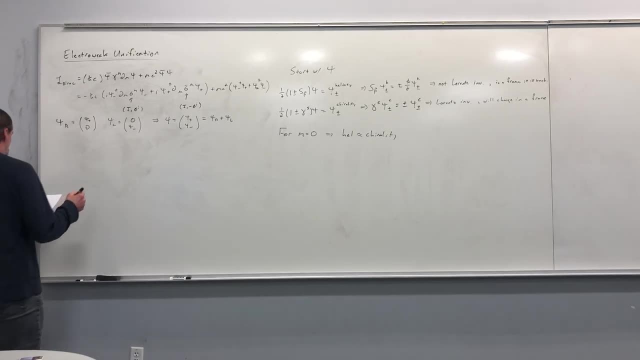 Or you can always write it as psi right plus psi left, It doesn't matter. Okay, Now let's recall: This is an arbitrary spinner. If we want to project on it, then we just use the good old one-half one plus or minus gamma five. 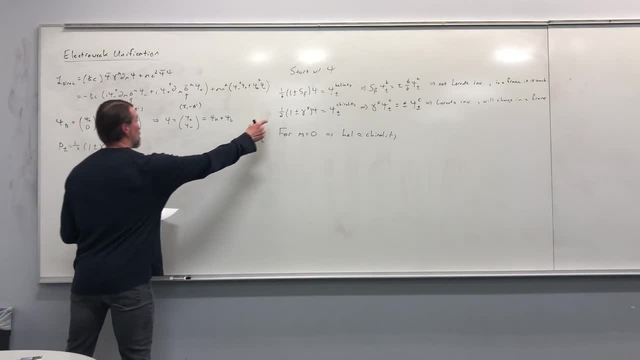 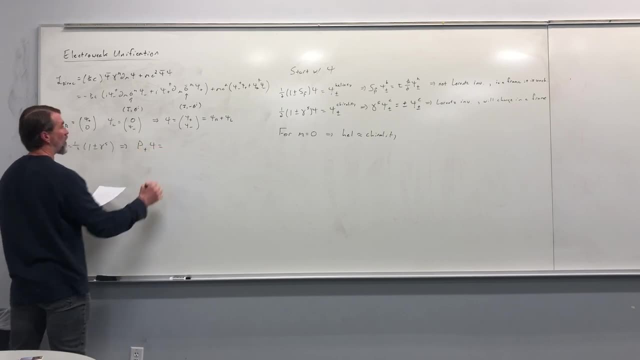 Okay, That's the chiral projection. Okay. So of course, if we take this and we hit psi with it, that's an arbitrary spinner. This is going to give us back, well, first of all the operator, If we actually plug in what the gamma pi matrix is. 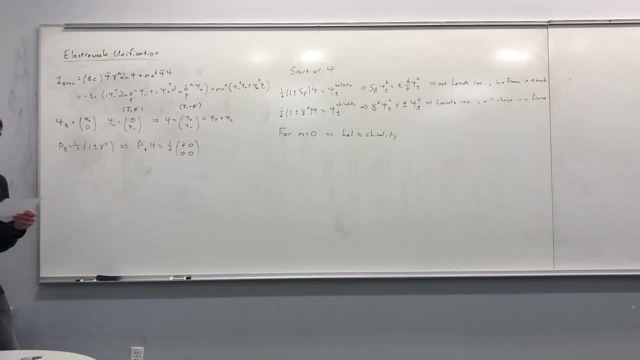 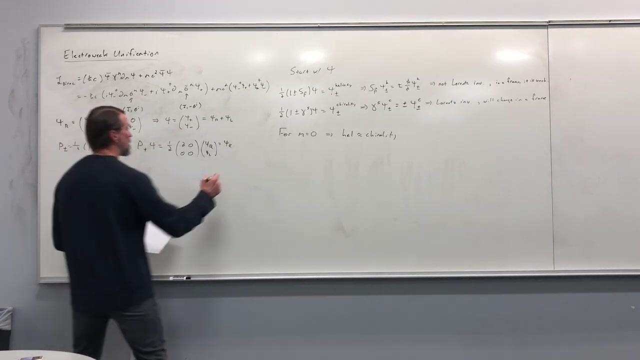 it's two zero, zero, zero. Okay. Psi right, psi left equals psi right, Okay, So the right-handed component is simply what comes out when I use the chirality projection operator on psi And, obviously, if I use the negative component. 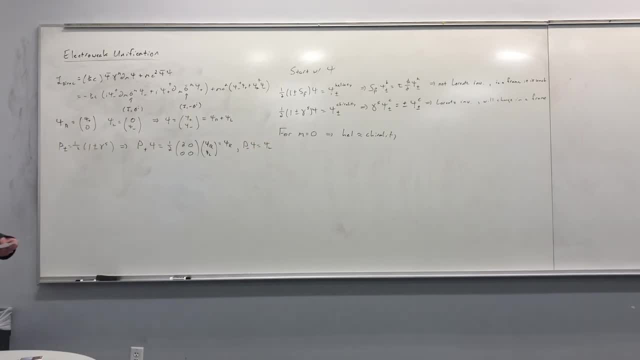 I get psi left. Okay. Now something interesting happens, though, because this is how psi gets projected. However, let's look at psi bar. Remember, psi bar is defined as I psi, dagger, gamma zero. Okay, So this is what you can think of as the dual spinner. 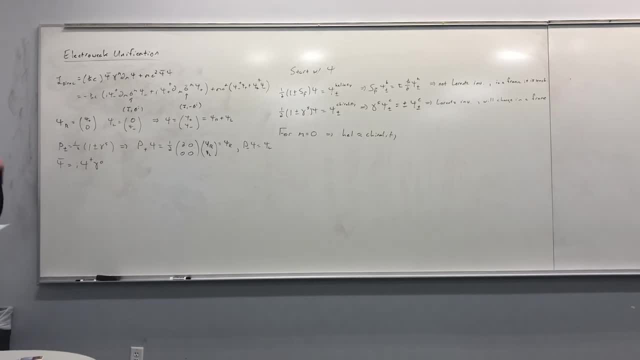 and it comes from the original spinner through this construction. All right, Now we can ask: what does the right-handed component of psi bar look like? So we'll just do this and we're going to bar this expression right here. No, sorry, we're not going to bar this. 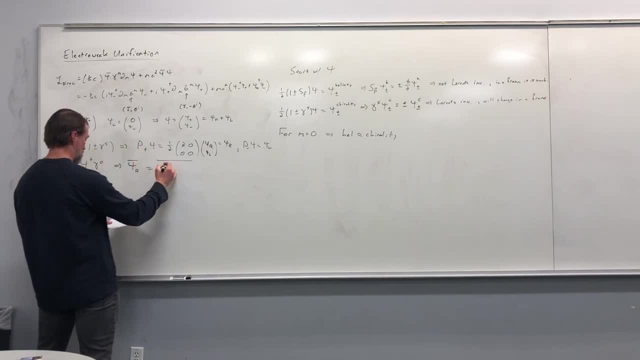 We're going to bar p plus on psi, So I can write this as one plus gamma, five over two times psi. Okay, This is psi, right? Okay, that's just the p plus operator on psi which gives me psi, right? So I mean, it's one half one plus gamma. 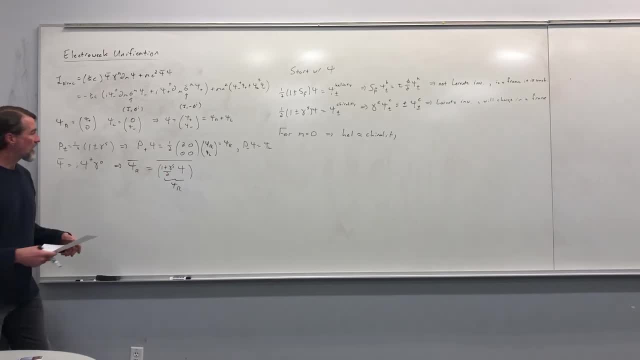 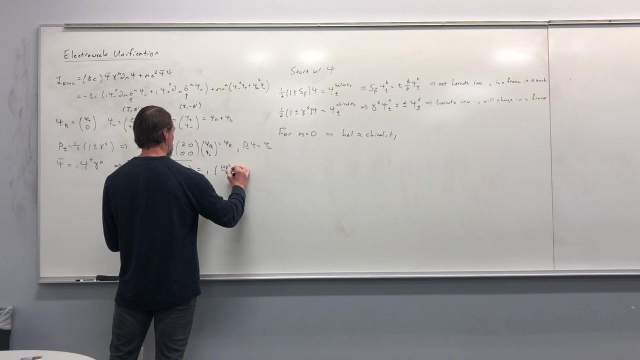 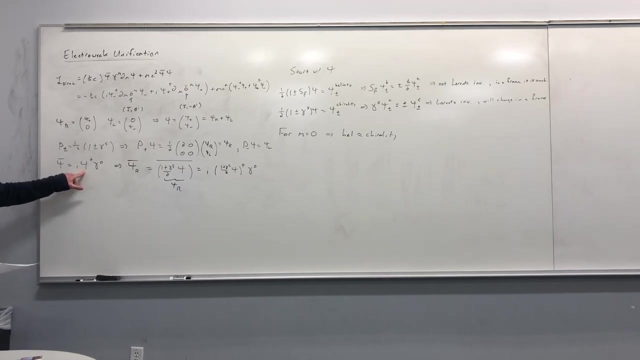 or it's one plus gamma five over two. All right, So now we can bar this according to this prescription. Okay, So this is going to be I, one plus gamma five over two psi dagger zero. Okay, Again, I just take everything that's in my psi expression. 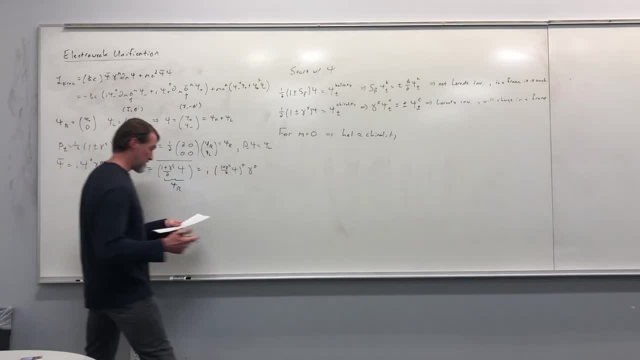 and I just dagger it and then I just tack on an I and a gamma zero. Okay, And now of course I can do the usual thing if I'm daggering a combination of things, and I reverse it if I want to do the individual daggers. 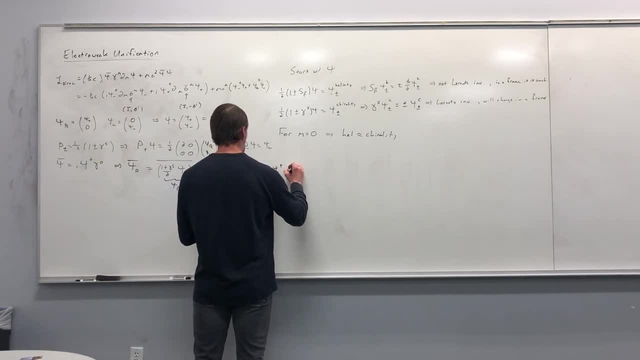 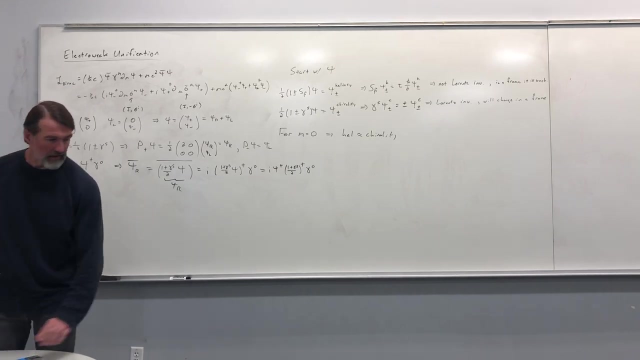 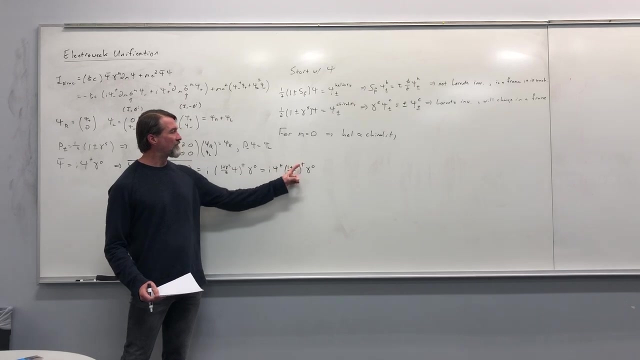 So this is going to be: I psi dagger one plus gamma five over two dagger. gamma zero, Davis, Yeah, Can you tell me what one half dagger is? Well, actually there's two questions. One is what is one half dagger, and the other one is what is gamma five over two dagger? 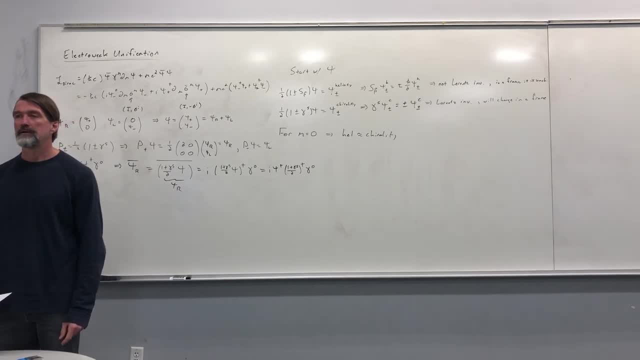 I'll do one if you do the other. Which one do you want to do? I like one half, Really. Yeah, One half is way harder. It's so complicated. You could try it. Yeah, it's one half. I'm totally kidding you. 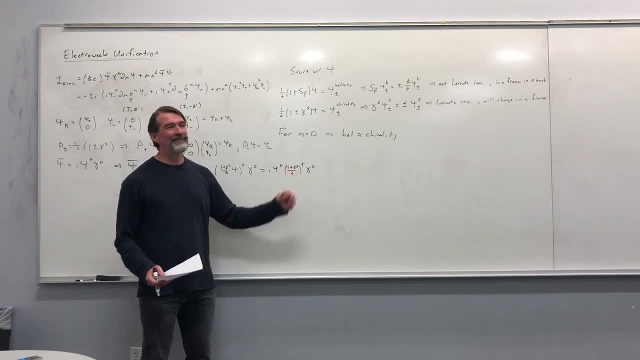 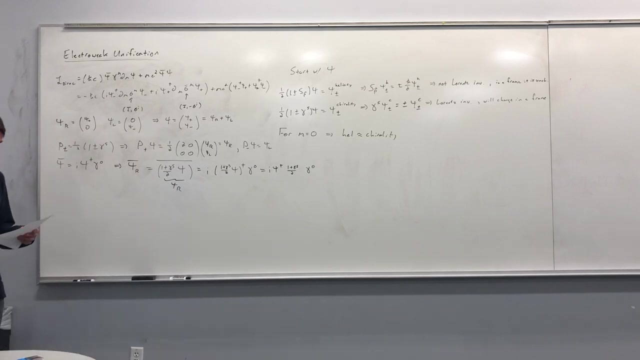 One half is daggered as one half Gamma five over two. daggered is gamma five over two. Gamma five dagger is gamma five. Okay, So we can actually just erase this. It's a nice property of gamma five, Okay. And now, oh wait, look, hold on. 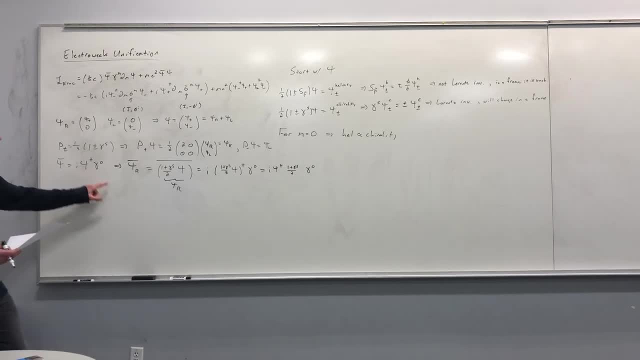 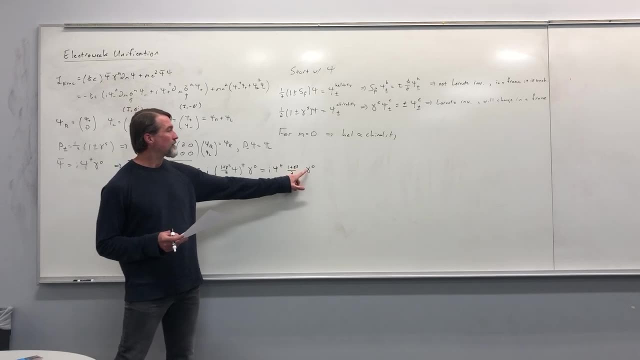 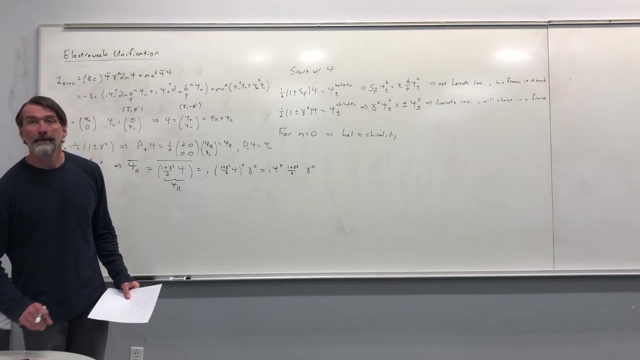 Sss, sss, sss. I side dagger gamma zero, I side dagger one plus gamma five over two. Okay, Maybe I'll just move this to the other side, But when I move gamma zero past one half, what happens, Henry? 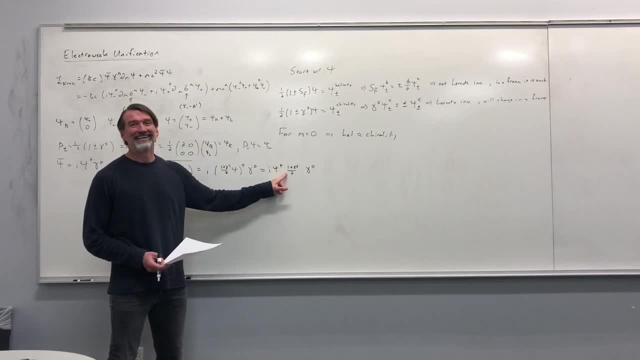 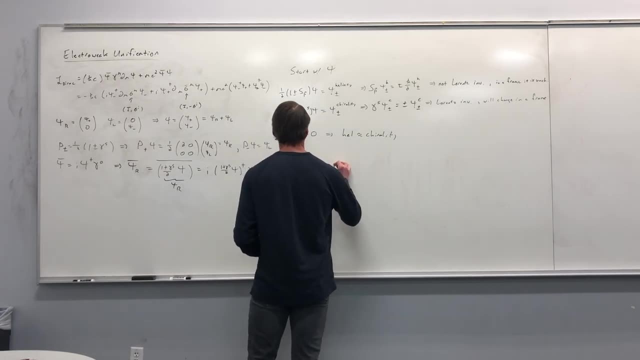 If I'm moving gamma zero past the number one half, Oh, none, None. What if I move it past gamma five, Then you get a negative sign, Then you get a negative, Exactly Okay. Well, this means side bar one minus gamma five over two. 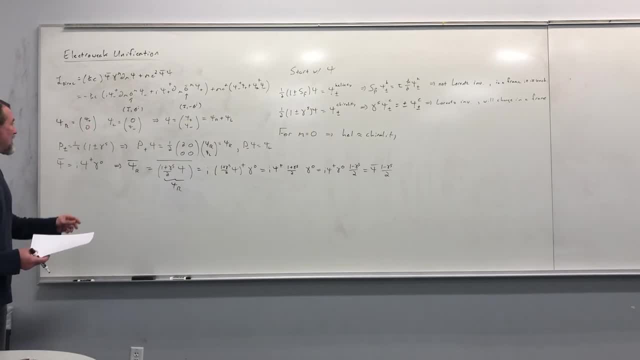 So the point of this is to get the right-handed component of the dual spinner. Instead of using one plus gamma five, we use one minus gamma five on it, Okay, Okay. So with that in mind, we can go ahead and write the direct, the equivalent of this, and this using these left and right components. 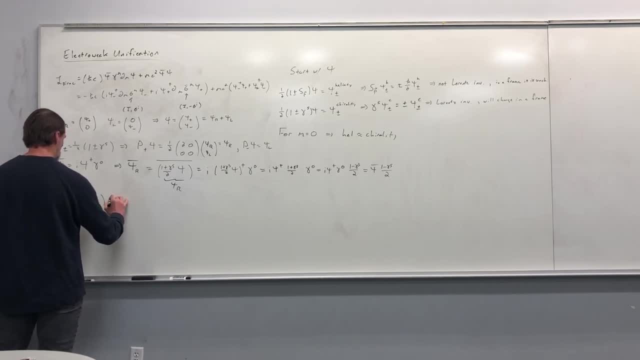 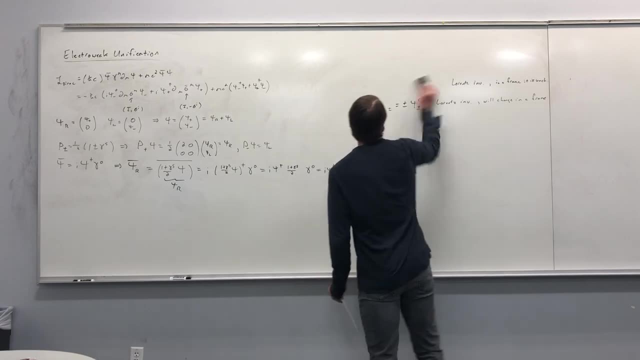 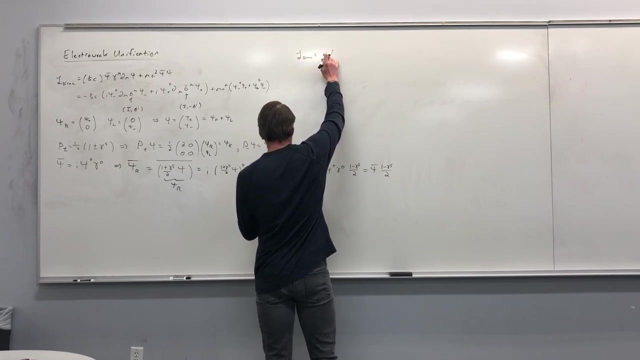 So here we go. H bar C. Actually, I'm going to write this up there. I'm going to erase this because we're not going to need it anymore And this is about to be the work done, All right. H bar C. 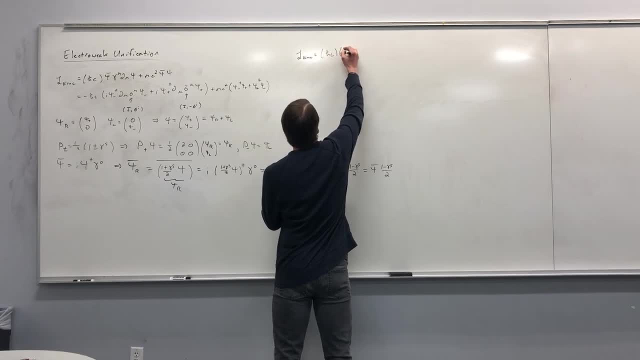 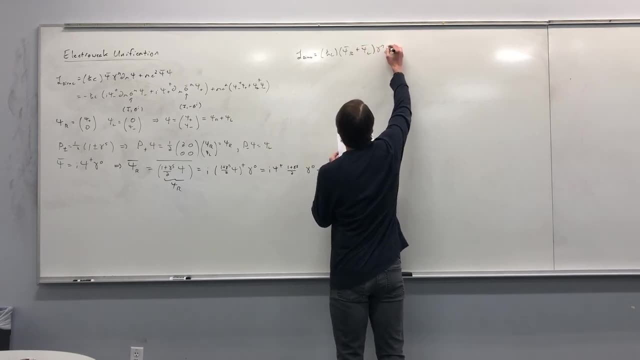 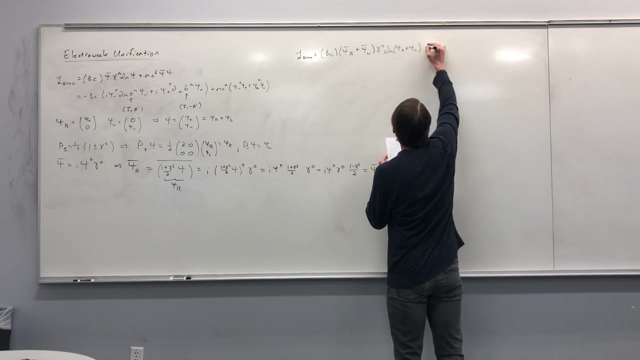 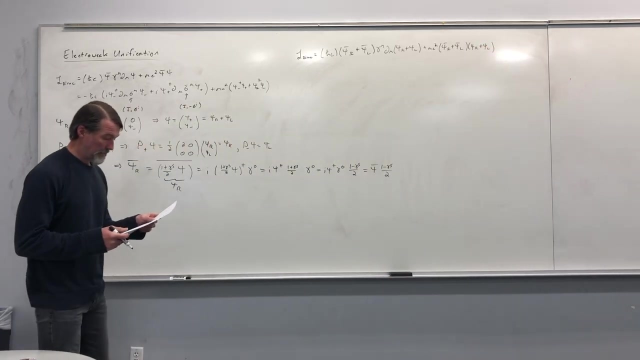 All right. H bar C. Psi bar right plus psi left. Gamma mu d mu: Psi right plus psi left Plus MC squared: Psi bar right plus psi bar left. Psi right plus psi left. No requested ratio, Okay, Okay. 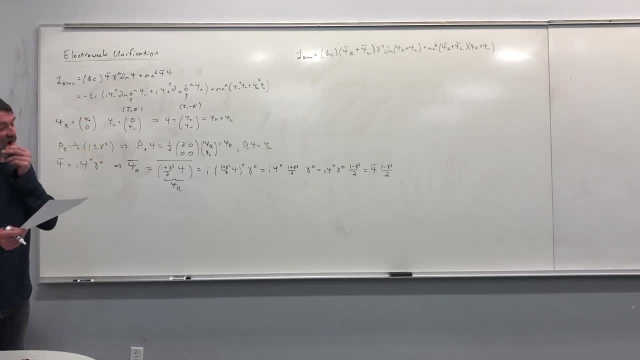 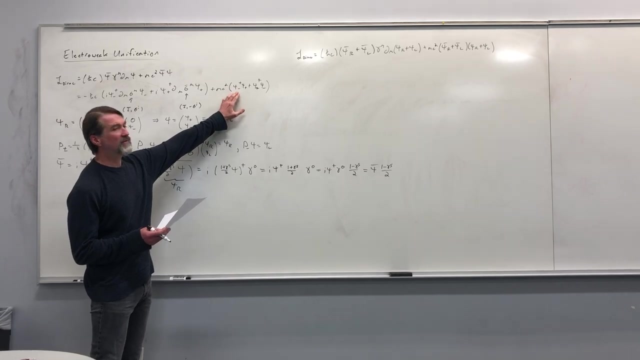 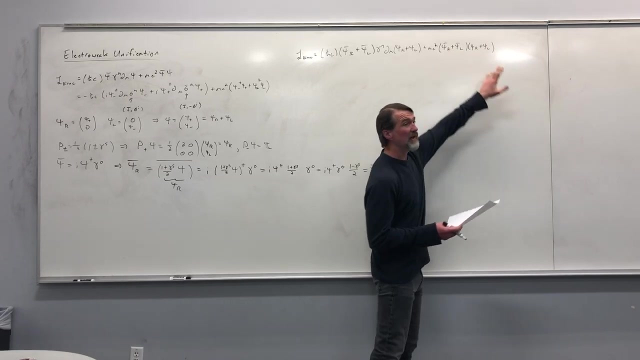 Let's write this down, Okay. Okay, Really, it doesn't really share this property, right? This property. you only had plus and minus combinations. I can have right and left and left and right, but I can also have right and right and left and left. 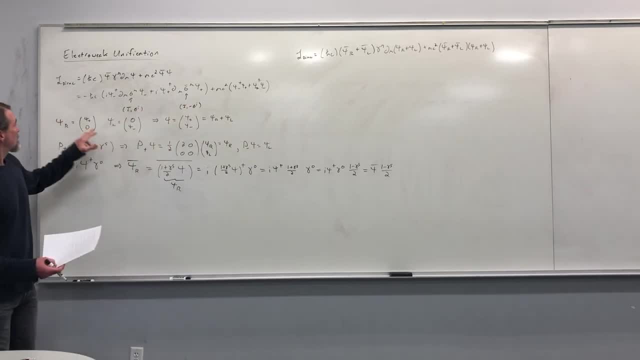 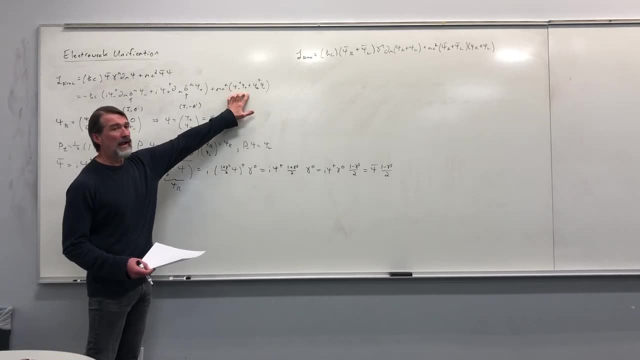 So it doesn't. I mean, even though the right component is just psi plus zero and the left is zero psi minus, it seems that I've taken this where I'm saying, like if the mass is zero, then you can take, you know, 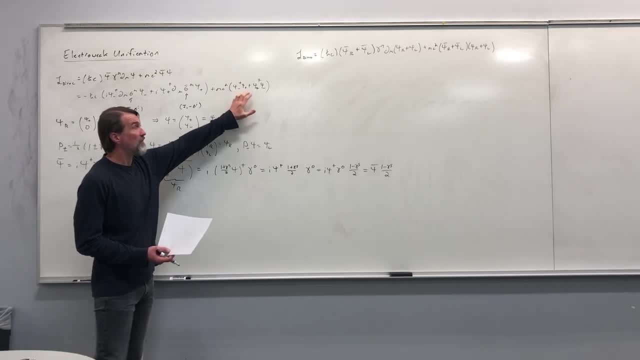 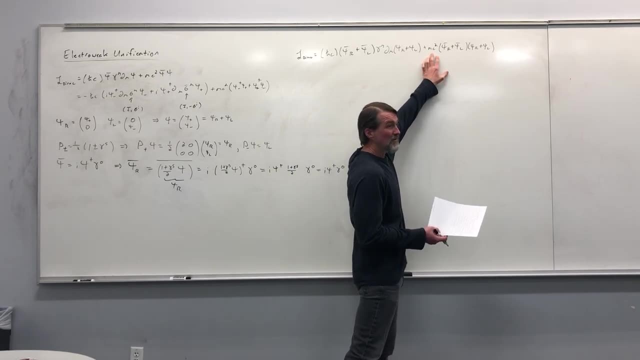 just the plus or just the minus, But if the mass is not zero, you require both. However, you know like it seems like I could take the left-handed parts to zero and still have a mass term right? Well, it turns out this contains: 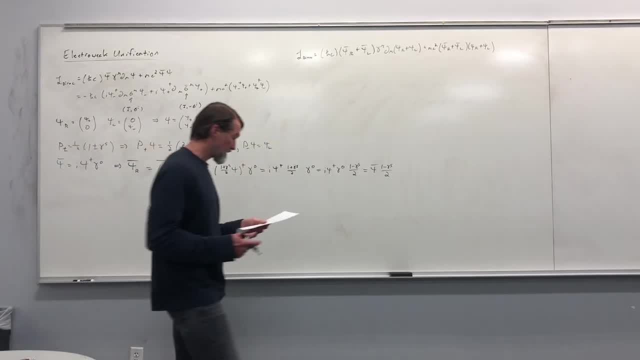 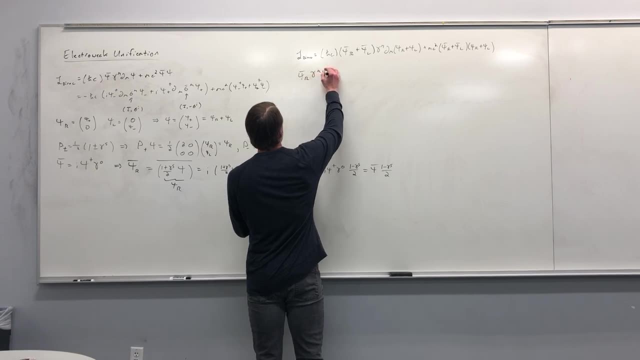 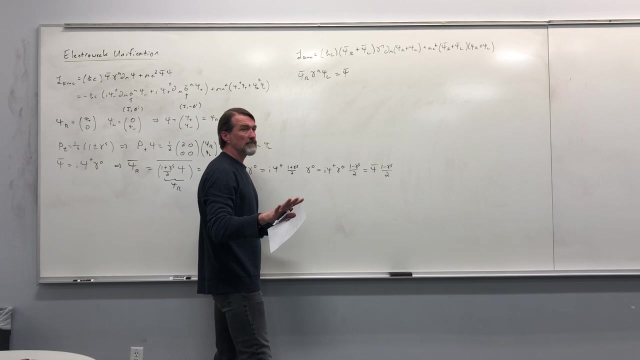 the same information as this. Let's see, First of all, if I do psi bar right, gamma mu, psi left, okay, then this is, and I'm basically just looking at the spin, This is the spin space structure, D mu, that's the space-time operation. 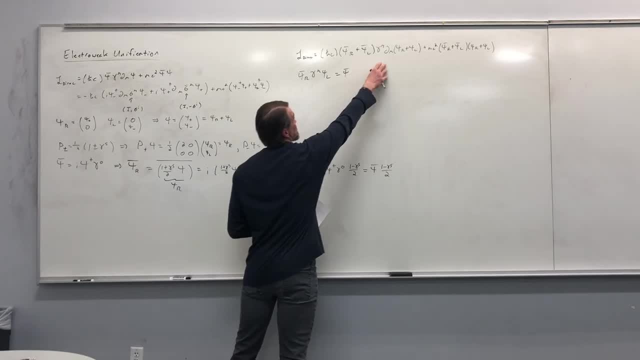 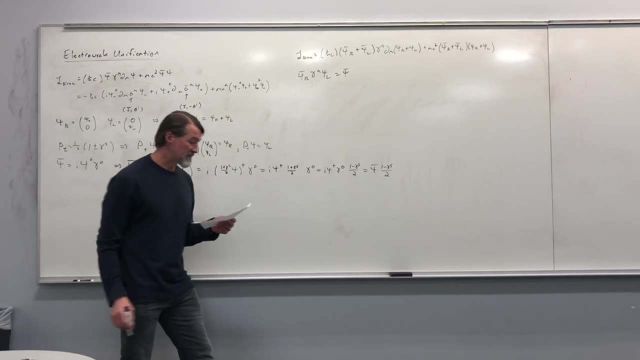 It's just the derivative with respect to where you are in space-time. okay, So it's got a trivial spin structure. This is obviously a matrix in spin space, and then these are spinners in spin space. So I want to look at the spin space behavior. 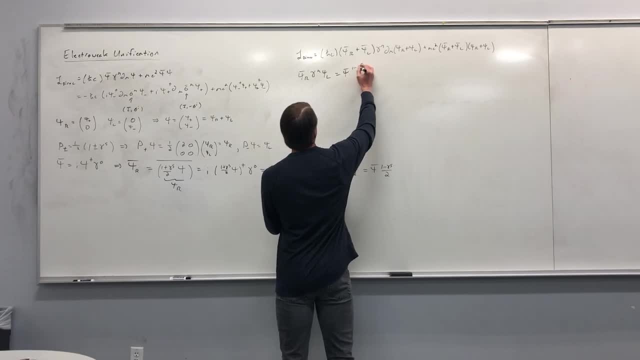 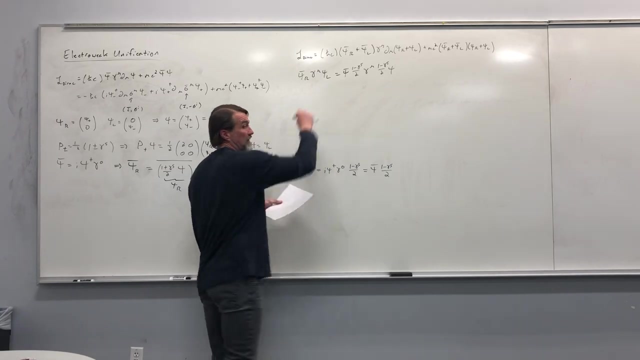 So this is going to be psi bar one minus gamma five over two. That's just the right-handed version of psi. bar Times gamma mu one minus gamma five over two psi. That's the left-handed component of psi. okay. 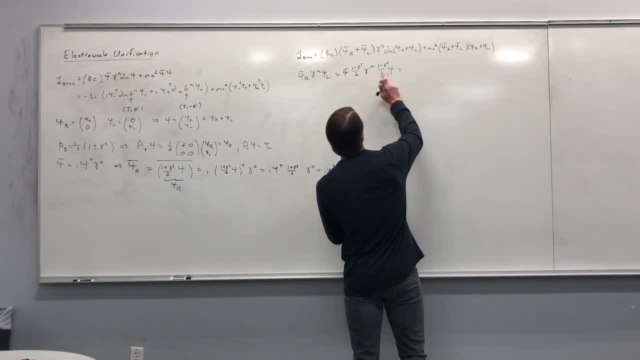 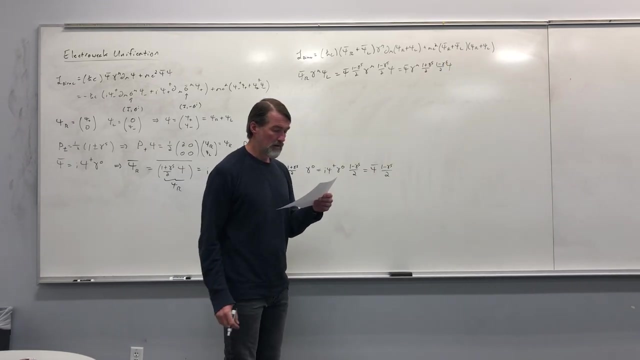 And then I can move this past the gamma mu to combine it with this and that's going to give me psi bar gamma mu. one plus gamma five over two, one minus gamma five over two of psi. Oh wait, This is one. 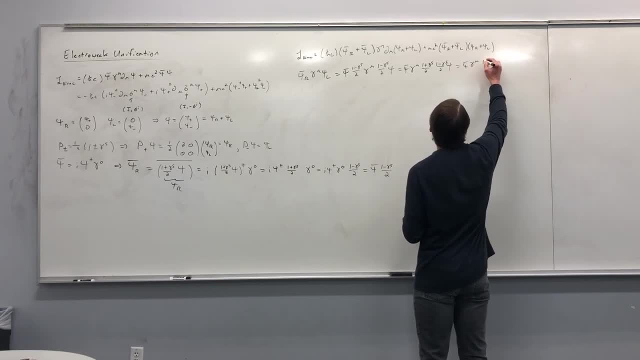 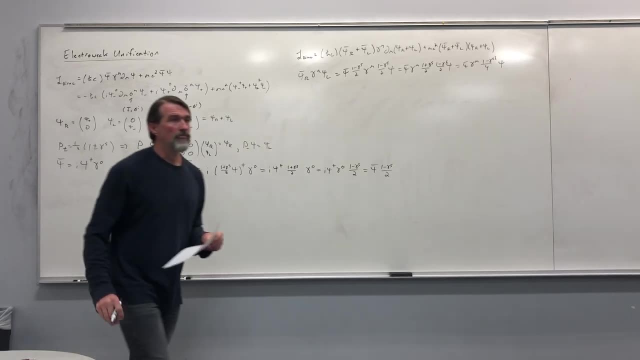 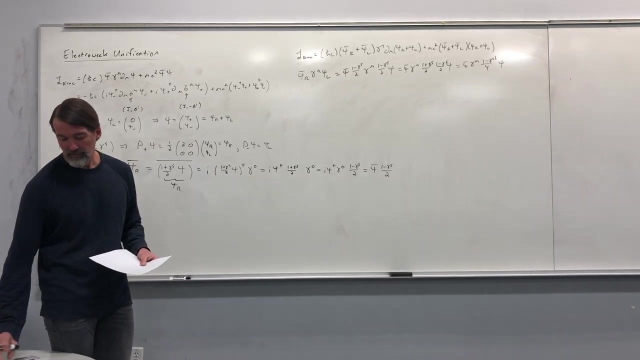 This is psi bar gamma mu, one minus gamma five squared over four times psi, It's just one plus times one minus. It's really simple, Joey, can you tell me what that is? What's the value of that? I'll give you a hint. 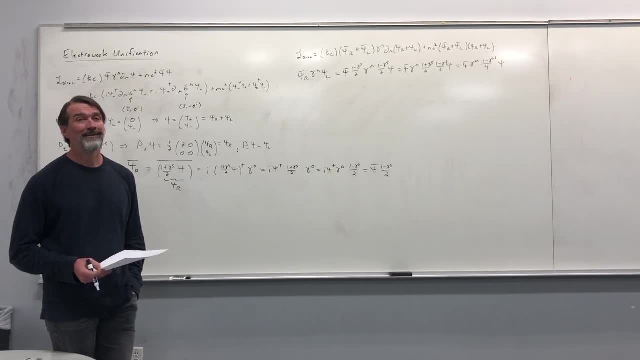 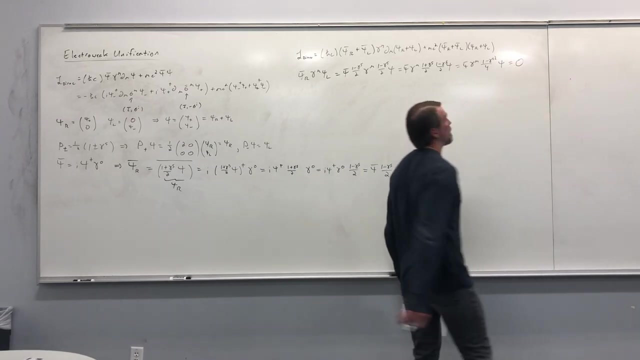 It's the value that's contained in the one minus gamma five squared. Do you remember what gamma five squared is? Gamma five, Oh sorry, Is it? i Can't remember, It's one, Okay, Okay, So it turns out if you do one minus gamma five squared. 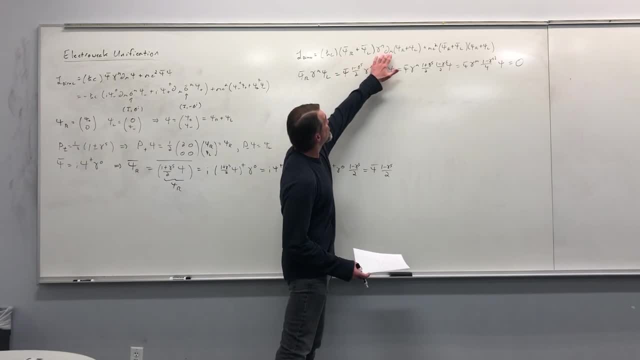 you're going to get the following. You're going to get the following: You're going to get the following: that in expanding this kinetic term, mixing psi right with psi left is always going to give me 0, and similarly, psi bar left with psi right, so that means the. 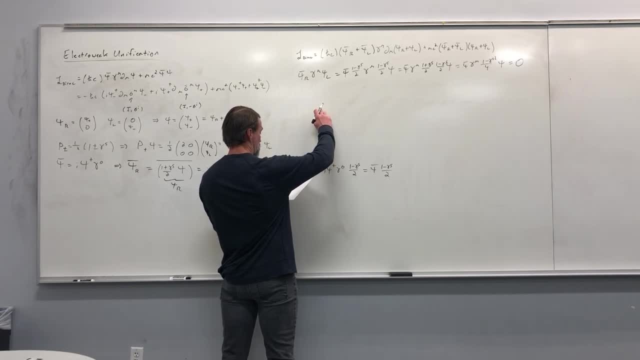 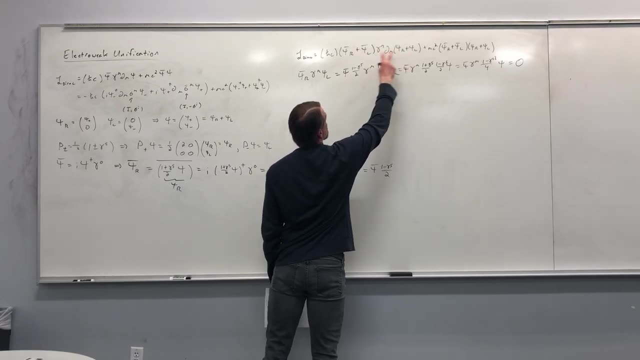 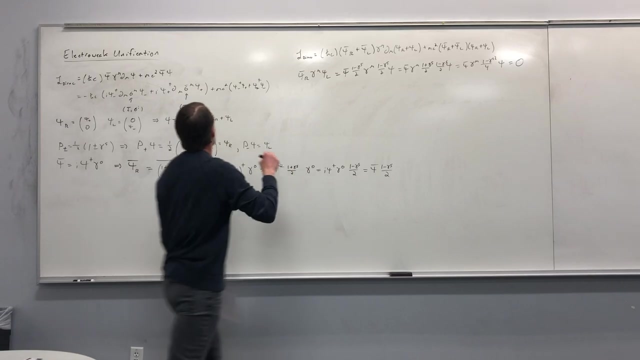 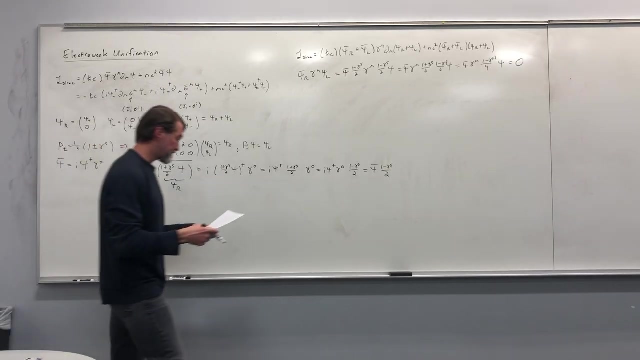 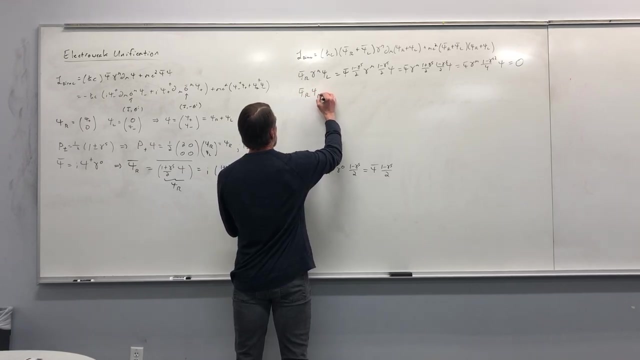 kinetic term. well, basically, in expanding this product, I'm only going to have psi of our side, our side, our terms, and sidebar left, side left terms similar to here, where I have minus and minus, plus, plus and the next terms of the derivative. okay, now we can consider side right, side bar right, side, side right. so this would be a term from. 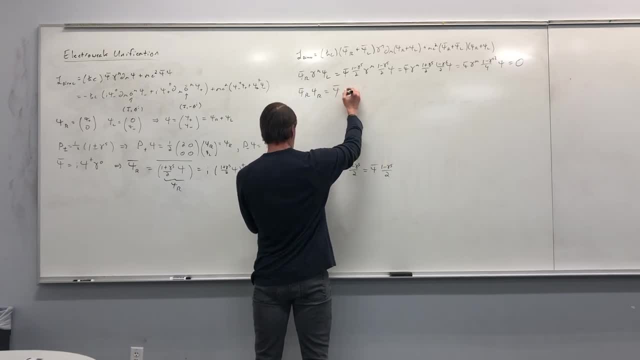 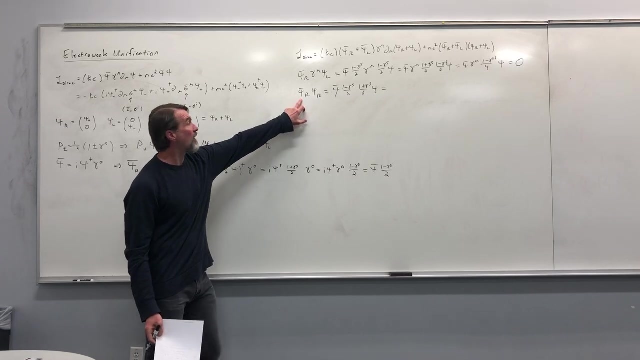 here- and this is once again going to be sidebar- one minus gamma 5 over 2 right and minus 1 minus gamma 5 over 2. one minus or one plus gamma five over two psi, Remember if I want the right component of psi bar. 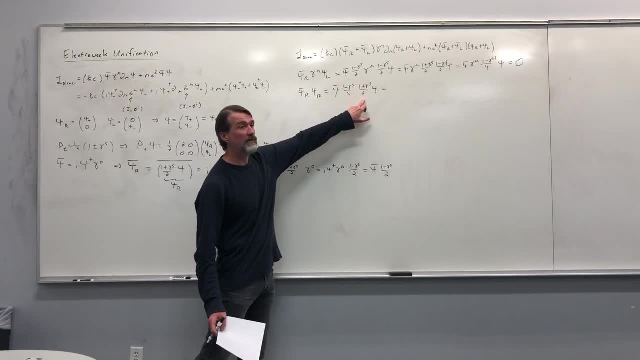 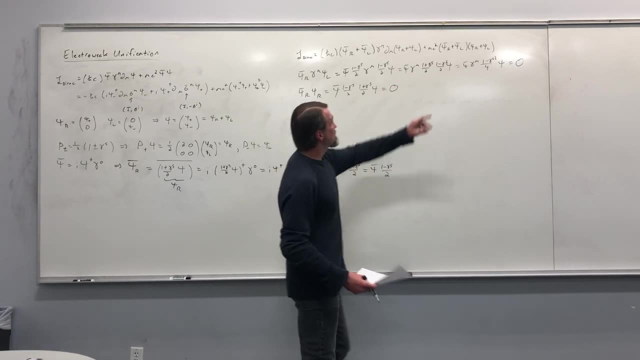 I do one minus gamma five over two. If I want the right component of psi, I do one plus gamma five over two. But what's this? equal to Zero, Zero, same story. So that means that in the mass terms, if I'm considering the psi bar right combined with psi r, 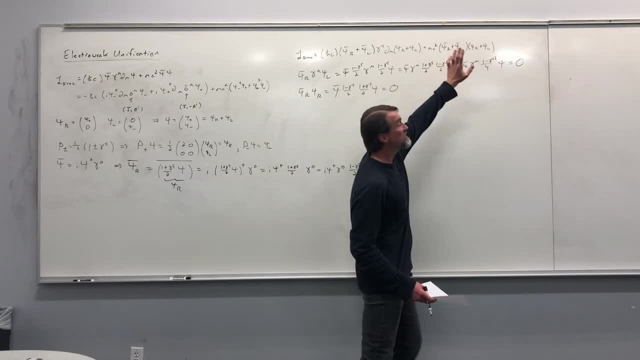 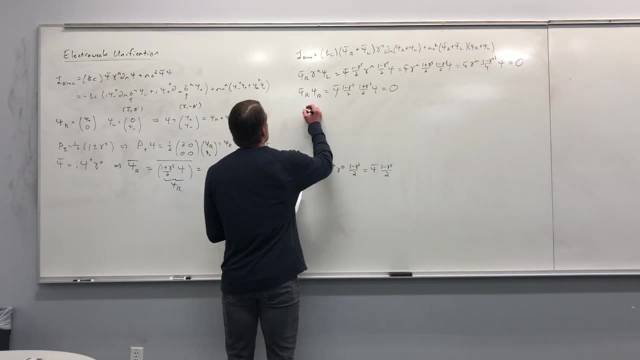 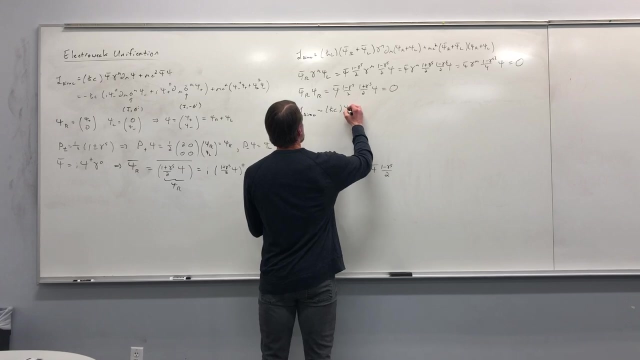 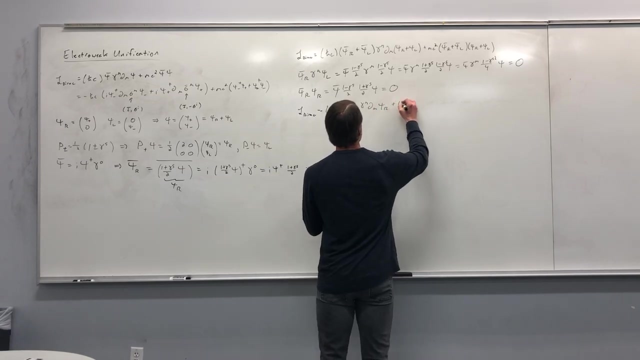 that's automatically zero. So in the mass terms, the only ones that are not zero are psi bar right with psi left and psi bar left with psi r. OK, So at the end of the day, our Dirac Lagrangian simplifies to h bar c, psi bar r, gamma, mu d, mu psi r plus h bar. 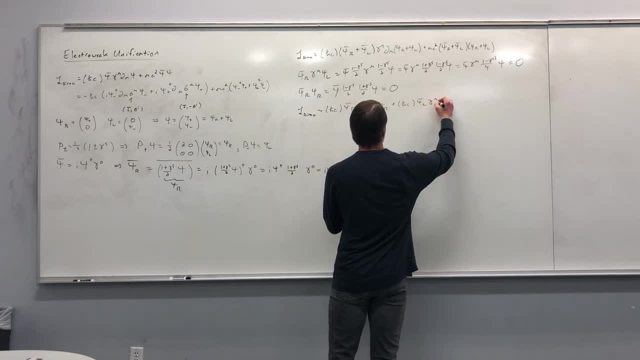 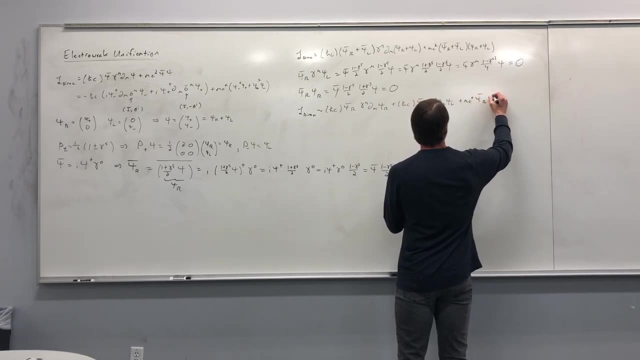 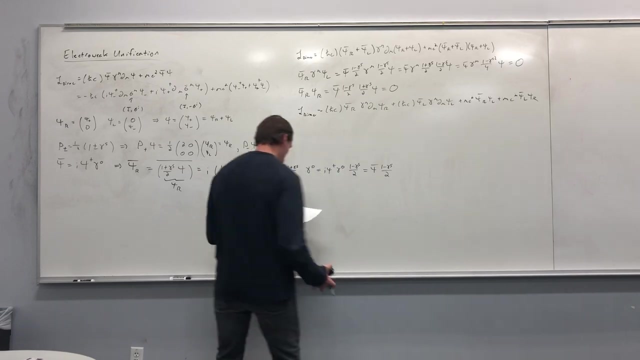 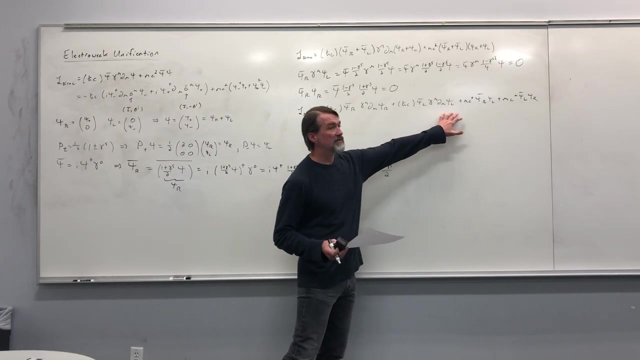 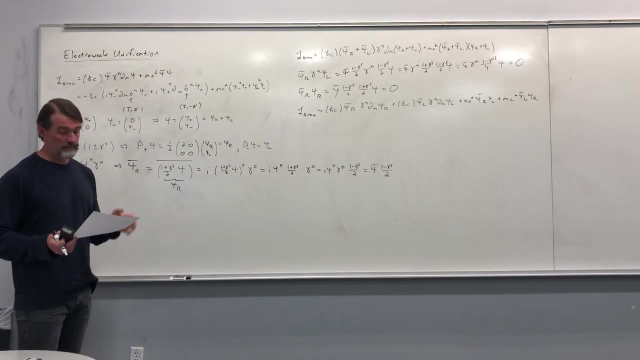 c, psi bar left, gamma, mu d, mu, psi r, Psi left plus mc squared psi, bar right, psi left plus mc squared psi, bar left, psi right. OK, Where everything in this expression is composed of four component spinners, versus this two component story, All right. 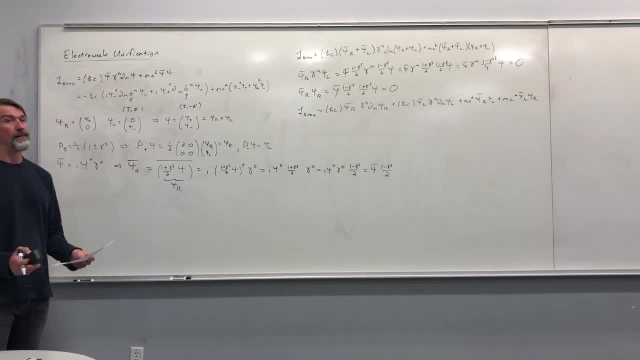 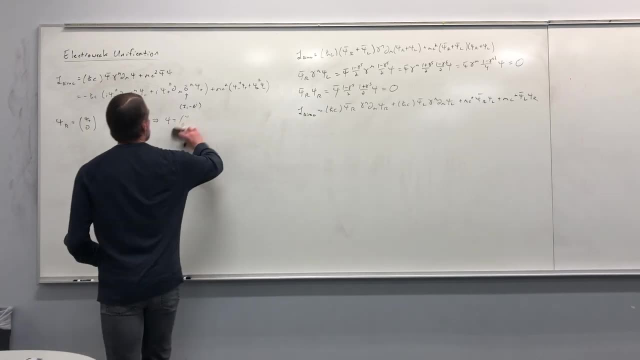 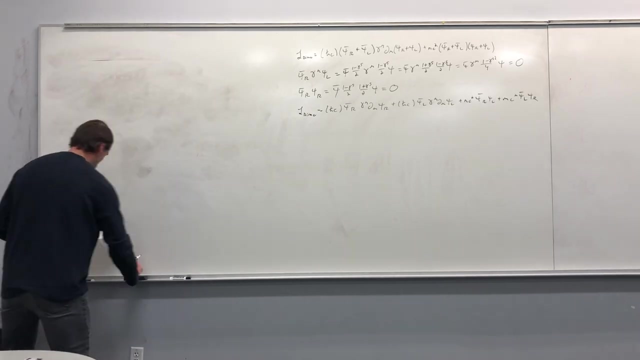 Any questions? All right, Now it's time to try and address the symmetries. OK, Remember our symmetry group is su two. OK, That's our symmetry group. left: cross U1 hypercharge. Okay, First of all, let's start with the SU2 left. 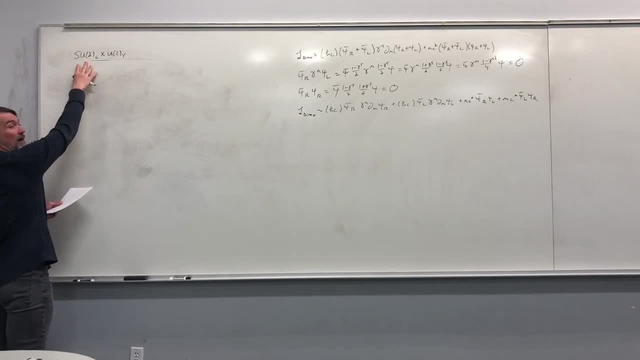 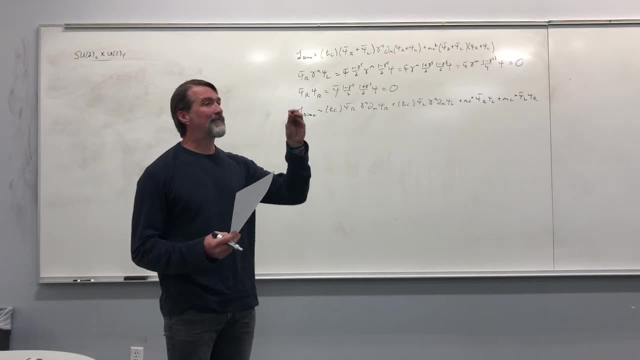 For SU2 left. these are obviously complex 2x2 matrices, So, as such, if they're going to act on something, they have to act on something that has two components, And it's exactly the same story we encounter with the strong interactions. 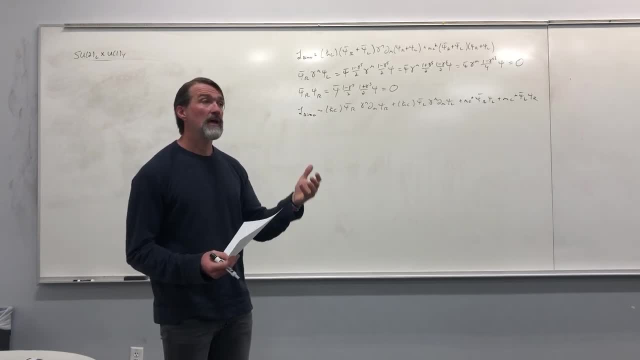 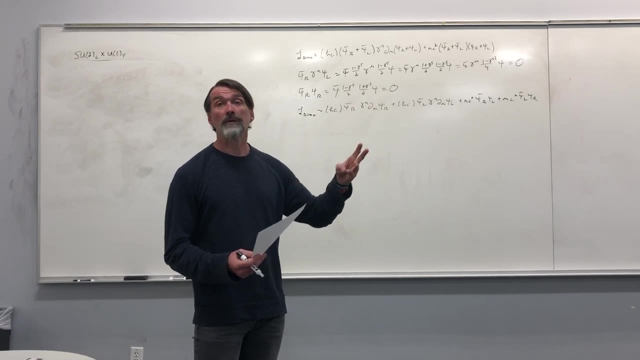 The SU3s were 3x3 complex matrices so we had to have it act on things with three components And we introduced red, blue and green, the three colors. So we said every single quark, whether it's up down, strange top, bottom. 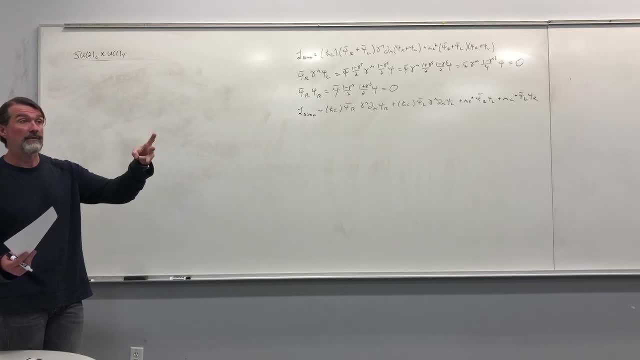 it doesn't matter. every single quark comes in these three flavors. So I can say the red up quark, green down quark and blue down quark, All three ups, sorry. At any rate, This has to act on two component things. 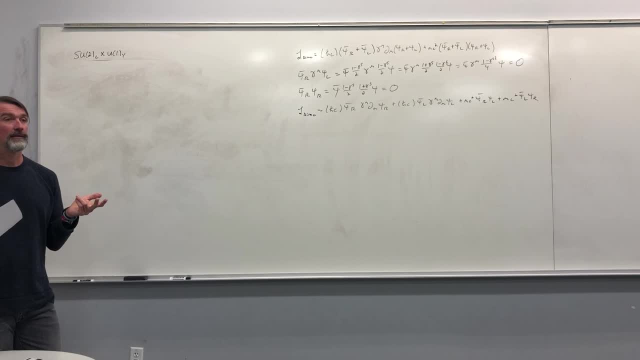 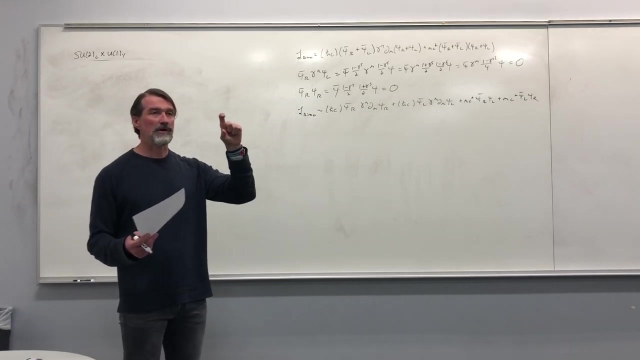 So what are we going to introduce in this story? What kind of doublets? What are they Exactly? Remember, I've been organizing all of the matter in the standard model, in these little pairs Up down, quark, charm, strange quark. top, bottom, quark. 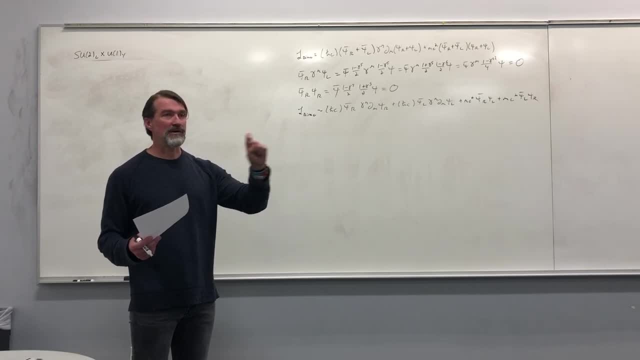 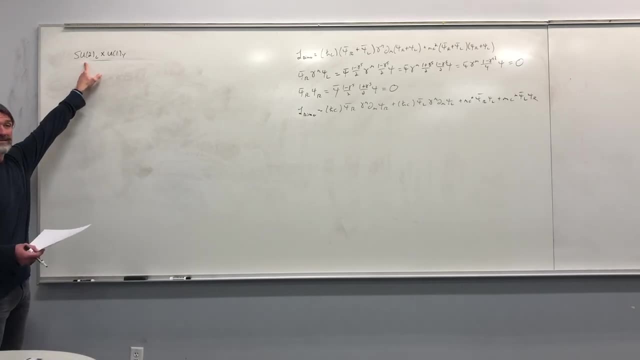 electron, electron neutrino, Muon, muon neutrino, tauon, tauon, neutrino. Those are two component objects. Those are exactly what these 2x2 matrices enact or act on. Okay, So we can say that we have left-handed doublets. 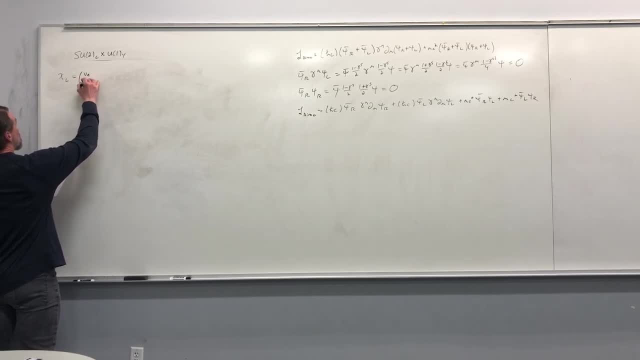 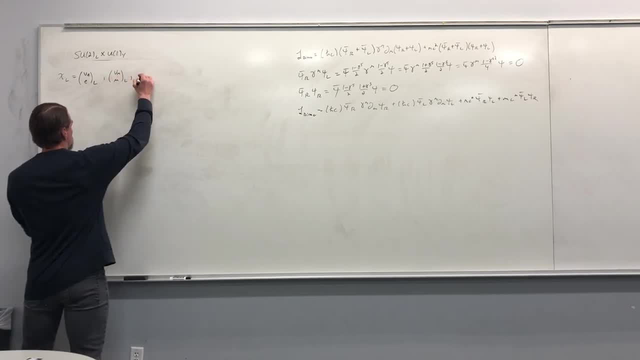 The muon, neutrino and the muon- the left-handed part of that. The tauon, neutrino and the tauon- the left-handed part of that. The up-and-down quarks, the left-handed part of that. The charmed and strange, the left-handed part of that. 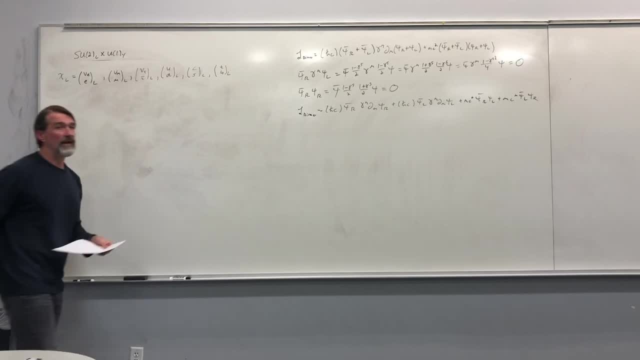 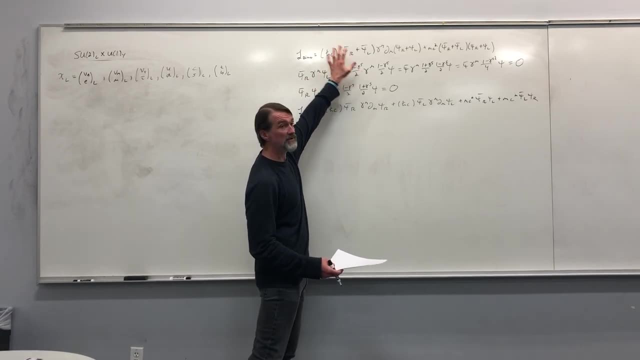 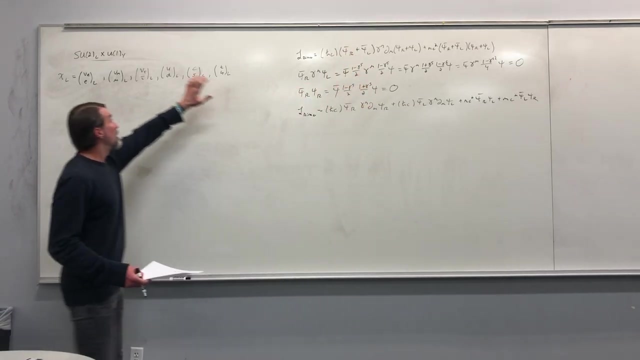 And the top and bottom, the left-handed part of that, Only the left-handed parts. Notice: everything is broken up in this Dirac Lagrangian. So this is the Lagrangian good for any matter, but it's just written in terms of left and rights. 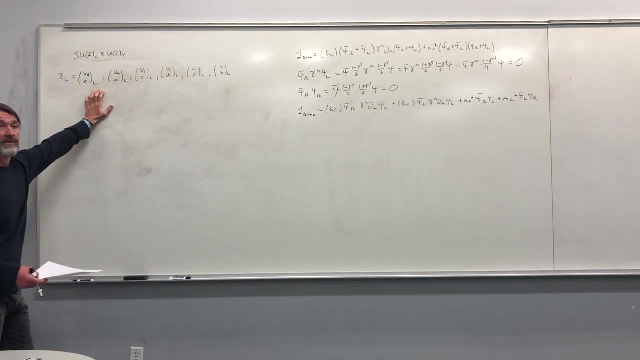 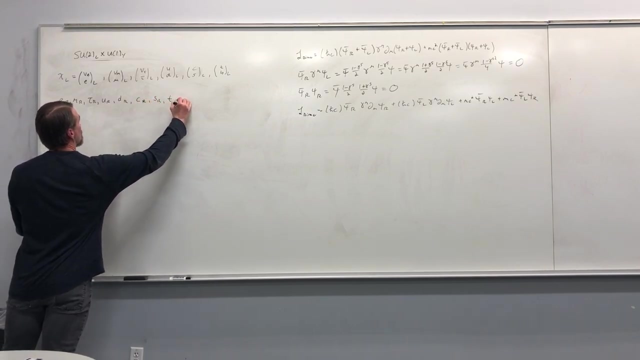 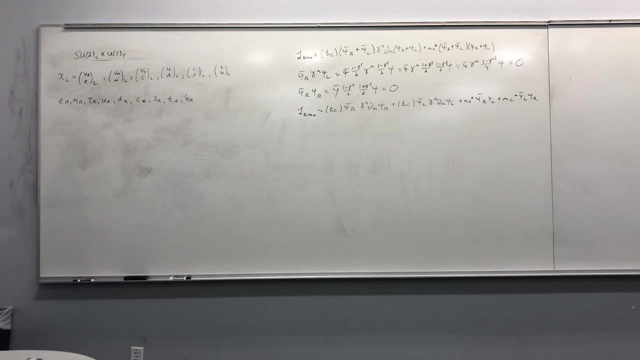 We're only going to use the left-handed parts with this doublet structure. Okay, For the right-handed side, we get singlets. Okay, Now wait a minute. am I missing something? I think we could hope so, Yeah. 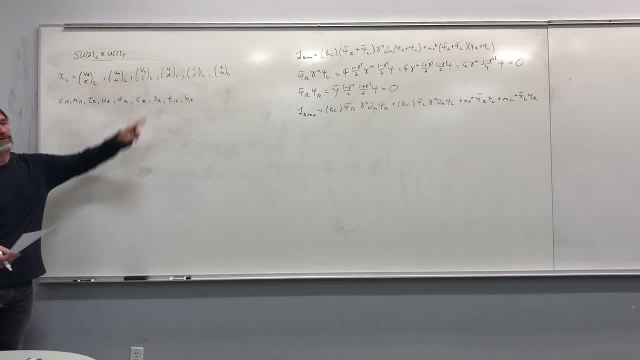 I seem to be missing the right-handed neutrino components In this class, which we're not going to go into this research. but in the modern take on things you could actually have right-handed neutrinos, but that's owing to the fact that neutrinos might actually have a mass. 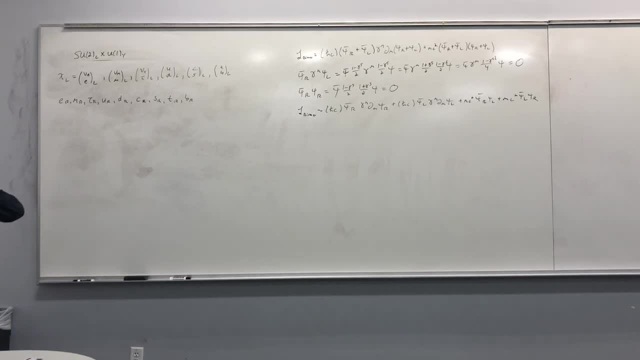 In this story that we're going to tell in this class we're just going to go with massless neutrinos, Okay, And if you have any questions about masses, that's who you can talk to. Okay, But what's important is: 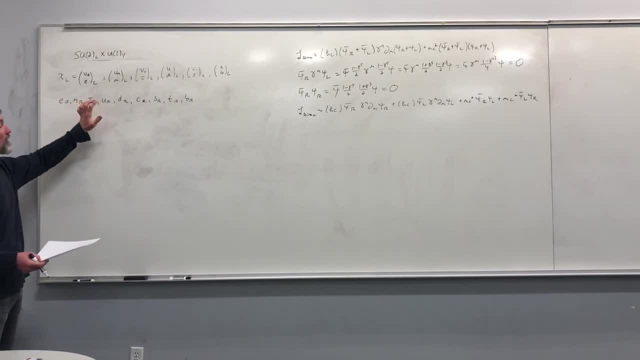 we're going to go massless neutrinos. therefore, they don't have right-handed components, They only have left-handed components. Okay, Remember what I said: If you're massive, then you cannot have just left or right, You have to have both. 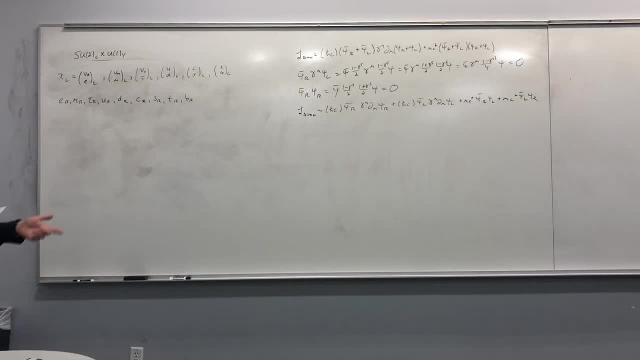 But if you're massless, you can have just left or just right. Well, it turns out in the massless story we only have left-handed neutrinos. We do not have right-handed neutrinos. Yes, Sorry, but when we are talking about models, 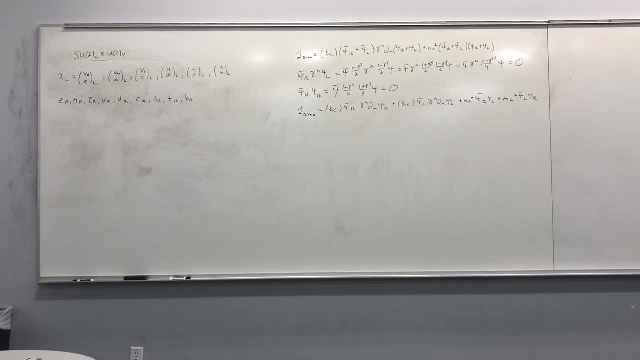 we talk about matter, but if we talk about antimatter, So antimatter largely follows the same story. But we work also with, for example, left, left or right, right, right, right, Yes With right Wait. 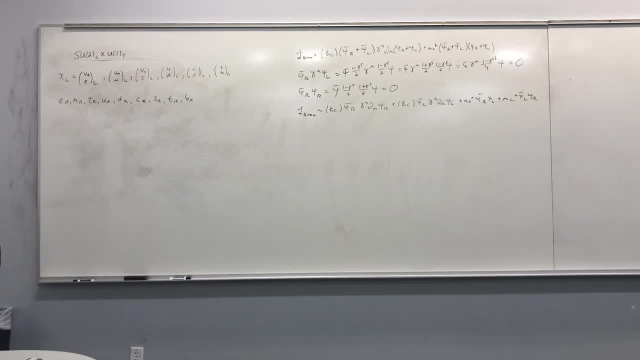 Ask the question again. It's like you are taking the duplex of left of all the particles, but if you develop, Okay, I will develop the same, but for anti-particles. So you should take a duplex of left, right, right, right, or? 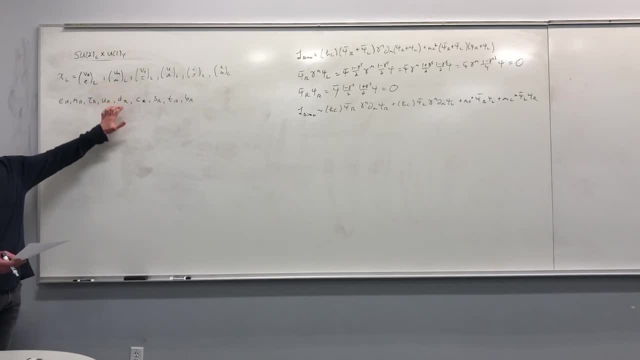 So are you saying that we would use left-handed particles and right-handed particles, but we would use- Or sorry, we would use left-handed doublets of particles, but we would use right-handed doublets of anti-particles? Yes, If you are developing. 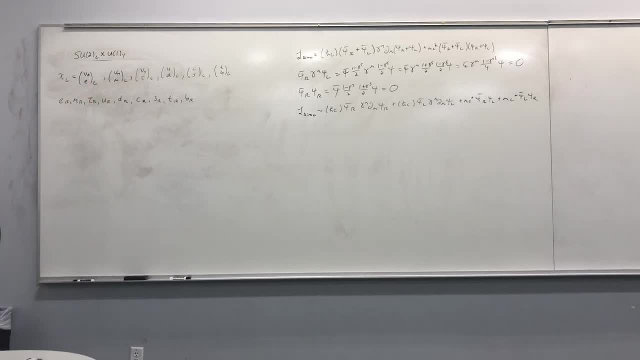 If you want to develop, in that case, Yes, yes, yes, That you'll switch, Okay, Okay, Okay Okay. So we are calling these xl. These are the doublets we are referring to. Yes, this is a doublet. 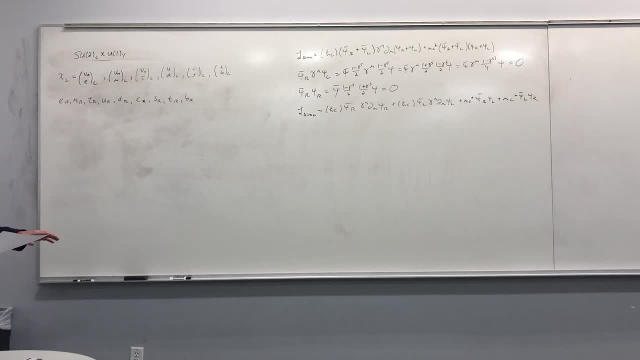 And doublets are just not singlets. Singlets- Is that put as xr or no? Well, no, I mean, this is plenty of a label. We don't have to give it another label. This is going to be. Yeah. I mean, we could just write them like this: 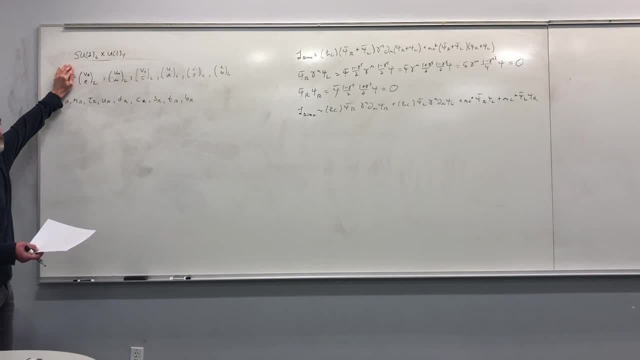 and that'd be the end of it. We don't need this label. Okay, Yes, So you said we were only taking the right-handed parts of the orange because the neutrinos have no mass. Yeah, What about? like the fork and the? 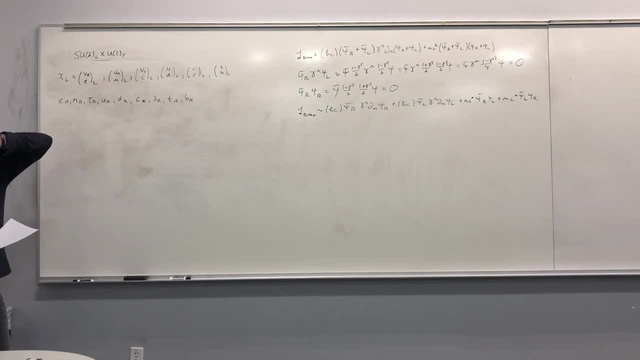 They all have mass. They don't have mass either. No, they all have mass. Oh, they all have mass. Yes, Why are we taking the right-handed parts? Why are we taking the right-handed parts? I'm sorry? Yeah, we have all six quarks now. 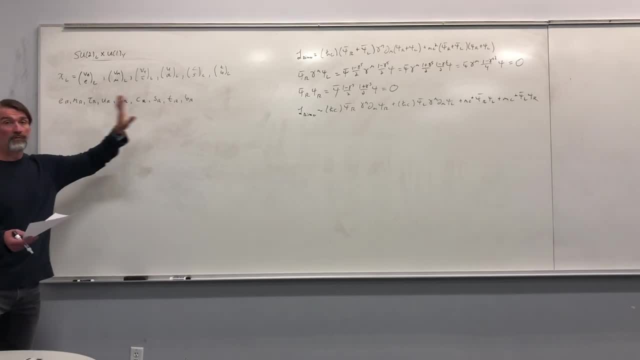 Yeah, just three leptons and six quarks. Everything that has mass, well-established, has a right-handed component. Okay, Like I said, he's got plenty of answers to all your questions about. wait a minute, those neutrinos have mass. 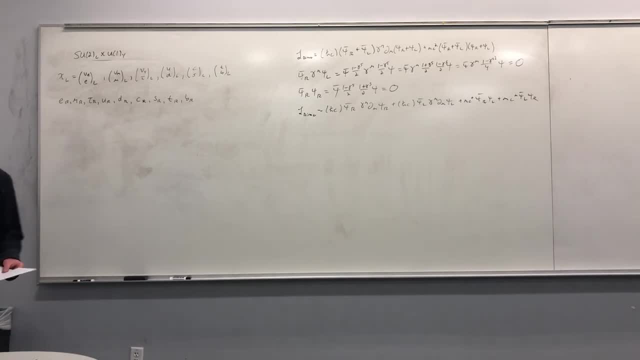 What do I do? Okay, Let me continue, because the next sheet's going to be the big, bad, ugly one. Okay, So what we're going to do- for simplicity, obviously- is we're going to focus on this and this. 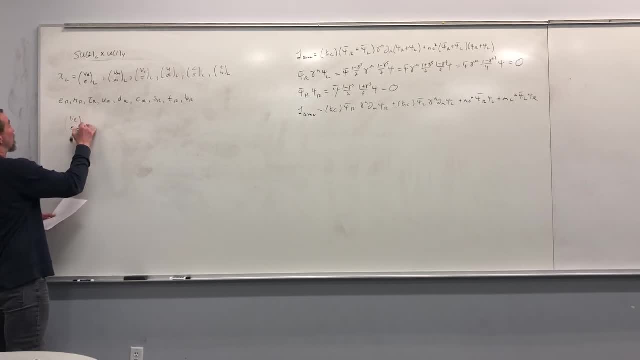 Okay, so we're just going to play our story out in terms of the electron whoops- the left electron-neutrino electron and then the right-handed electron, And everything that I'm going to play out will copy itself for the rest of these. 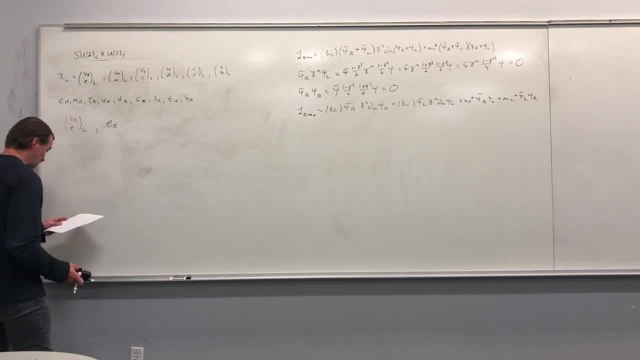 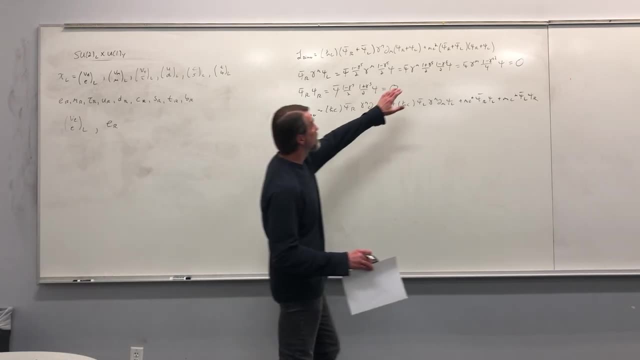 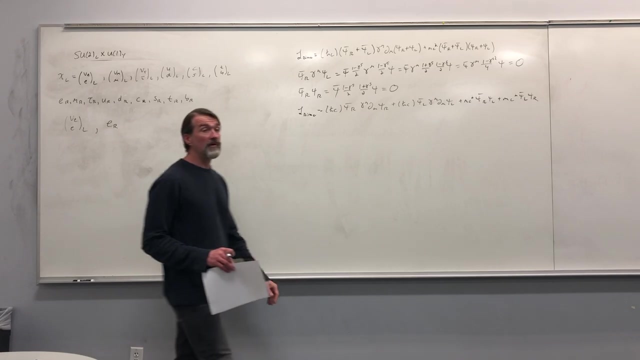 Okay, All right, And we're going to go ahead and ignore the mass term as part of this story. We'll come back to that later, But we're just basically going to focus on this derivative term, because what we want to do is we want to take this gauge symmetry. 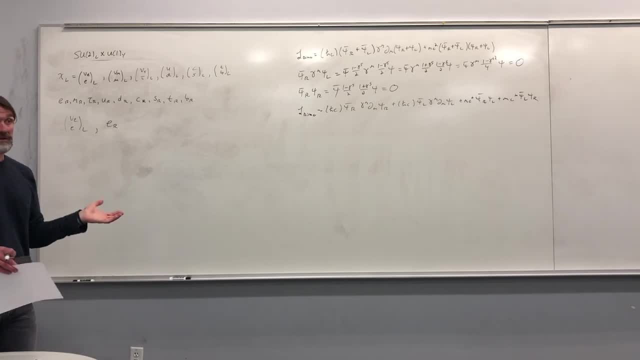 this SU2 left cross U1Y and we want to gauge it. We want to make it local, Okay, And we all know that the derivative is the term where that gets screwed up, Okay. So here we go. Let me just write down what the Lagrangian looks like. 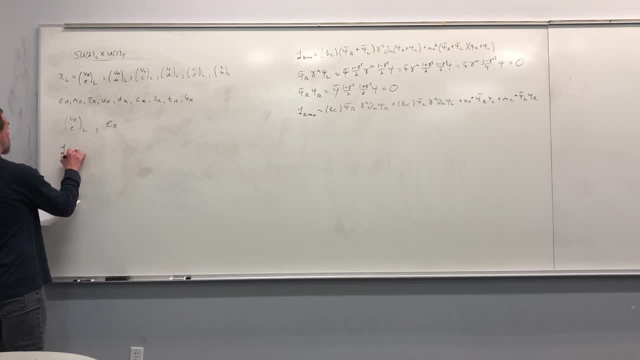 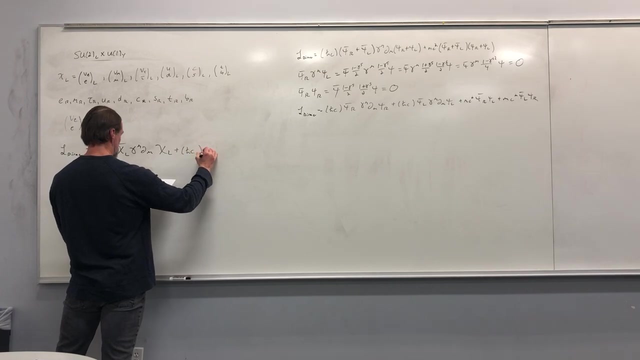 for these terms We're going to have the Dirac Lagrangian takes the form H bar C chi left. bar gamma mu d mu chi left, plus H bar C E bar right. gamma mu d mu E right. 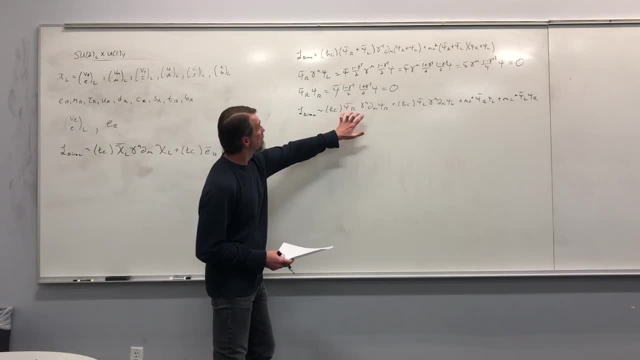 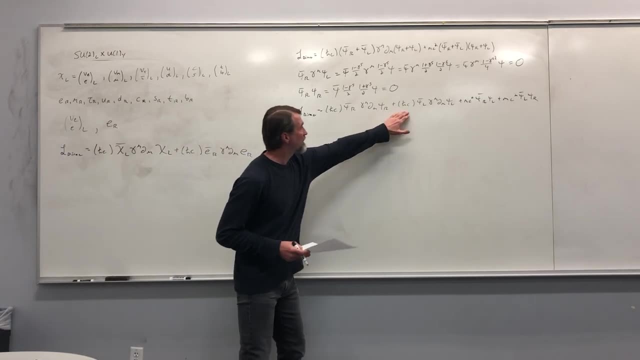 Okay, This is just this term right here for the left and this term right here, whoops. this term for the left, this term for the right. If we're doing the left, we have to include the doublets, and if we're doing the right, 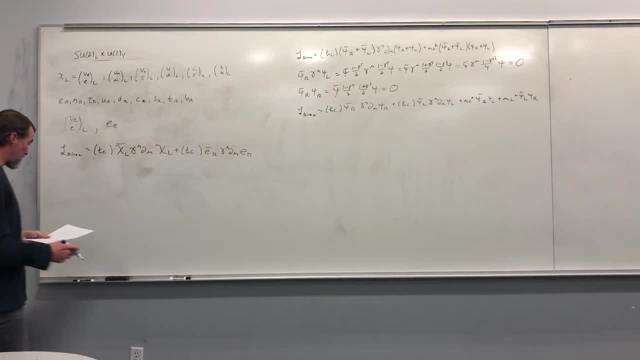 we just use the singlets. Okay, All right. Now let's go back to C. This is a pseudo-familiar ground. Let's gauge this symmetry of this Lagrangian. Let's localize it. Okay, As you can expect, this is going to be ugly. 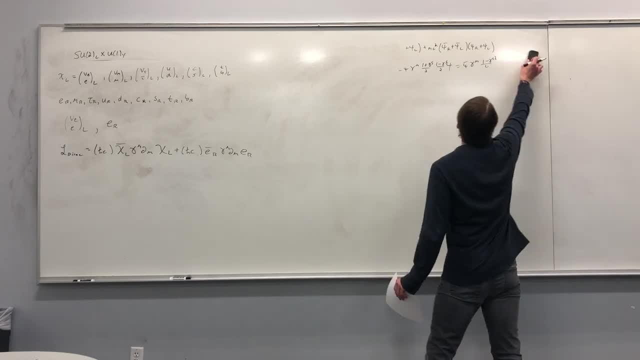 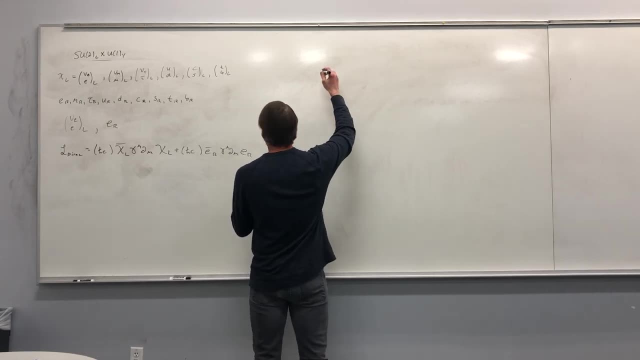 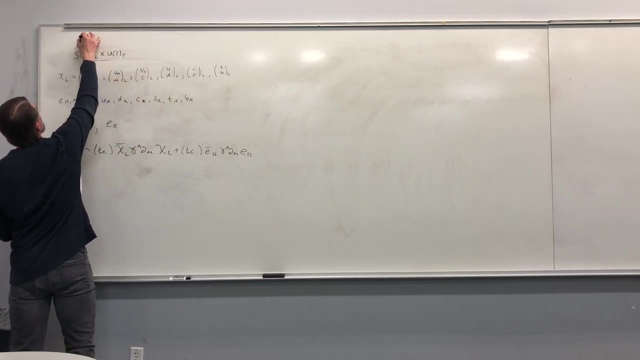 All right, Okay. So first of all, this is what is often called the isospin transformation, And I'm just giving you names. so if you want to look any of this up, you can, And this is once again given by the hypercharge. 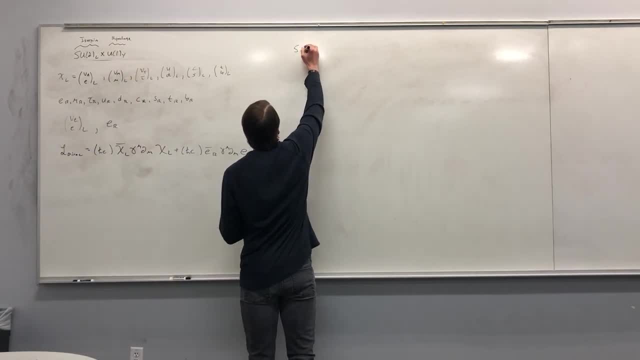 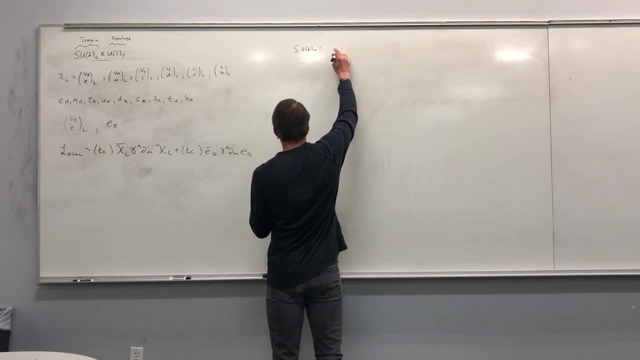 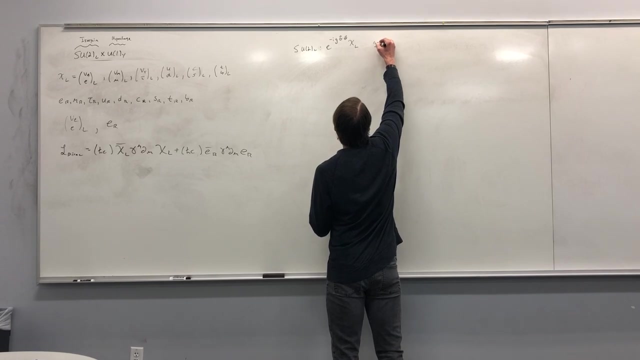 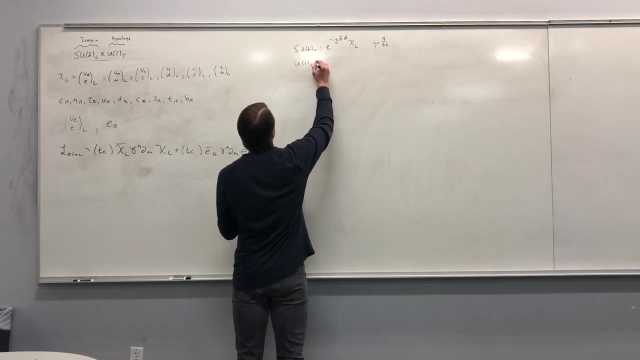 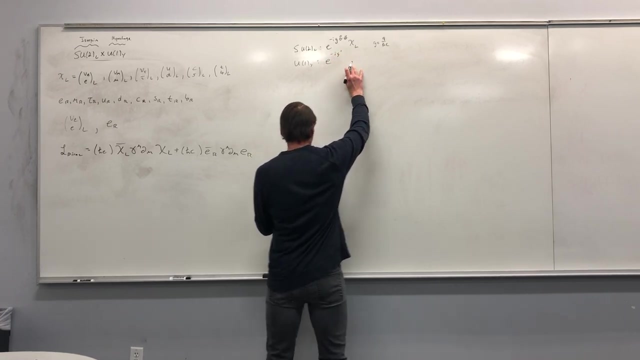 Okay, Where the SU transformations take the following form: E to the minus IG sigma dot theta chi L, where G is also Q over H bar C, And then the U1 hypercharge transformation takes the form E to the minus IG prime Y chi L. 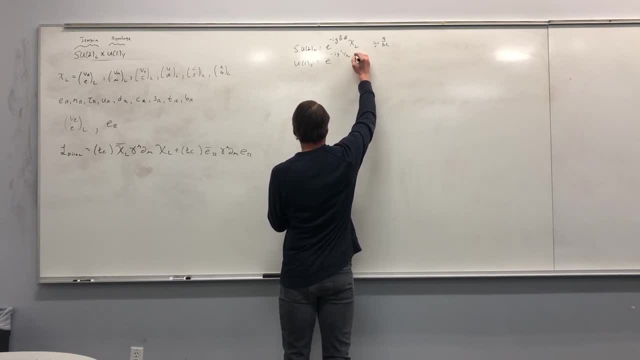 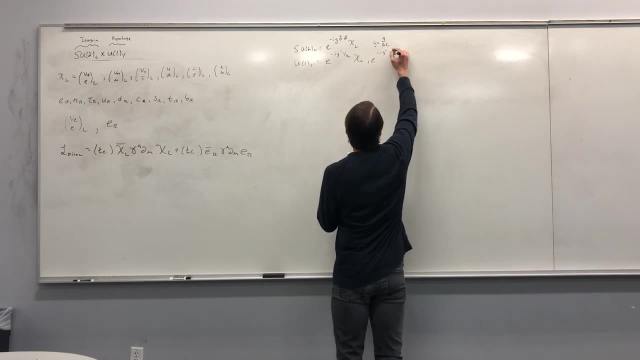 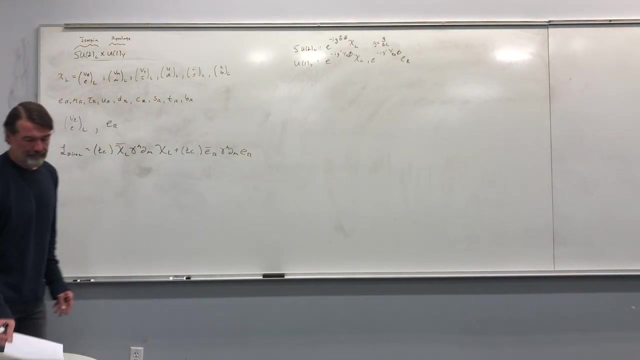 acting on chi L And then E to the minus IG prime Y ER. there should be a phi parameter in there times ER. Okay, Now let me just go over this really quickly. First of all, U1, this hypercharge. 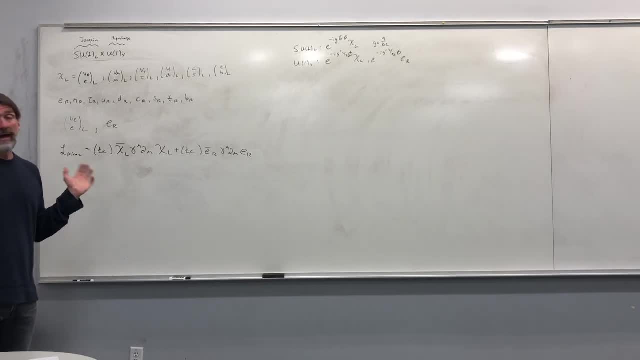 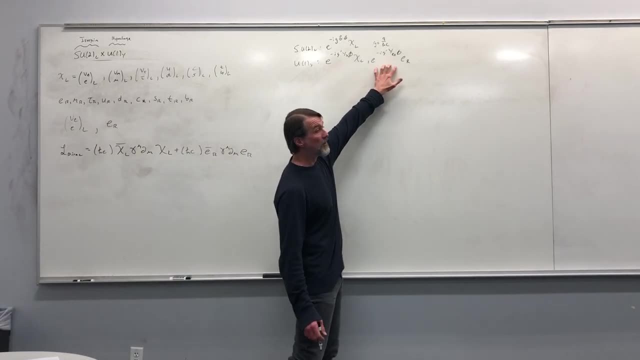 acts on both the left and the right sides. It doesn't have to just act on one side, It acts on both. So we're having this transformation: transform the left and the right-handed parts of the story. The SU2 left only transforms the left side. 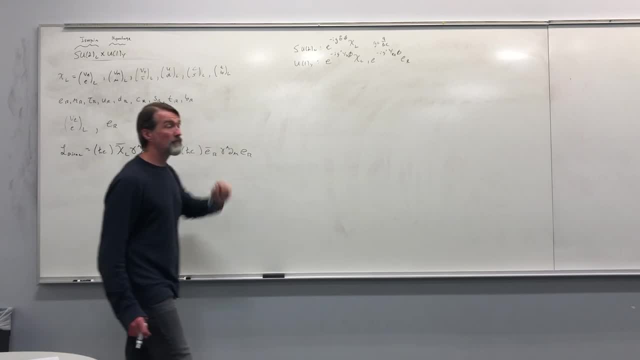 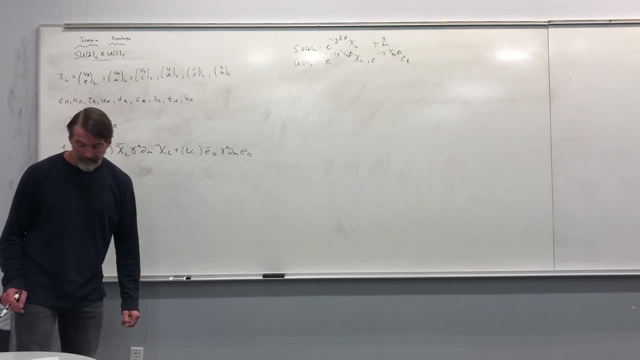 Okay, Sam, Sorry on the SU2, is that G sigma dot theta? Yeah, Okay. So once again, we've taken this and we've broken it up into a left-hand piece, which is a doublet, a right-hand piece. 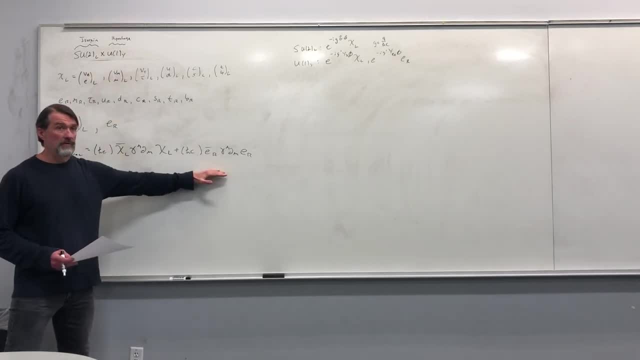 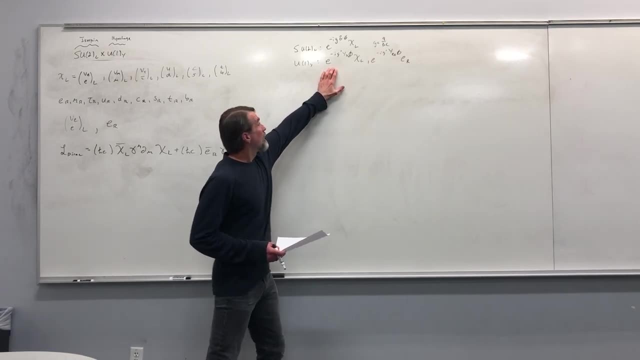 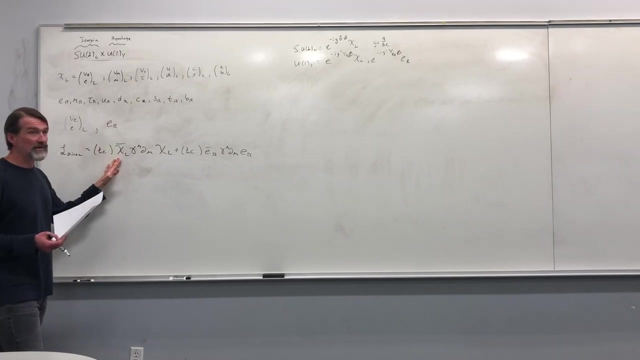 which is a singlet U1 acts on both of them. There it is, Notice U1, U1 is just a complex number. It's not doing anything to the fact that there are two pieces in this story. It's just multiplying the whole thing by a complex number. 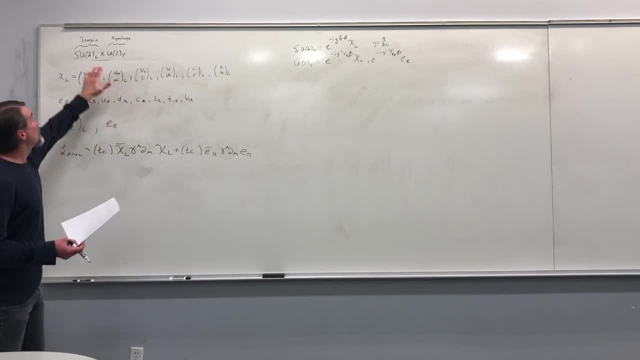 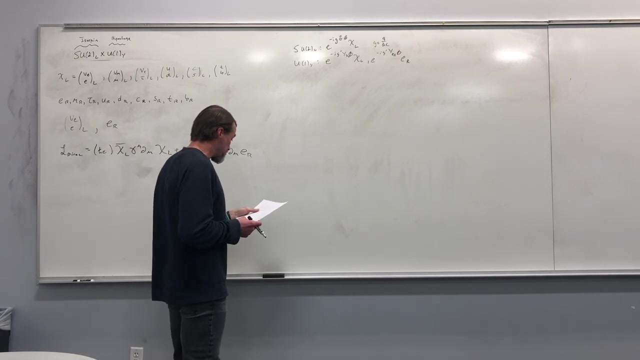 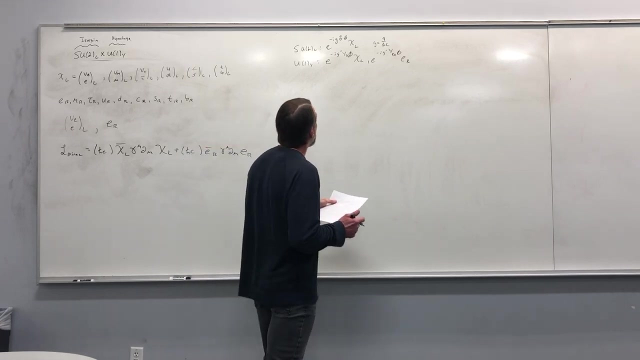 And it's multiplying this by a complex number. SU2. left is acting on these complex doublets by a multiplication by a two-by-two complex matrix And it's not touching these. Okay, All right Now. so G is obviously the coupling. 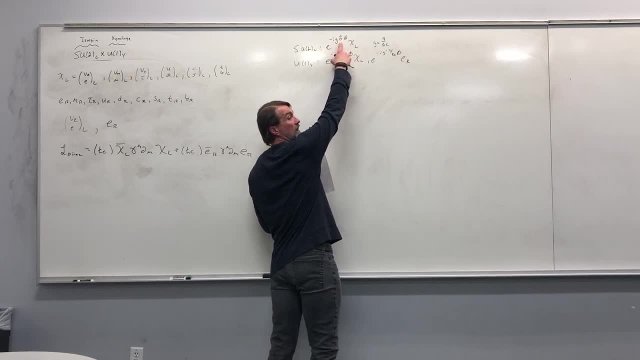 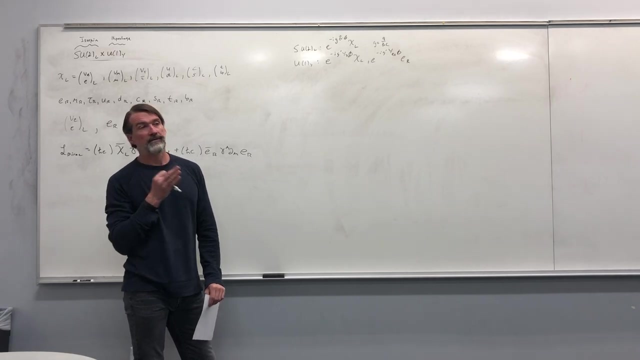 So sigma is the generators. This is the story of the exponential map. Sigma is the generators. Theta is the parameters for each generator. How many generators of SU2 are there? Seven, Eight, Twelve, SU2.. That's SU3.. 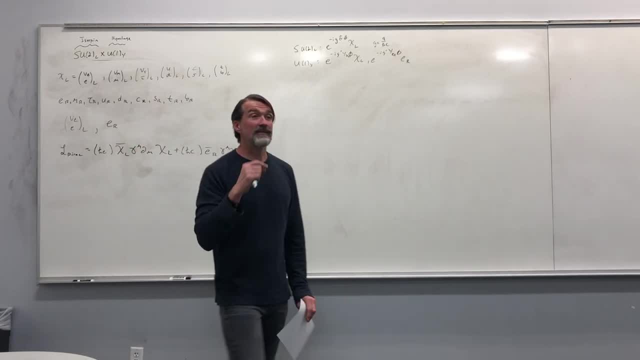 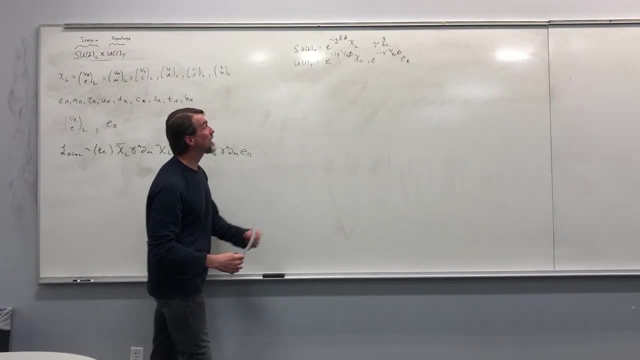 Three. There's three generators of SU2.. It's isomorphic to SO3. Remember That's how we found spinners, And SO3 has three generators. At any rate, there are three generators. There's three sigmas. Each of them gets its own parameter. 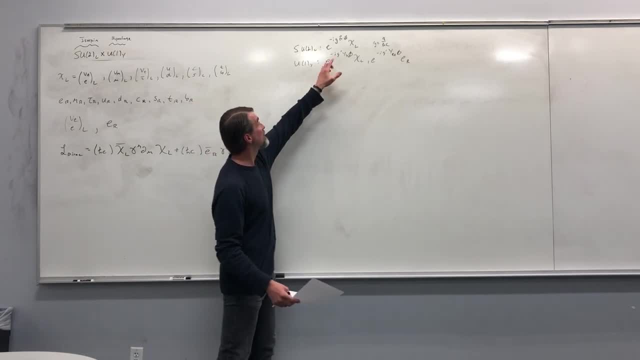 You can do this much in this generator, this much in this generator, this much in this generator. That's why we write theta as a vector of parameters. G is the coupling. Okay, Now down here again. this is just a complex number. 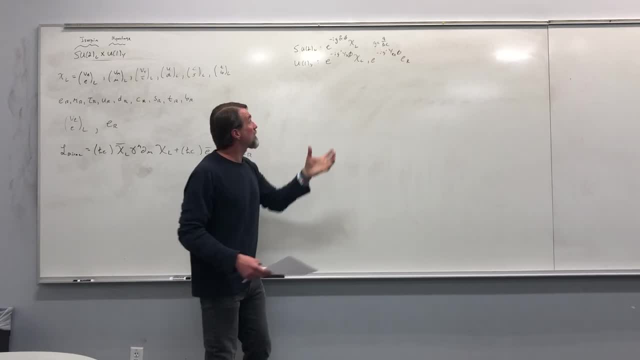 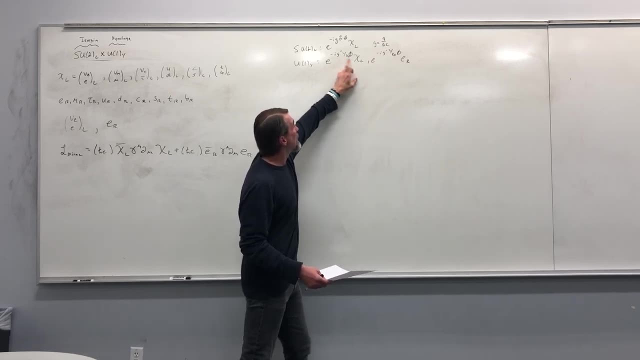 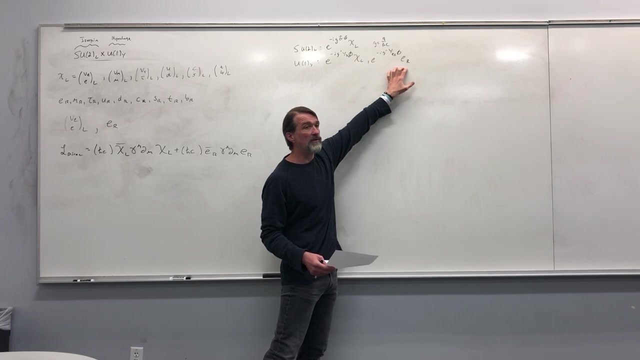 Phi is. the parameter that we're transforming by G prime is the coupling. Well, this factor of y chi left and y e right is just in case. the coupling to the left is different from the coupling to the right, So I'm going to put a G prime factor in. 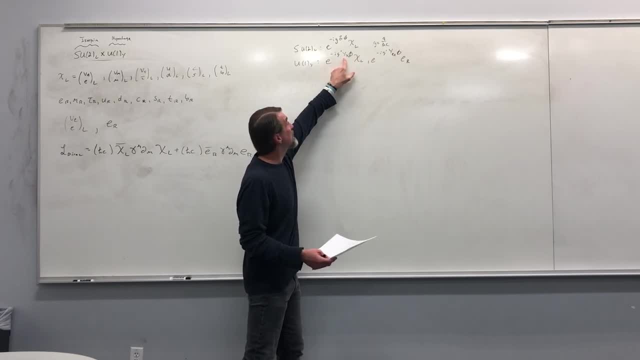 and then I'm going to let this impact overall change between this y chi l factor and this y e r factor. So this is just saying this U1 transformation might act on the left with a certain strength and the right with a different strength. 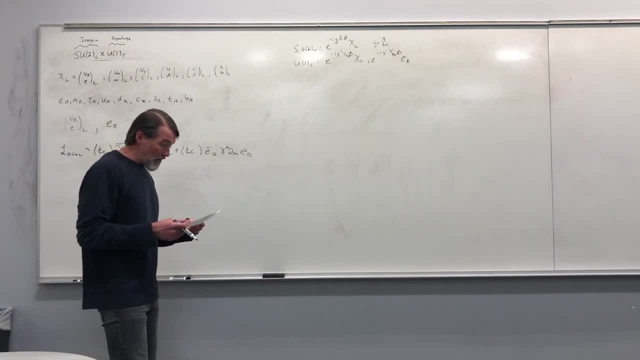 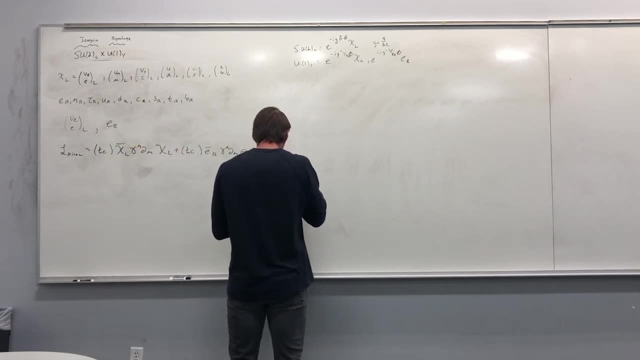 Okay, Okay, All right, Here we go. Oh boy, It's going to be a headache. So what we want to do is we want to take the ordinary derivative of the left-handed component of the story and we want to turn it into the covariant derivative. 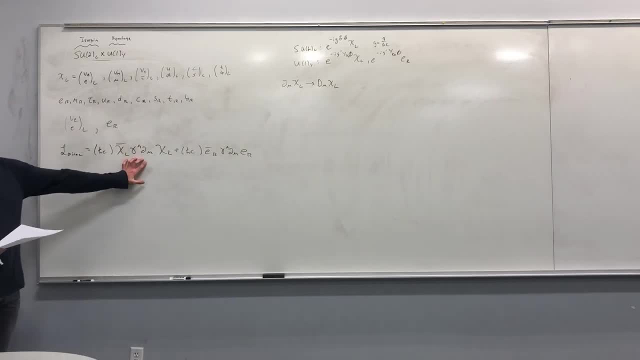 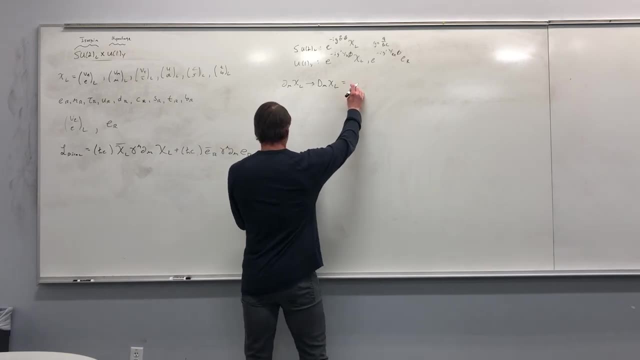 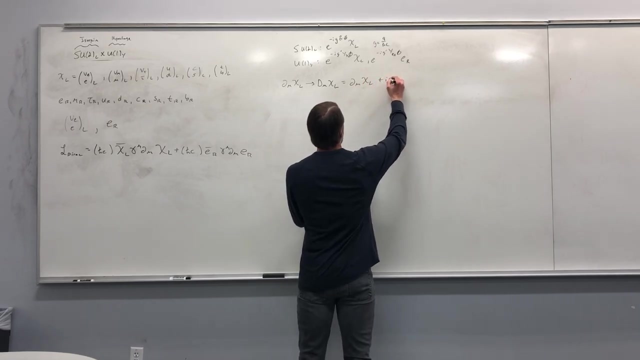 Okay, So we're attacking this term first, and then, in a few minutes, we'll attack this term. So, in order to do this, we should remember how the story goes. We get the ordinary derivative plus i, g sigma, and then we have to introduce gauge fields. 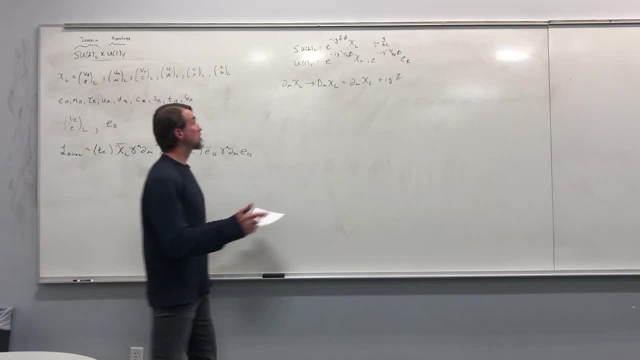 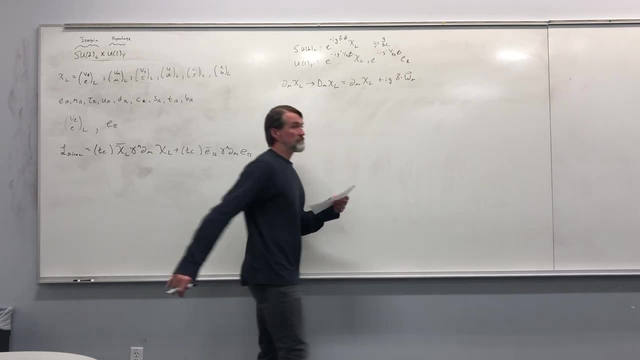 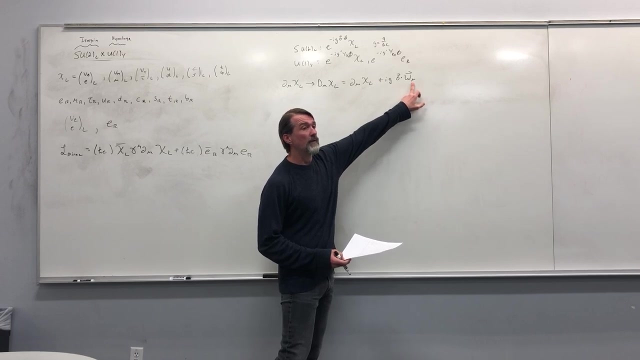 one for each generator. We have three generators, so we'll introduce three gauge fields. Okay, They are vectors in spacetime. This is just like the photon or the gluons, but there are three of them. That's why it's a little vector. 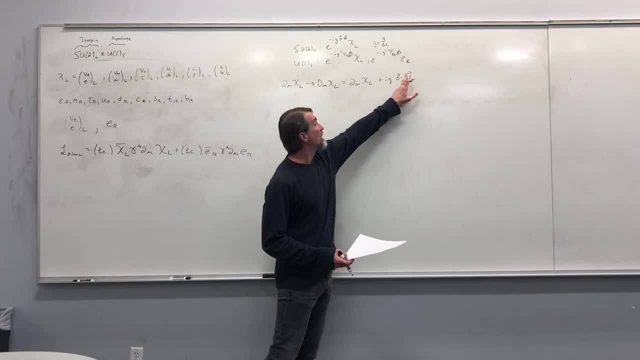 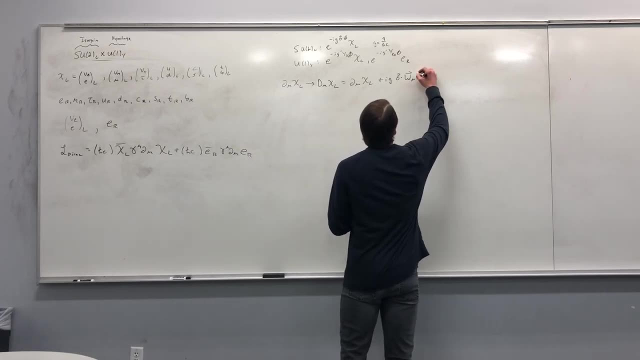 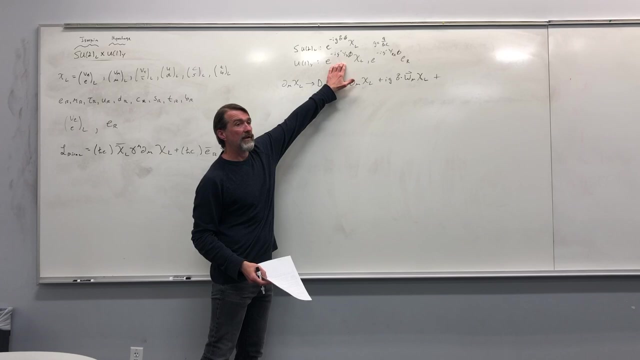 The fact that it's a spacetime vector is indicated by this mu. This vector sign just says: this has three components. this has three components. Okay, Times chi L. And then we also have this impacting the left-hand terms. So we have to gauge this. 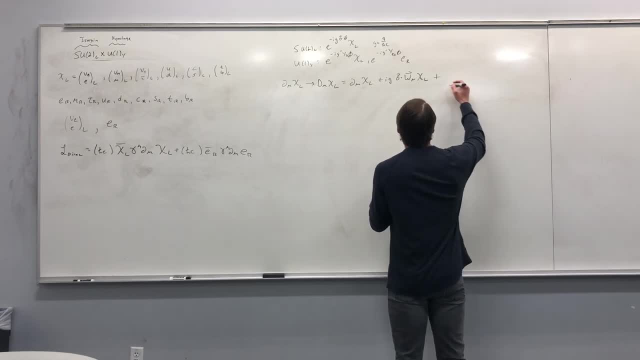 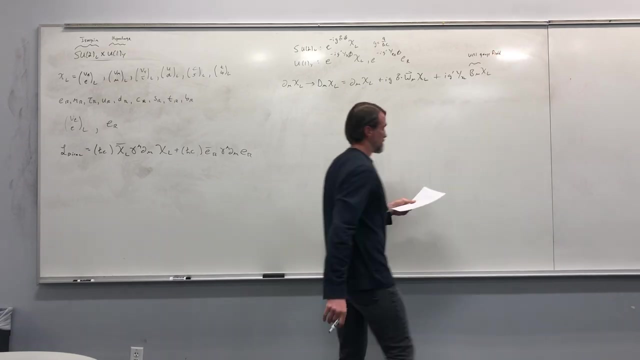 We have to include this in our modification of the derivative as well. So this is going to be: i g prime y chi L times b mu chi L. Okay, Where this is just a u1 gauge field, All right, And this, as I mentioned, 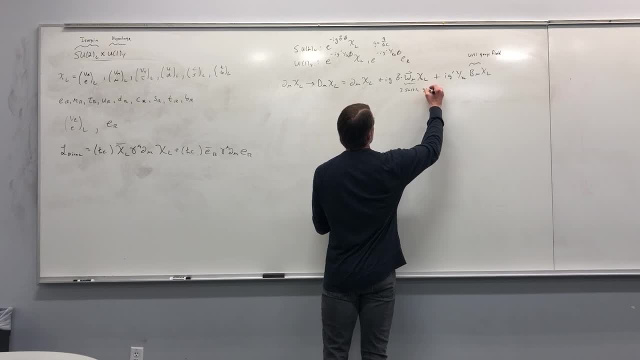 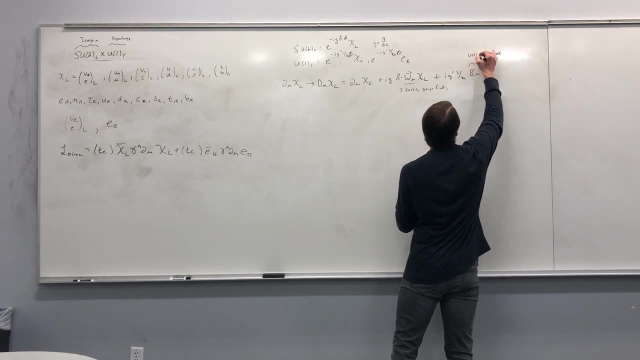 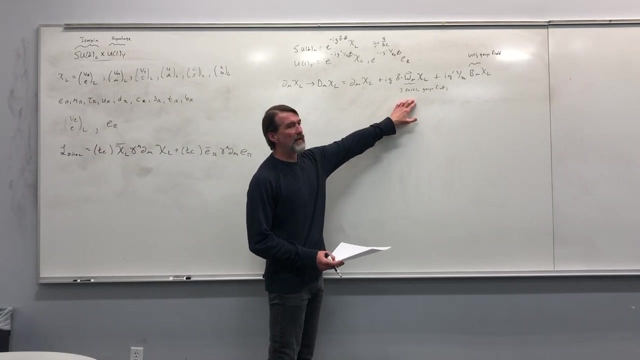 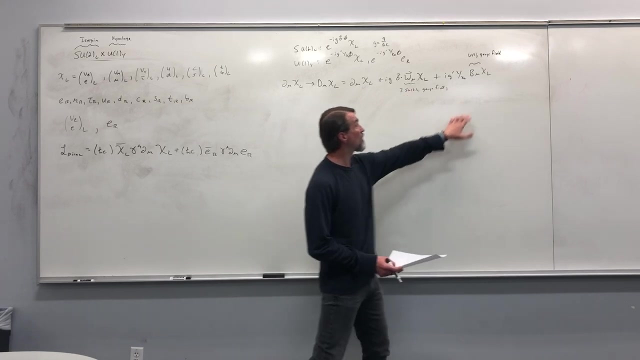 is three Su2 left gauge fields. I should say this is hypercharged. Why? Okay, So our story automatically has four gauge fields because, acting on the left-hand side of this story, we have three from Su2 left and then one from this u1 hypercharge. 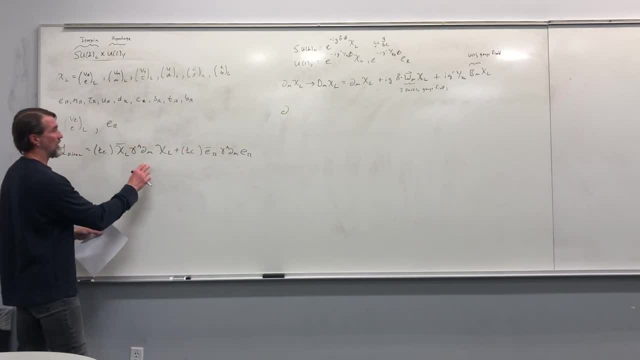 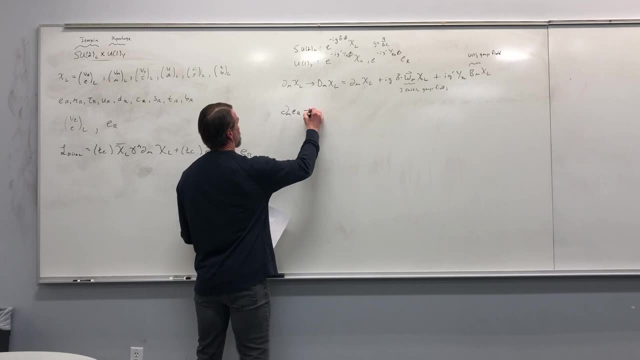 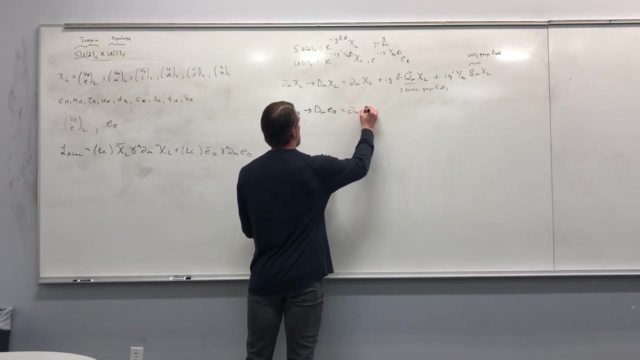 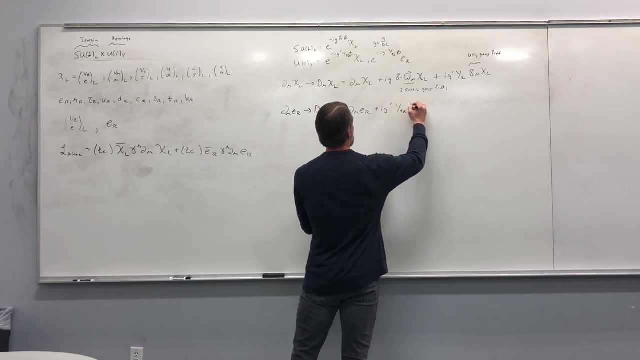 Now we also have. we have a derivative of the right-handed singlet, So this is going to have to be promoted as well, But this gets promoted in a simpler fashion. This is just plus i, g, prime, y, e, r, b, mu e r. 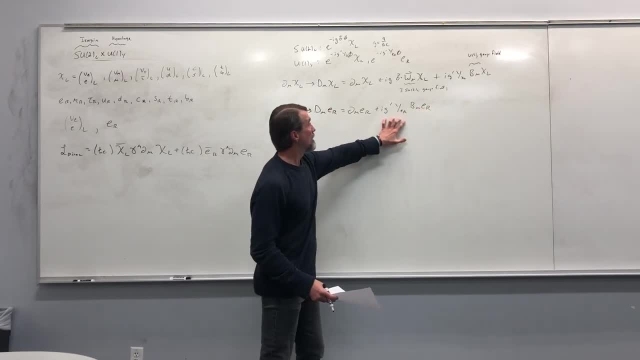 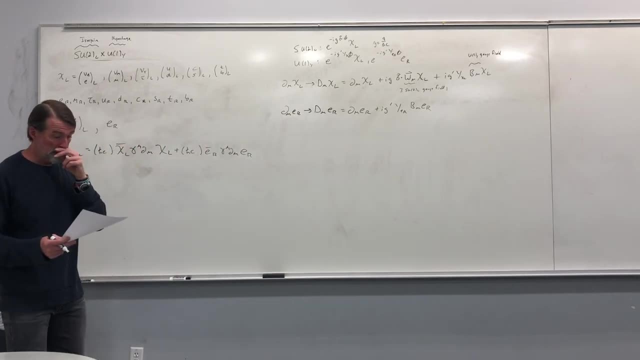 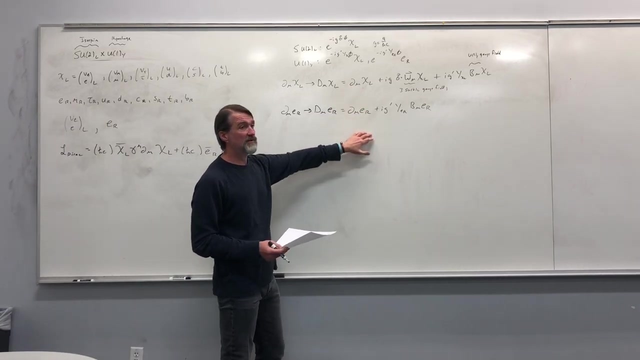 That is, we just get this term with the y e r instead of the y chi L. We don't get this term because this does not act on the right. Okay, So these are our proposed redefinitions of the derivative And what I would argue. 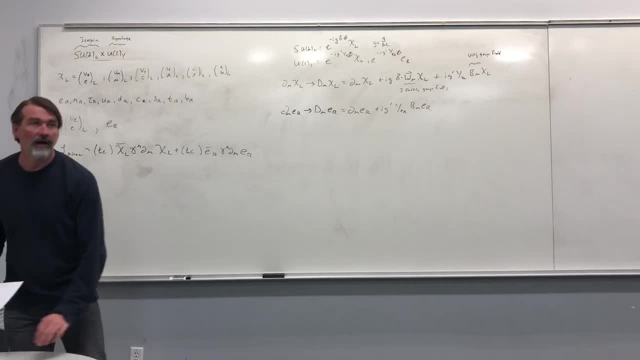 and Connor's going to help me. Connor, if I put this derivative and this derivative into this Lagrangian, what do I have to determine in order for this to be invariant with these derivatives in there? What unknowns do I have to determine? 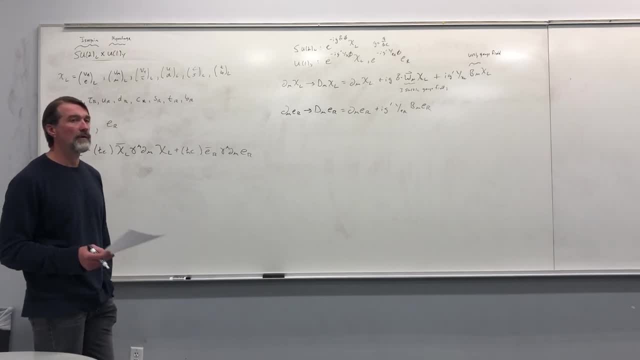 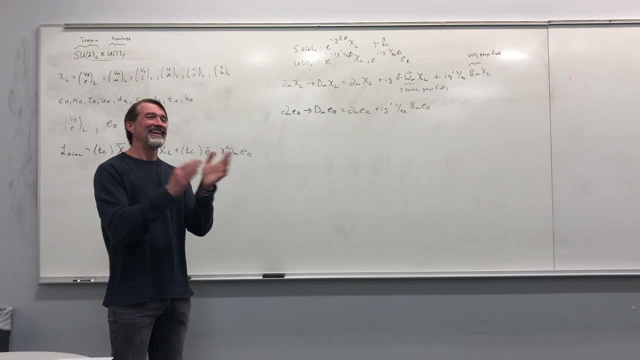 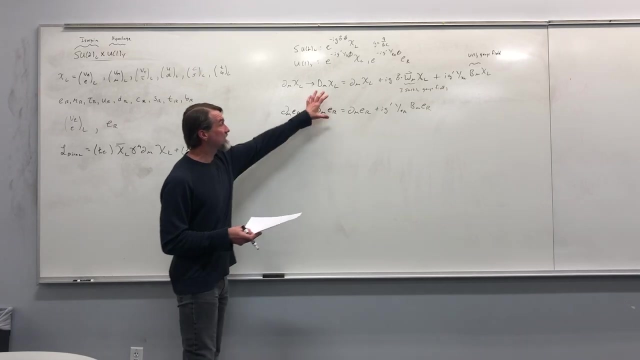 You would need to find the transformations of each gauge field. That was a perfect answer. Give the man a hand. Someone's paying attention, All right, yeah, We have to plug these in and then demanding that it be invariant. that's going to tell us how the w's. 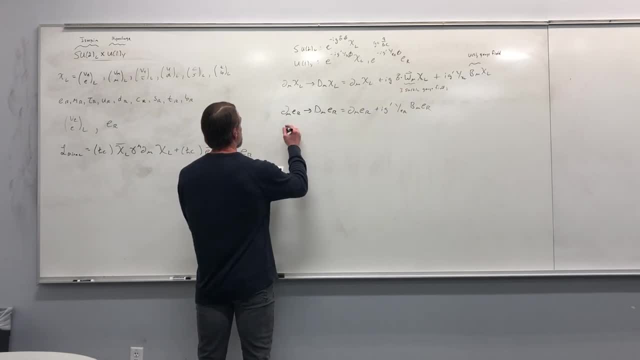 and the b's transform. Okay. So, as you may or may not remember, this is very similar to what we've already done with both the QCD, which has a non-abelian group like this one, and then an abelian group. 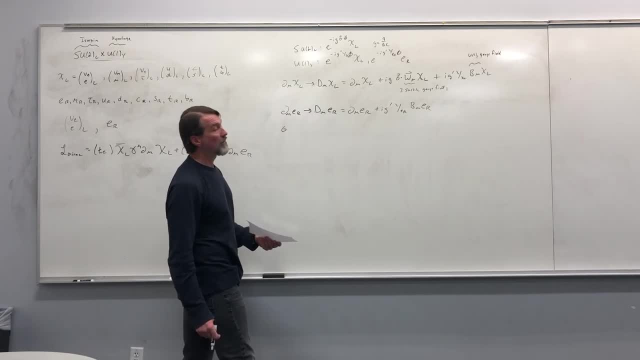 Go ahead. The y, y e r and y chi are those scalars? Yeah, those are just numbers, Yeah, Okay, so you might or might not remember in the SU story, which was a non-abelian group. 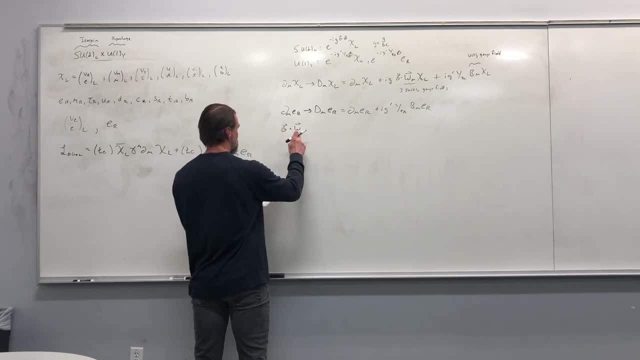 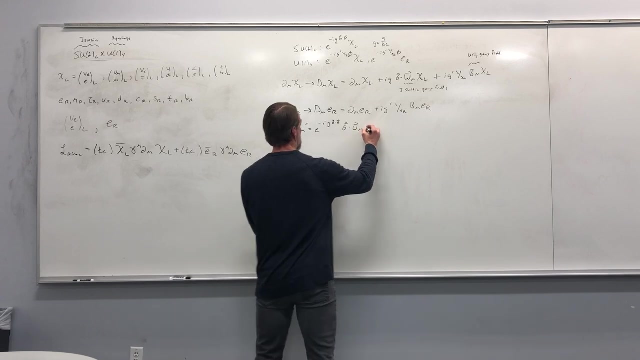 we found that the transformation has to be written in terms of the generators contracted with the gauge fields, that the primed version of the gauge fields goes as e to the minus i g. sigma dot theta. sigma dot w mu. e to the i g. sigma dot theta. 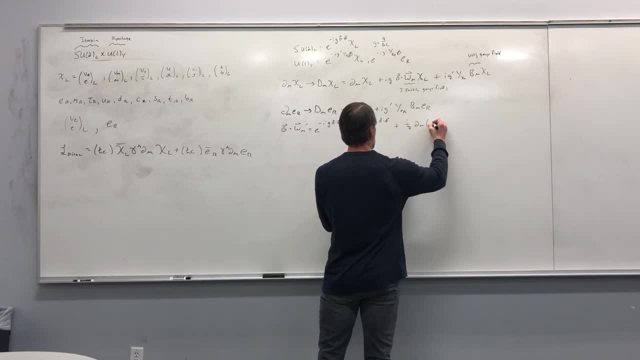 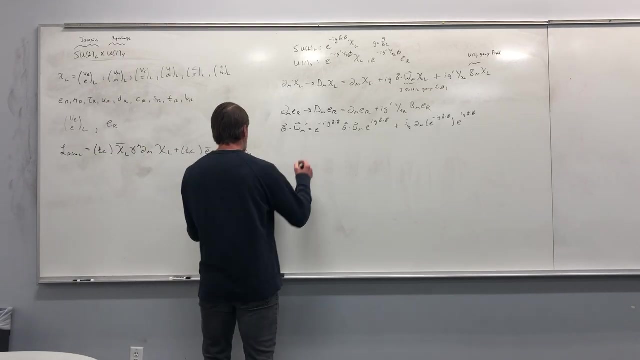 plus i over g d mu e to the minus i g sigma dot theta. e to the i g sigma dot theta. Okay, And then for the gauge, for the gauge field, for the u1, it's that simple result that it's b mu plus d mu phi. 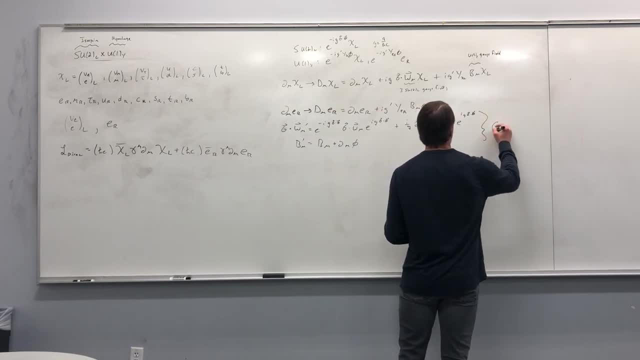 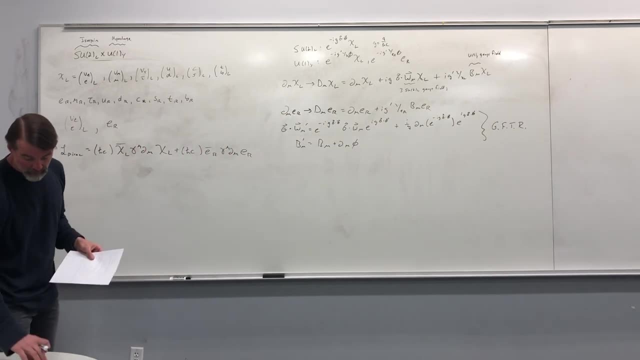 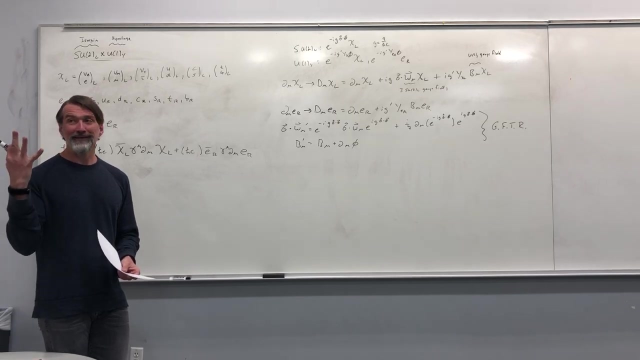 Okay, So we have here our gauge field transformation rules. Okay, Drew, Is Drew here? I don't see Drew. I have not seen Drew without a mask ever. This is the third class you've taken from me, The third class he's taken from me. 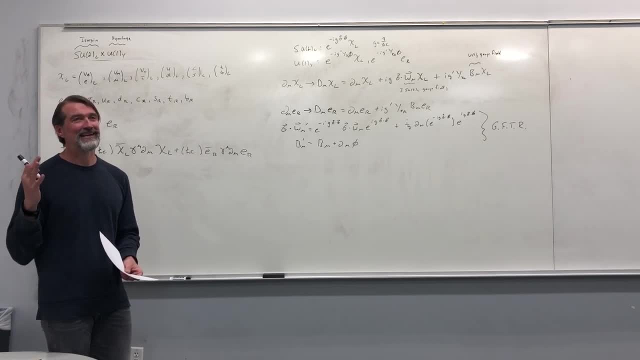 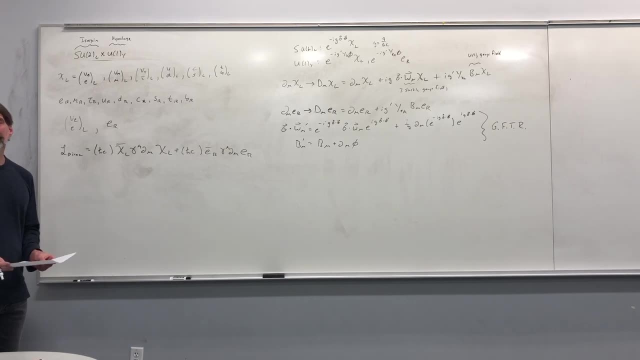 and I've never seen him without a mask. When I saw my colloquium I was like: you got Drew's hair. You're Drew, Okay, Drew. what's the next step in the story? Plug in and suffer. Plug in and what. 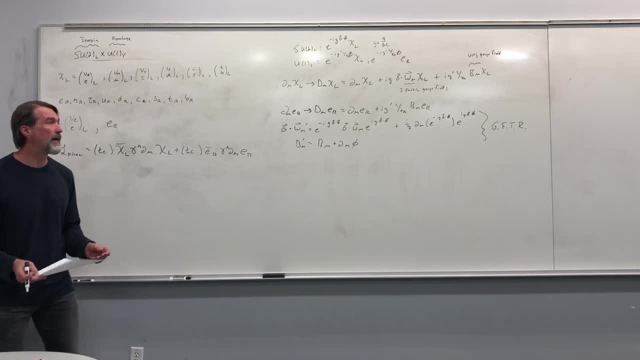 Plug in and suffer. No, no, no, Yeah, I mean, yeah, you plug this in, but there's actually, without ever planning to actually plug anything in. there's another critical step to the story of localizing the symmetry in order to get an interacting thing. 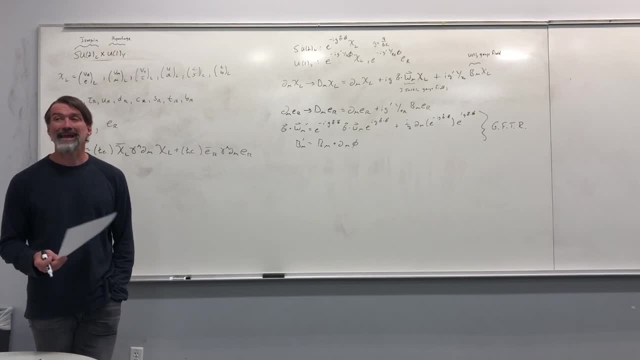 I mean, this will give us an interaction, but it'll give us an interaction between the spinner and a background Gauge field. It'll give us the interaction between the spinner and the gauge field, but the gauge field will just be a background. 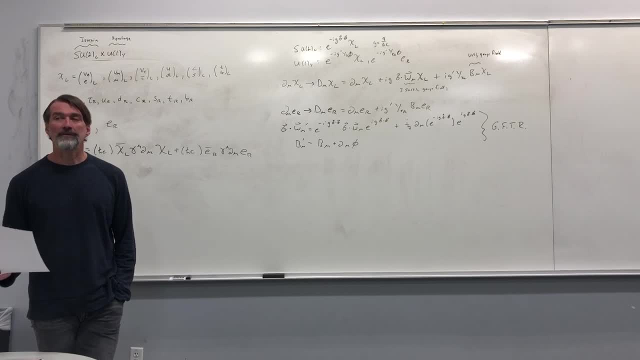 It is not dynamical. What do we have to add to the story to get the gauge field A kinetic term for the gauge field? Yes, exactly, We have to add kinetic terms for the gauge fields, okay, So remember how you do that. 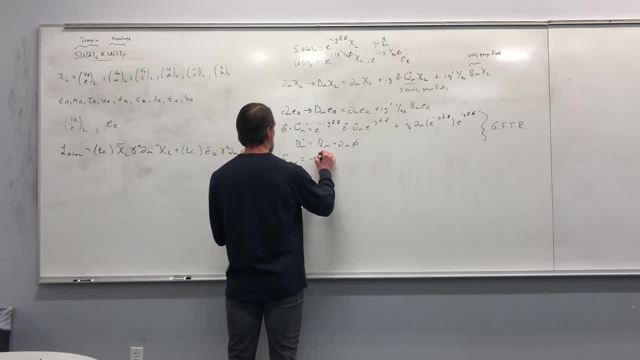 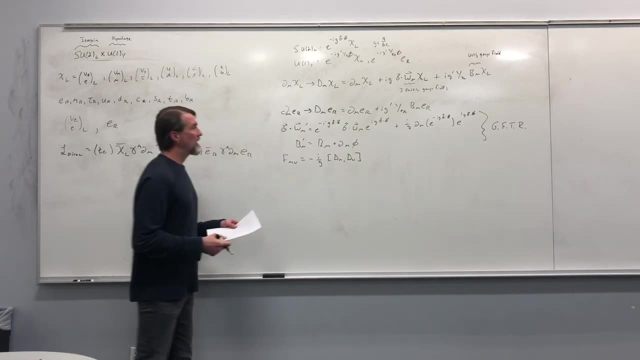 You say: okay, the kinetic term for a gauge field is just minus i, over the coupling times, the commutator of d mu, d mu, d mu, okay, which is obviously going to be different on the left and the right. So if we do this, 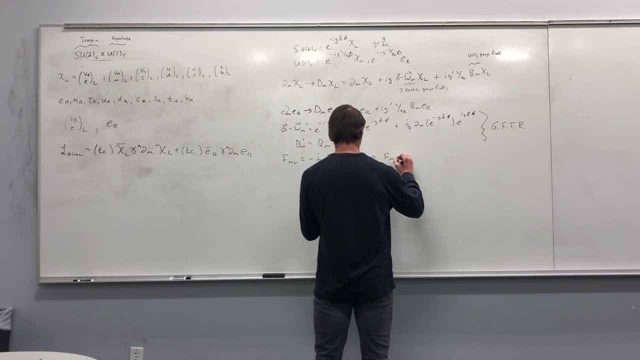 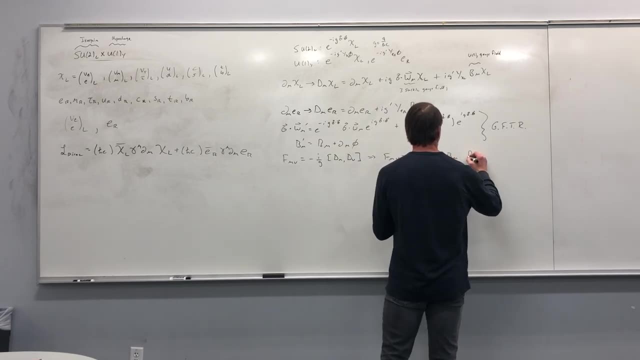 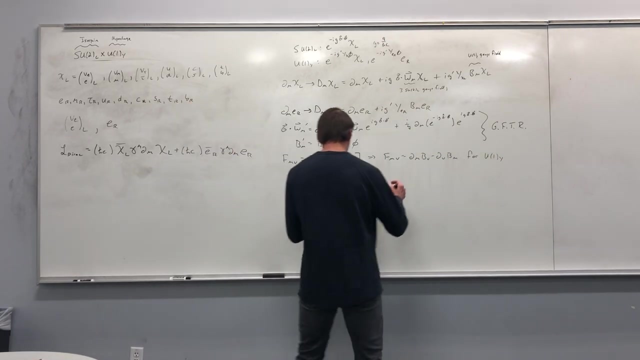 we'll find: f mu nu equals d mu b mu minus d mu b mu for the U1 hypercharge. That's what we expect. That's the same as electromagnetism, And we're going to end up with f mu nu a. 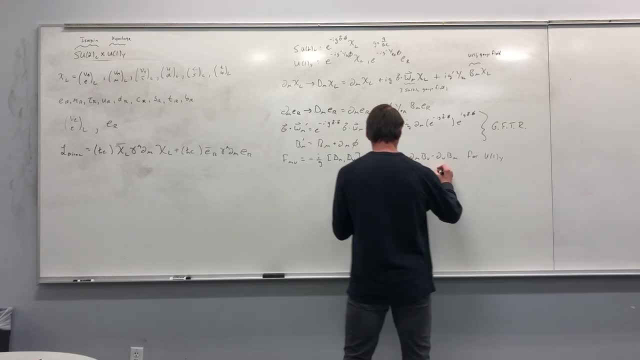 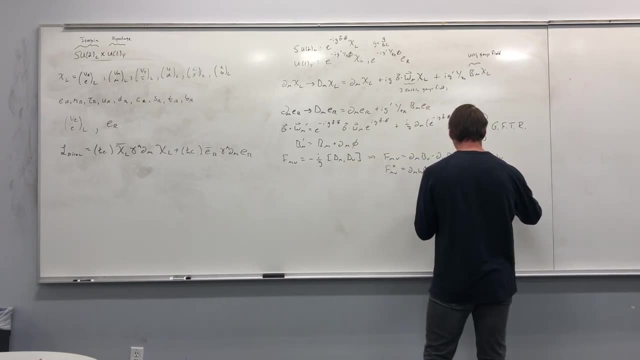 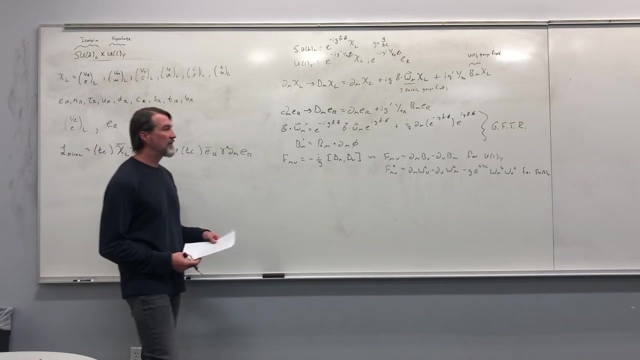 which is d mu w a nu minus d mu w a mu minus g epsilon a, b, c w mu b w mu c for SC2 left. Okay, This is a little bit different than in the SU3 case, because in the SU3 case, 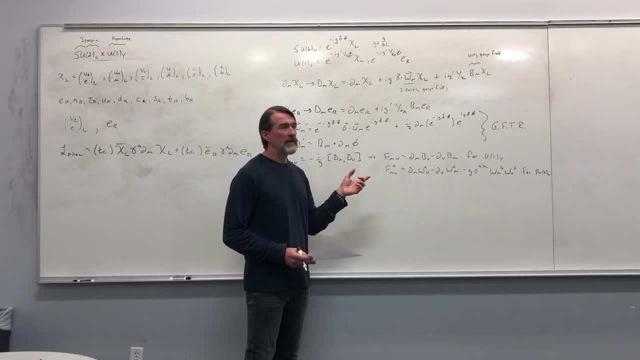 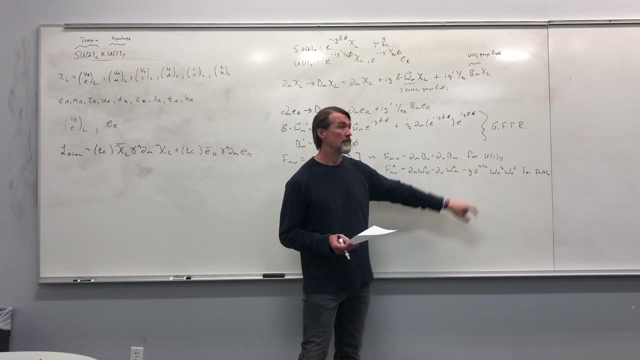 if you do the Lie algebra of SU3, you get these structure constants, these f's, and they're different values. However, SU2, that Lie algebra just uses the. let me save it as something, Okay, All right, I mean. 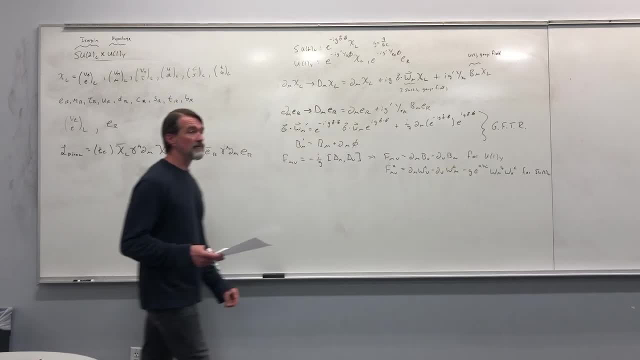 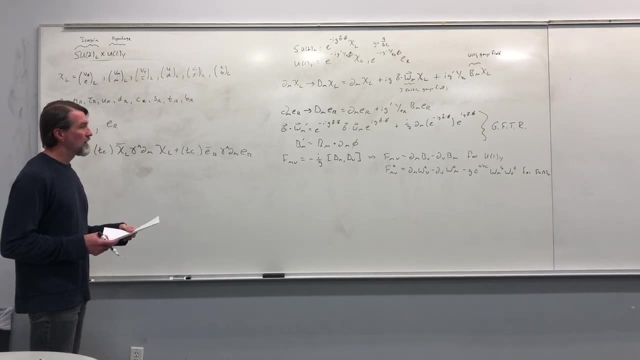 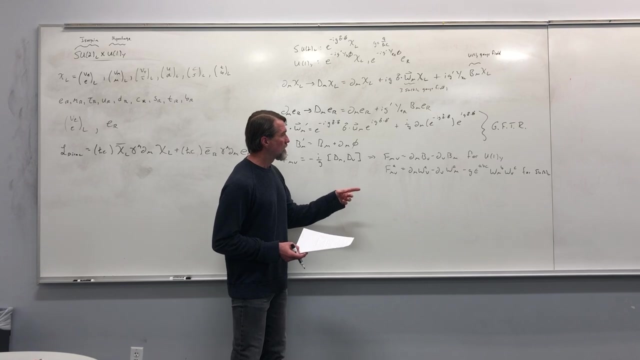 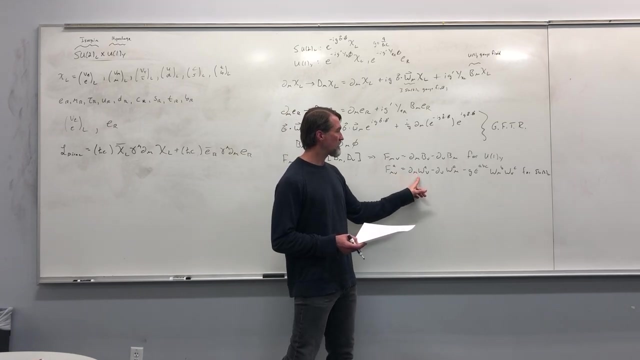 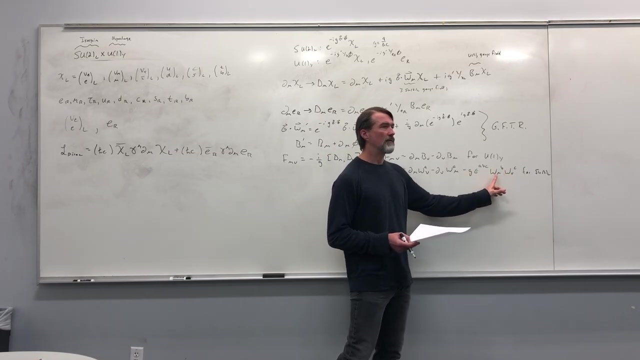 these are the structure constants of SU2.. They just happen to take that particular form. Wait a minute. SU2 left- kinetic term for SU2 left- has the derivatives of the gauge fields. Then it has these terms. What kind of terms are those? 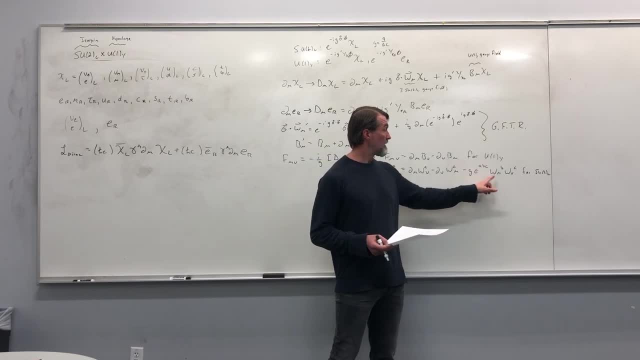 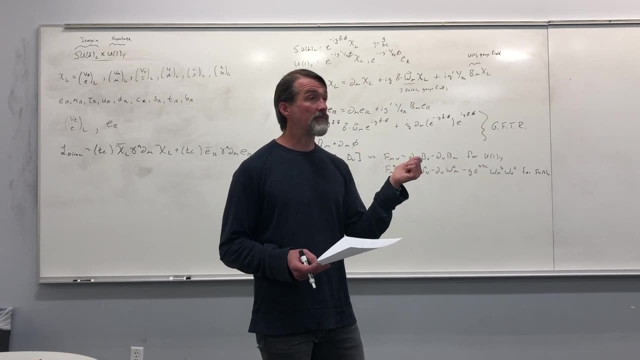 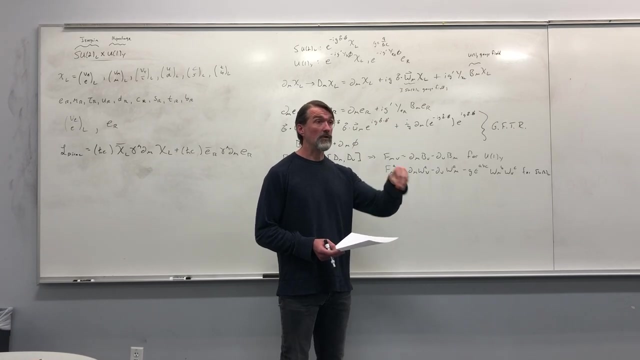 Of what? With what? Of the gauge fields with other gauge fields Exactly? Remember how for electromagnetism the photons don't interact with other photons, But for QCD, SU3, quantum chromodynamics, we found that the gluons interact with other gluons. 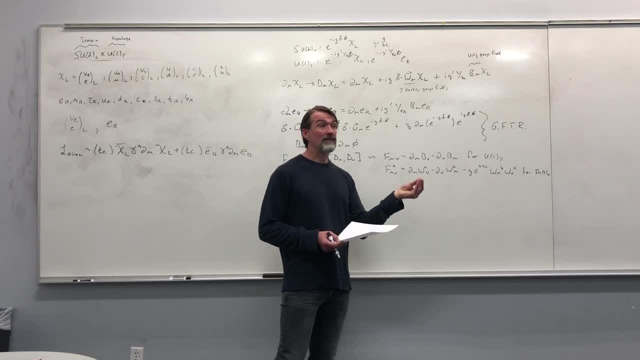 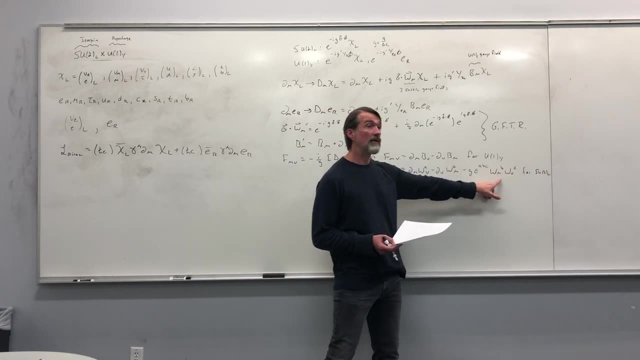 And we pinned that on the fact that SU3 is not abelian. Well, guess what? SU2 is not abelian, So the SU2 left induces interactions between the gauge bosons. Okay, But it's going to turn out to be: 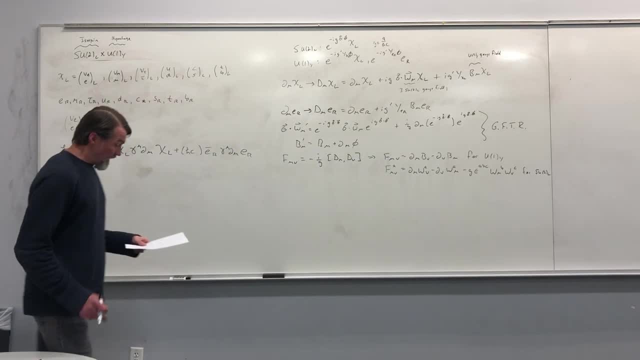 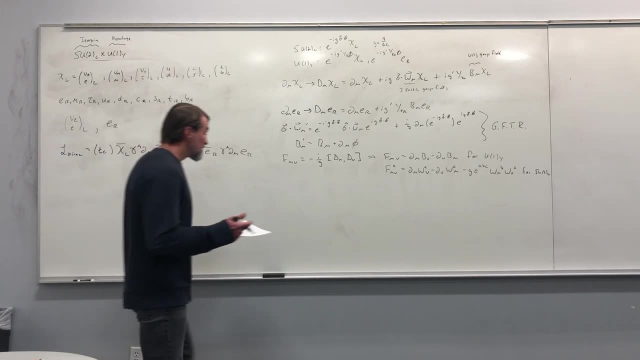 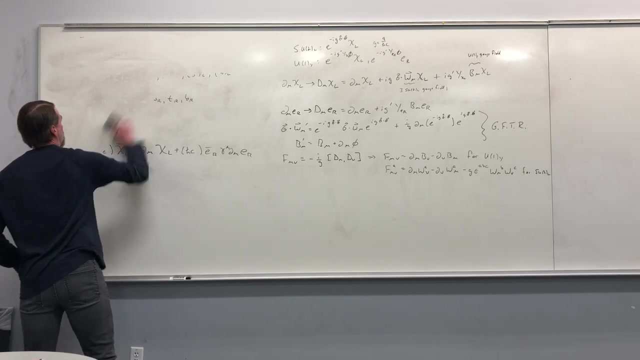 an even more interesting part of the story. Let's follow this. We expect three gauge bosons, and let me go ahead and erase this. We expect three gauge bosons, So we'll call them Wmu1,, Wmu2, and Wmu3.. 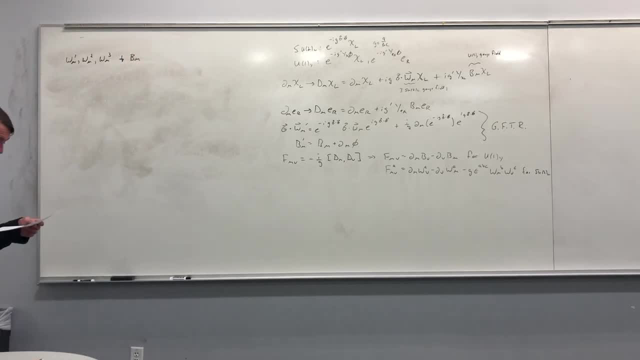 And then we have the gauge boson for the U1 part of the story. And these gauge bosons, they act on the two component parts of the spinner. Okay, Now, these are acting on these doublets. So you know. 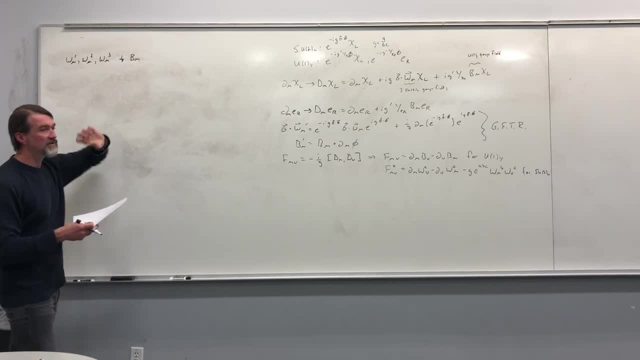 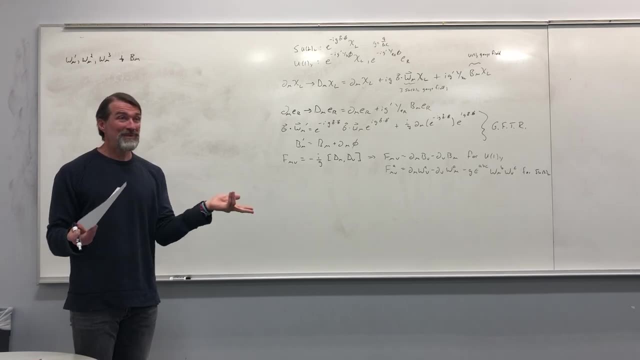 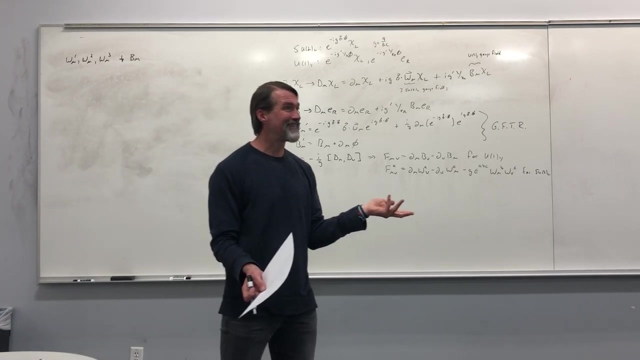 when I combine these with the generators, these are going to be two by two complex matrices. They're acting on doublets. Have we ever seen this before? Two-dimensional spinners from quantum mechanics? We've seen this, In fact. the underlying group in that story was SU2.. 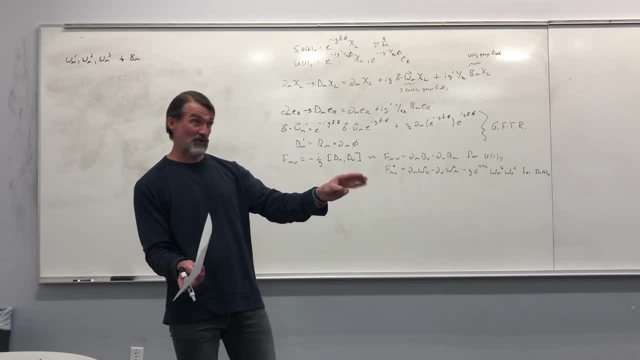 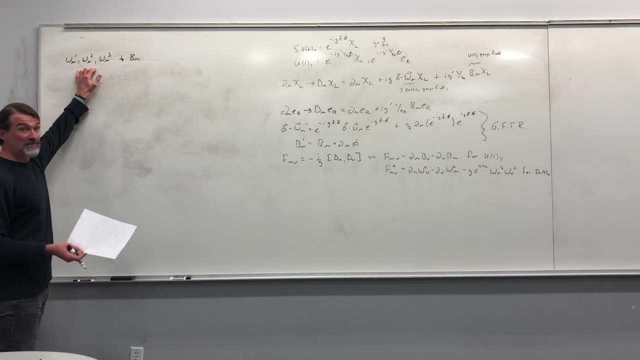 Remember, we took three spatial dimensions- SO3, and we said, oh, that's equivalent to SU2.. Therefore, you can do a two-dimensional complex spinner representation of that. Well, those same ingredients are here, even though now we're not talking about spinners. 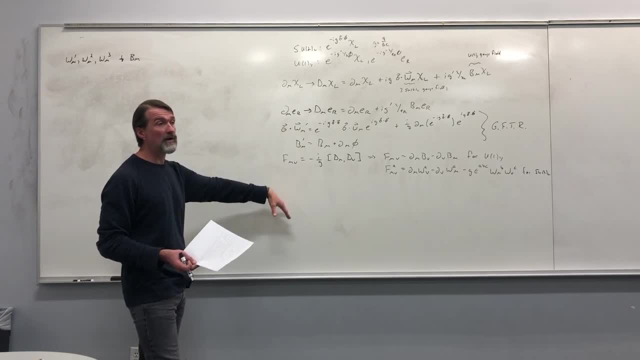 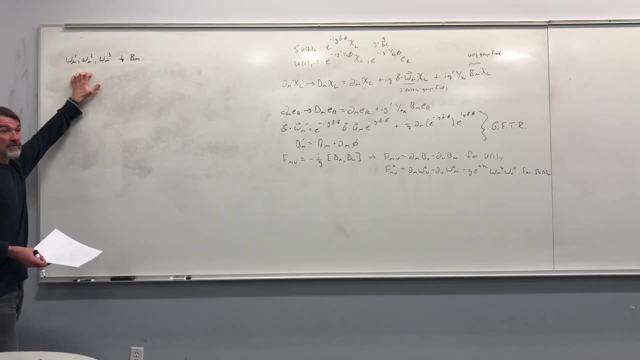 We're talking about spinners. They're a story, but they're four component objects. Rather, this is the two-dimensional space of the weak interaction. This is the doublet, which has nothing to do with space-time components, but rather flavor. 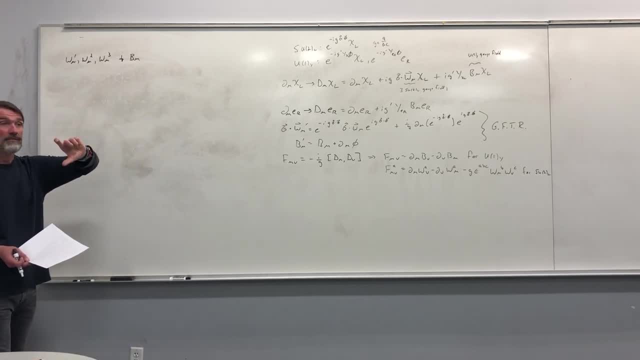 up-down neutrino electron. Okay. So we're going to use the same machinery that you use in two-dimensional spinners and non-optimistic quantum mechanics, but we're going to apply it to this space. Okay. And the reason I say that is because 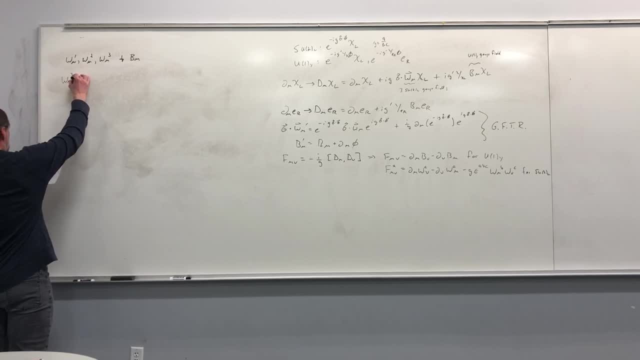 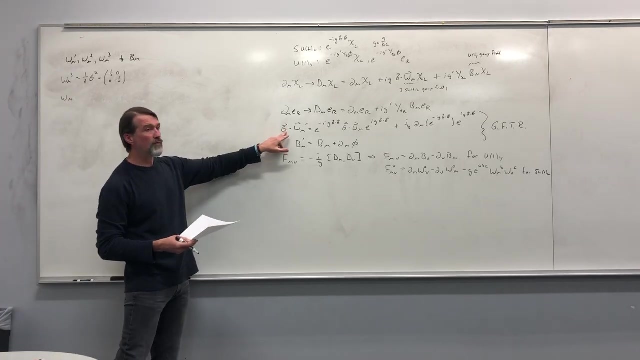 we could imagine that W mu3, which is related to, which is related to one-half sigma z. Okay, Well, if you just look at what sigma z is, that's one-half zero, zero minus one-half. Whereas if, instead of using sigma 2 and sigma 3,, 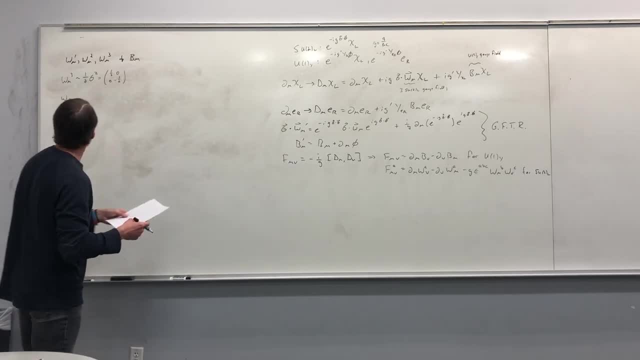 so this is using- sorry, this is sigma z. Yeah, Yeah, Using sigma 1 and sigma 2, let me combine them into a linear combination which is suggestive of what they might be able to do. Let's combine them into one-half sigma 1. 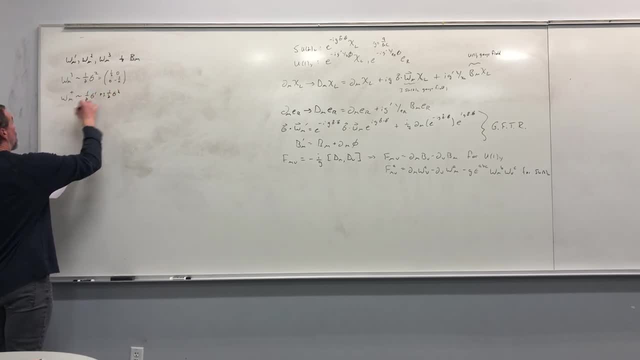 plus i, one-half sigma 2, and then W mu minus, which is one-half sigma 1 minus i, one-half sigma 2.. Hopefully you've seen this sort of manipulation in many contexts. In this case, the matrix becomes zero one, zero, zero. 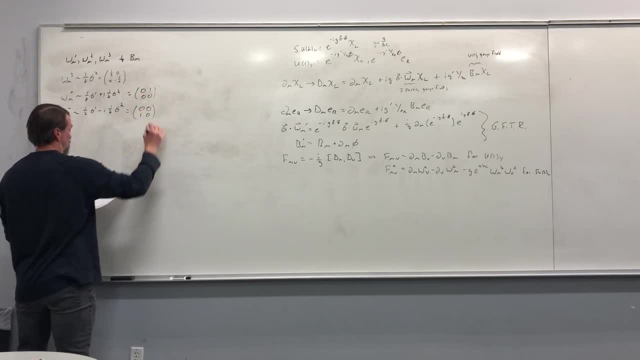 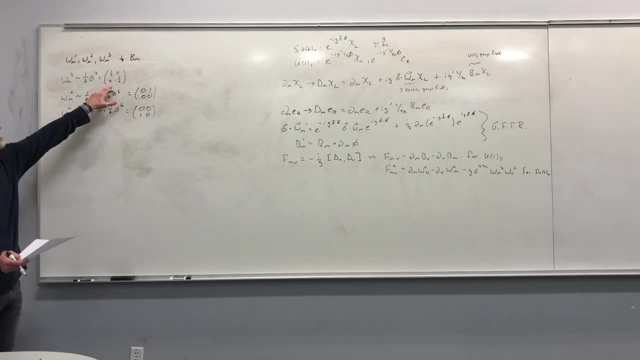 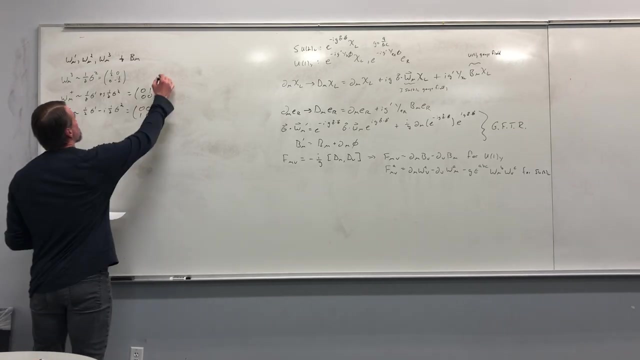 And in this case it becomes zero, zero, one zero. Okay, So really simple matrices from these linear combinations. And then this is obviously a simple matrix, But now let's watch what happens. This is where it gets really interesting. 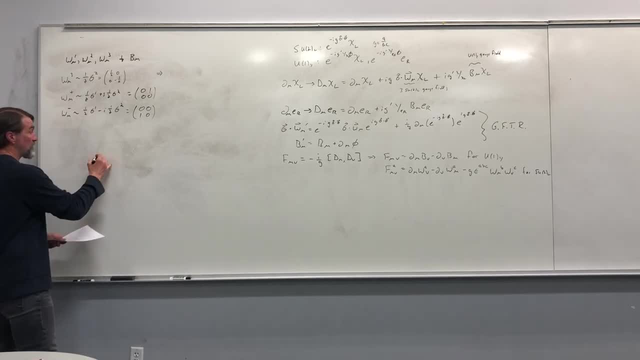 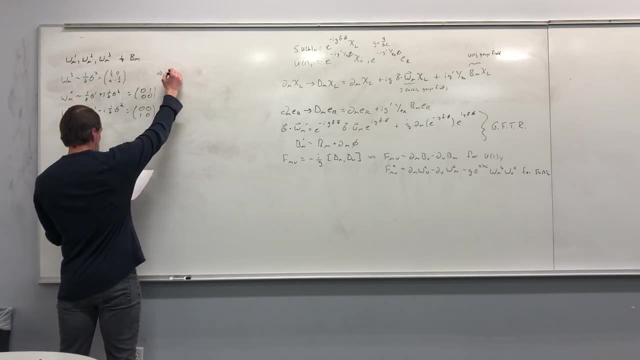 If I take a doublet- and you remember, by a doublet I might mean the electron neutrino and the electron, Okay, If I take a doublet and I act on it with this, well, if I start out in the state, 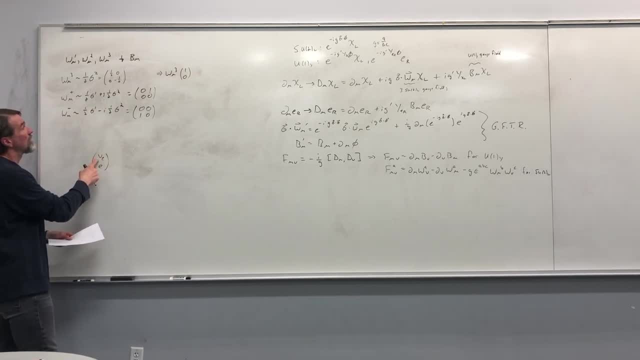 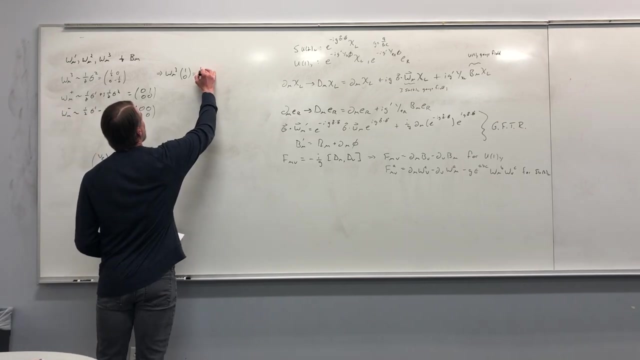 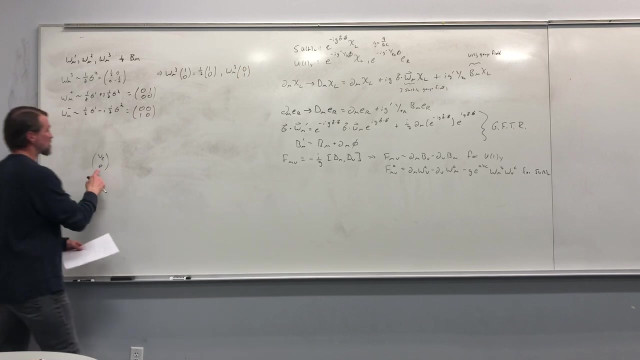 of the electron neutrino. what do I get when I act on it with this? If I multiply this matrix times this- folks, I'm making this easy- You get half- Yeah, you get half of what you started with. And if I do this on just an electron? 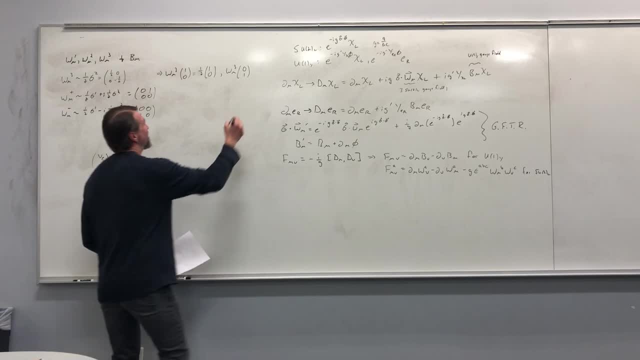 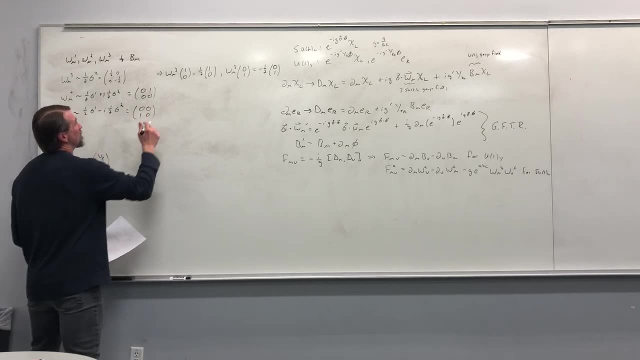 I'll get. Thank you, You guys are getting braver and braver as we go. Okay, So what this says is: if I am using this gauge boson to mediate an interaction for an electron neutrino, I have an electron neutrino come in. 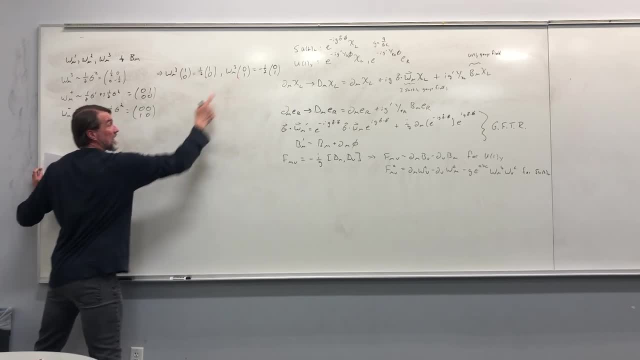 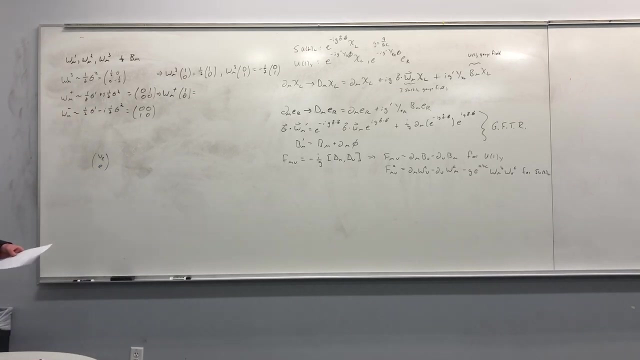 and an electron neutrino go out. If instead it's an electron, I have: an electron go in and an electron go out, Okay. But now let's consider W mu plus on. What do I get? I get nothing, Okay. 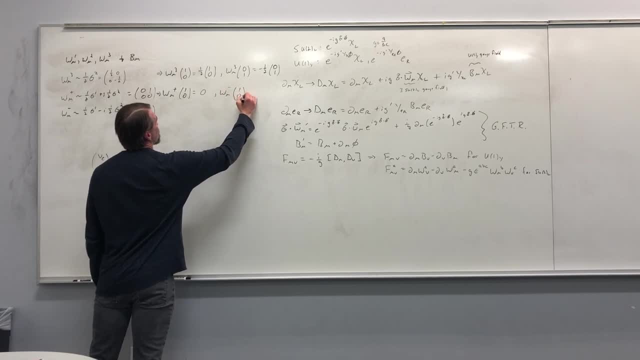 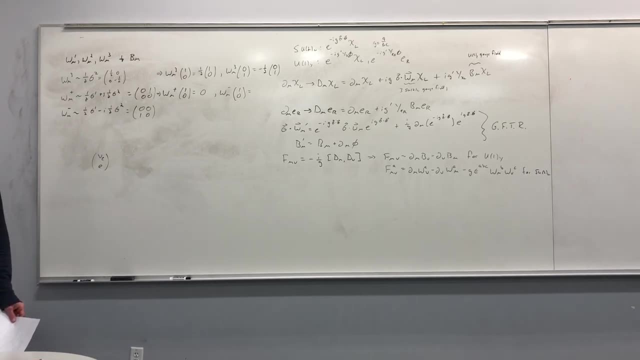 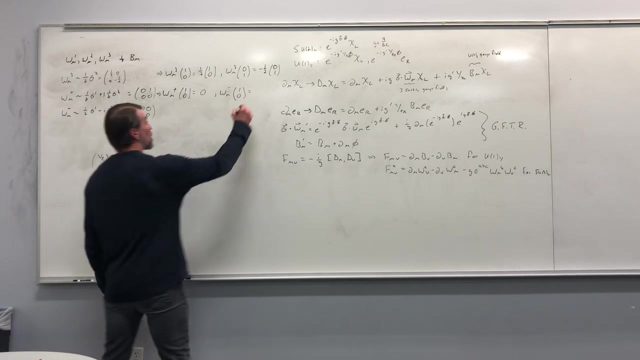 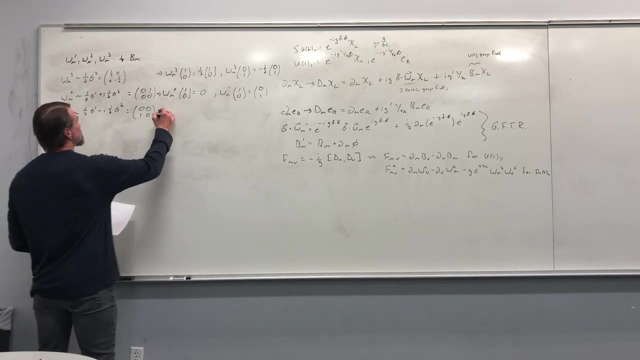 However, what if I act with W mu minus Any takers? It's, If I take this matrix and multiply that vector by it, I get Okay. Similarly, if I do W mu minus on, That's going to give me. 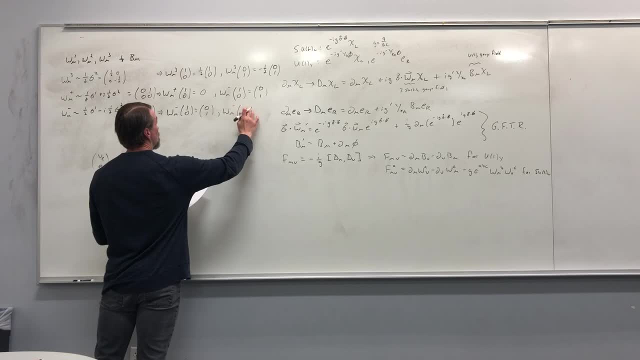 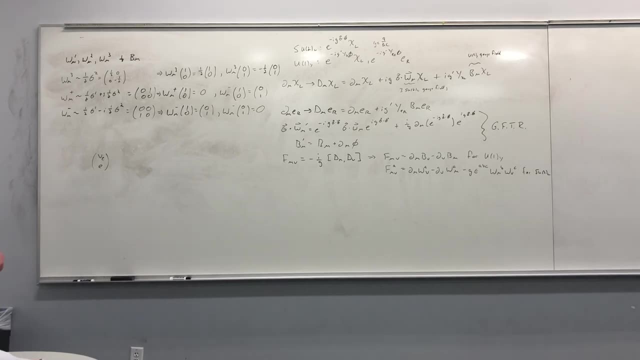 And if I do W minus on, It's going to give me Okay. Yes, Should the first line both have W, mu plus. Sorry, yeah, That should be plus. Okay, Now are you ready? We're going to have some insight. 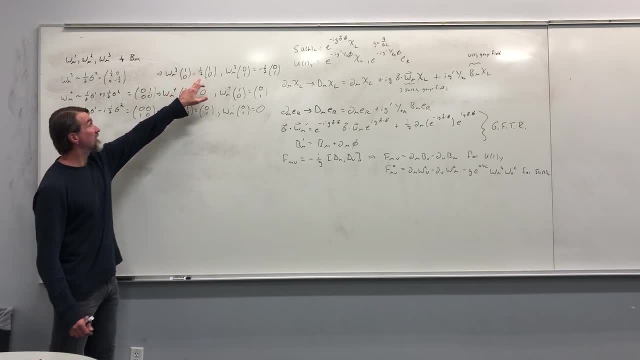 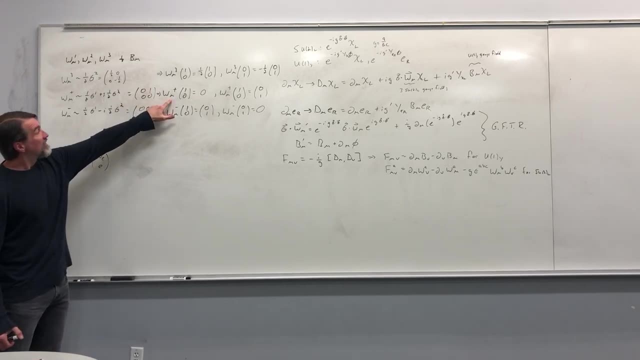 This thing is taking a neutrino and giving us back a neutrino. It's taking an electron and giving us back to an electron. Okay, This thing is taking an electron neutrino and giving me back nothing, but it's taking Oh shoot. 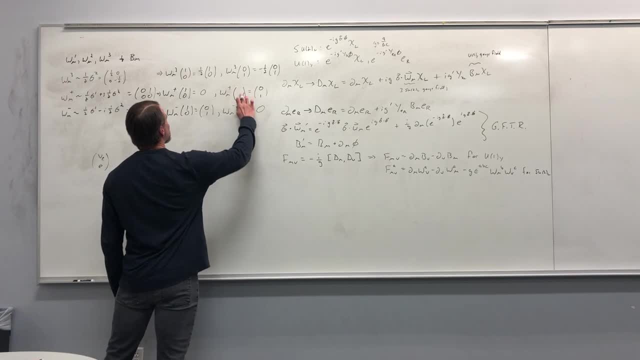 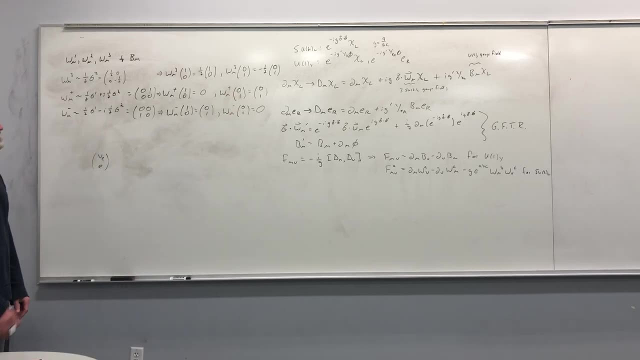 Oh sorry, Yeah, This is Sorry, I get so confused. Sorry, This is it acting on? Oh God, I totally did it backwards, Geez. Thanks for correcting me now, after I've already gone through this line. 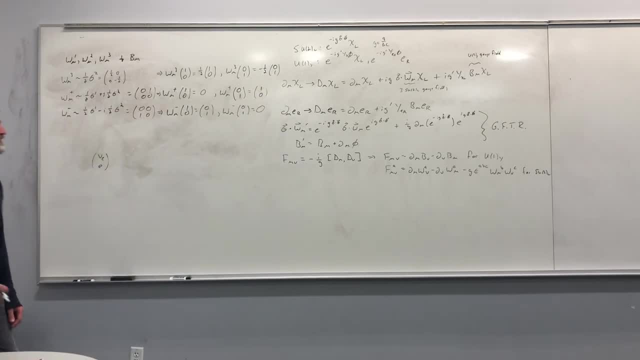 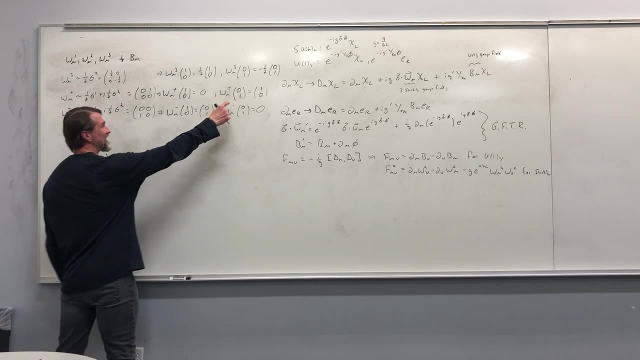 Jesus, Okay, Anyway, Yes, All right. So this is taking an electron and turning it into a neutrino. Now here's an important point. This is taking an electron and turning it into a neutrino. Now, here's an important point. 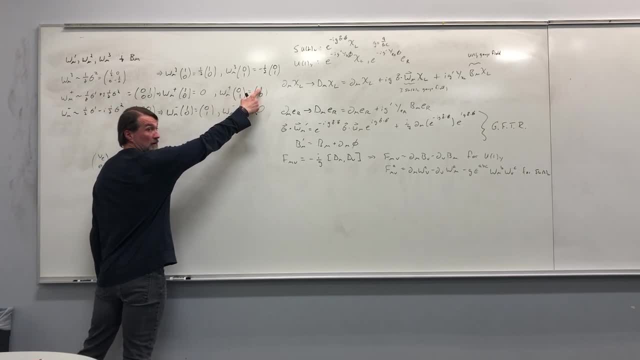 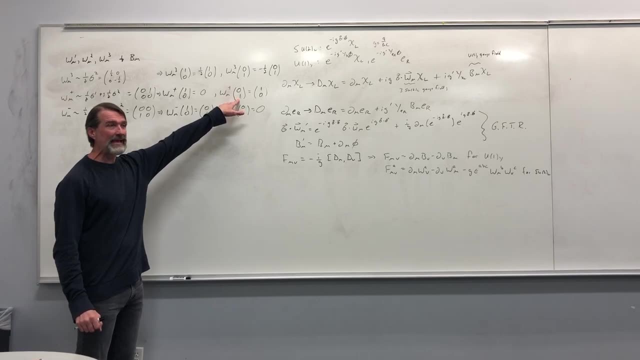 This is taking an electron and turning it into a neutrino. Now here's an important point. This is taking an electron and turning it into a neutrino. Now here's an important observation. This is taking a negatively charged particle and turning it into a particle. 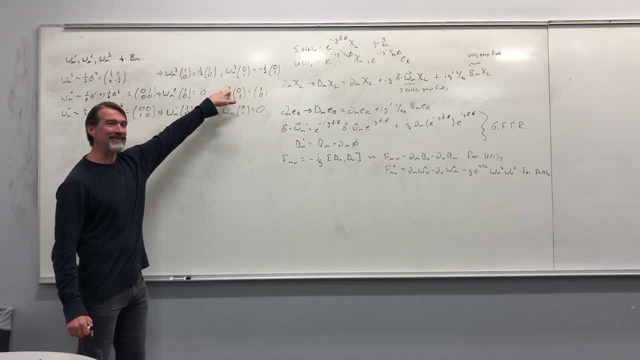 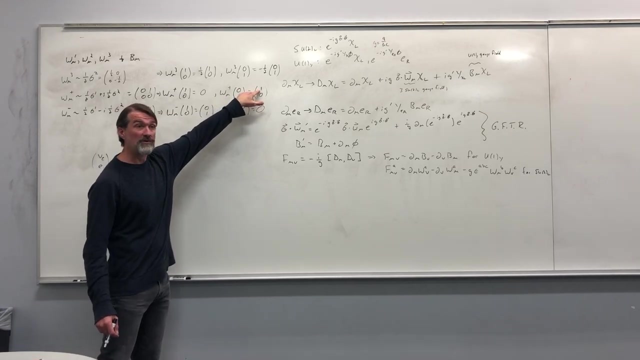 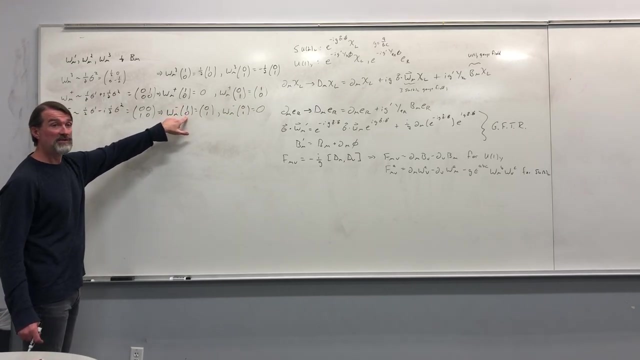 with zero charge. What does that plus mean? That means that this boson has positive electric charge. That electric charge combines with the electric charge of the electron to give me zero electric charge. Same as true here: The W minus acting on a charge-less neutrino. 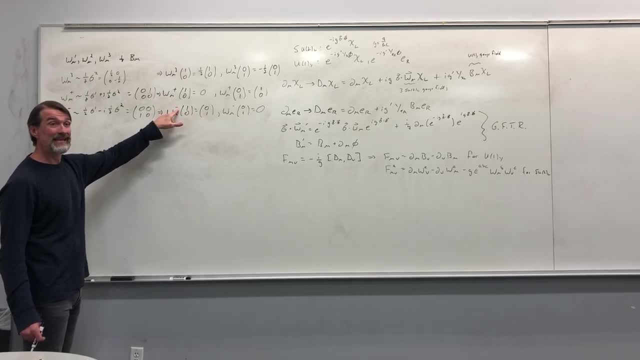 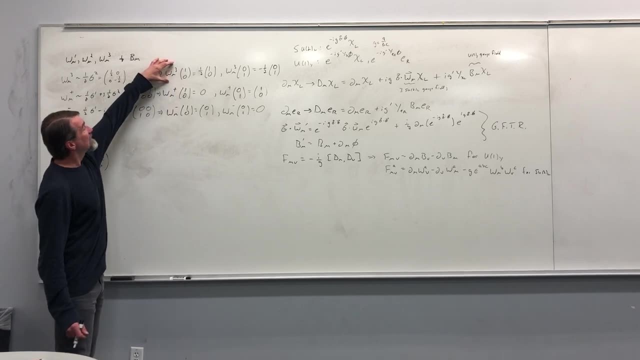 gives me a negatively charged electron. That minus is that this thing has negative electric charge. Okay, You can't do anything in this case. So notice: the W3 is electrically neutral, whereas W plus minus mu is charged. Okay, So now we have no interaction. 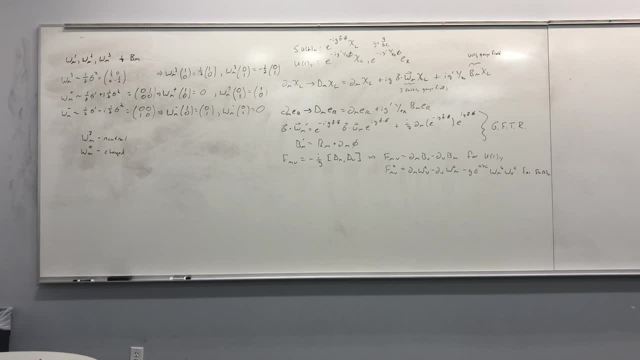 Okay, Go ahead, Okay, Go ahead. Well then, why do you get zero? Well, just Well, just Minus on. It's just because this, this boson, is not going to interact with an electron. That just means no interaction. 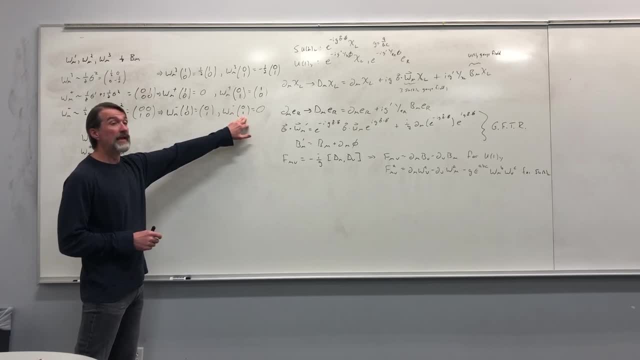 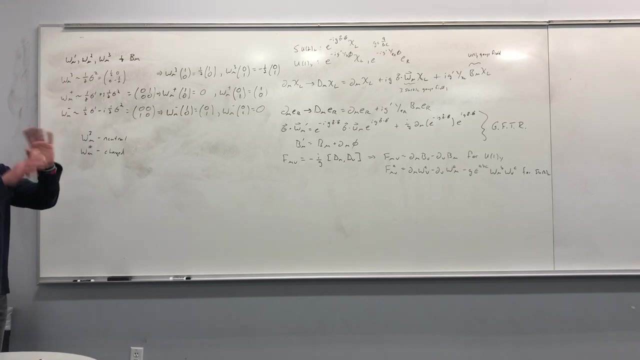 Yes, Okay, It doesn't. And no interaction here. It doesn't mean it made the electron go away. No, Yeah, Definitely Yeah, No interaction, Okay. So I just want you to notice We've been talking about that SU2 left rotation thing. 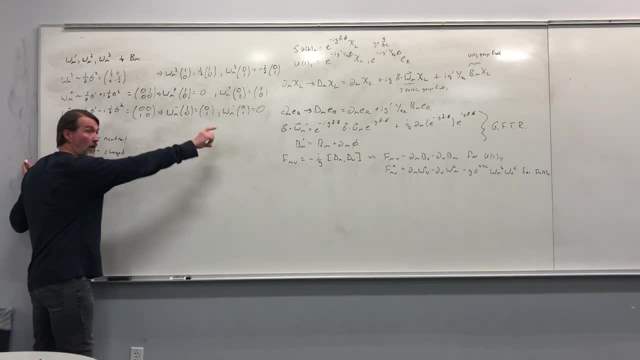 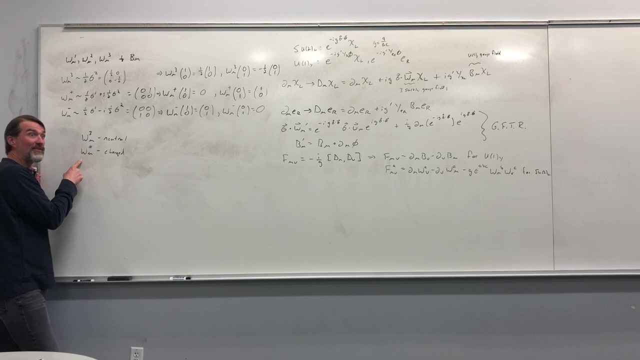 but what we've discovered is that the generators- that that requires two of them- come with electric charge. This also means that these two generators are going to interact with each other via the electric force, the electromagnetic force, because they've got electromagnetic charge. 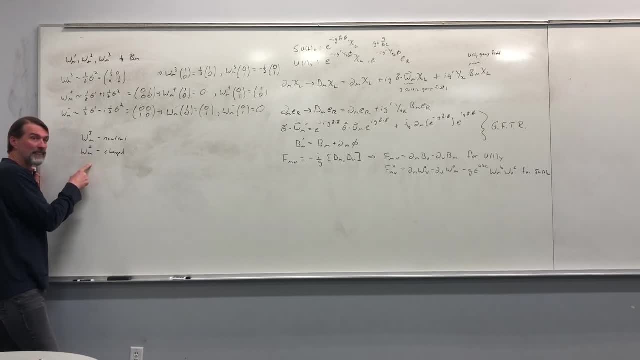 They can interact with each other via that, OK. So you see why having the weak interactions period automatically incorporates electromagnetism, because it's got charged bosons, all right, OK. OK, so we've got the neutral, We've got the charge. 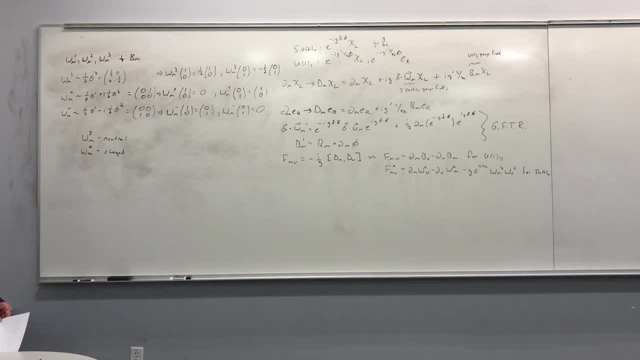 Now I've got five minutes to do my last problem. I have surgery. If you ask me a hard question, I'll kick you out of the room, but go ahead. Yeah, the easy thing is that. what means the negative, What emits the negative? 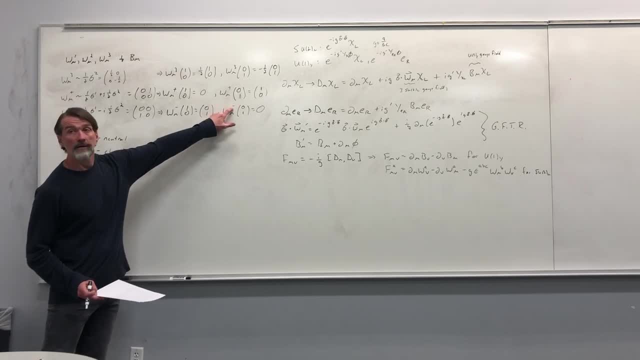 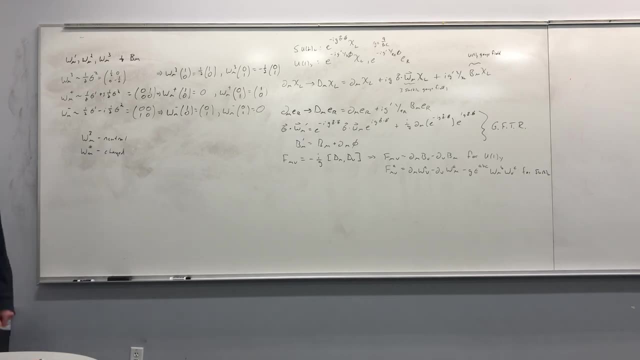 The negative has some meaning Here. No, in the first row, Sorry here. Yeah, yeah, yeah, That's just a coefficient. Don't worry about that. It's not important At the end I will do the other. 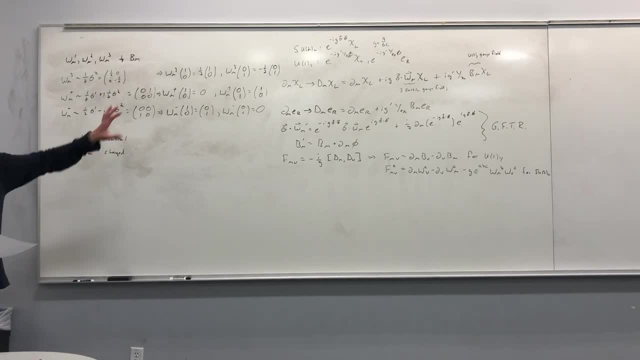 At the end of the day that's going to have some importance, but not nearly in this interpretation. in terms of plus or minus, It's going to have some minus electric charge. That's not going to be a part of the story. OK, 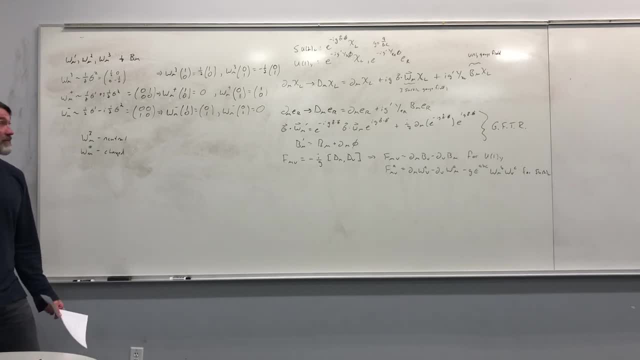 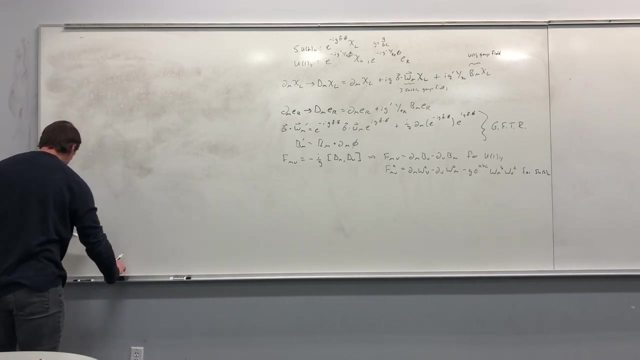 All right, are you ready? folks, I'm about to hand it to you. You good and ready? All right? yes, Here we go. We're done with the work. We've actually finished everything Now I want to make- it's going to suck that he left. 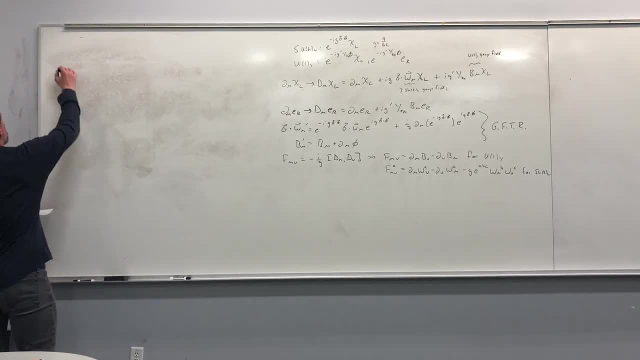 There are two big problems with this Problem. number one: the weak bosons, actually all of them. The weak bosons are massive, All right, All right. So the bosons affiliated with the weak interactions are massive. So the bosons affiliated with the weak interactions are massive. 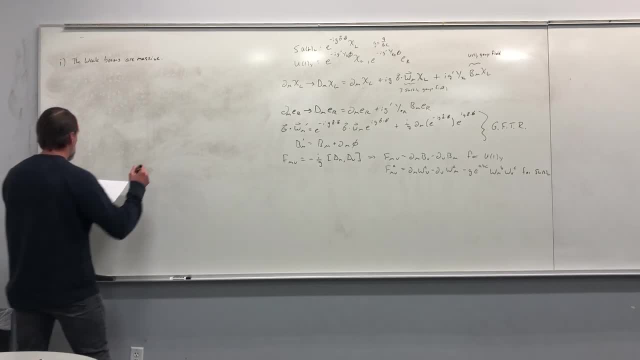 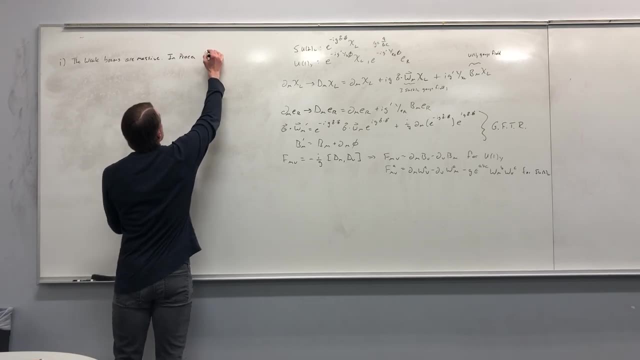 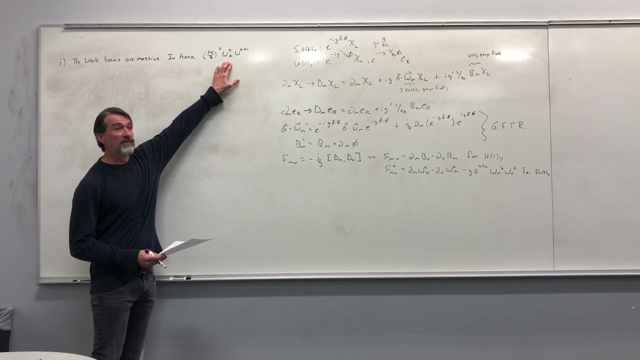 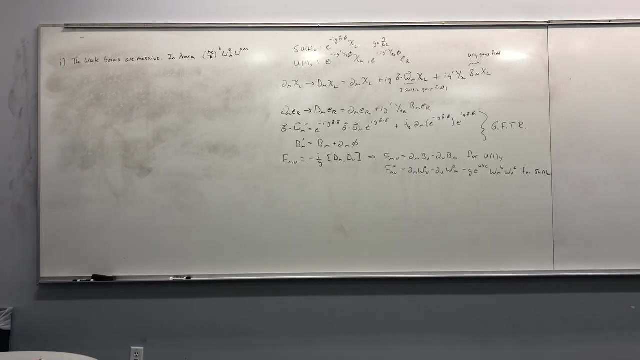 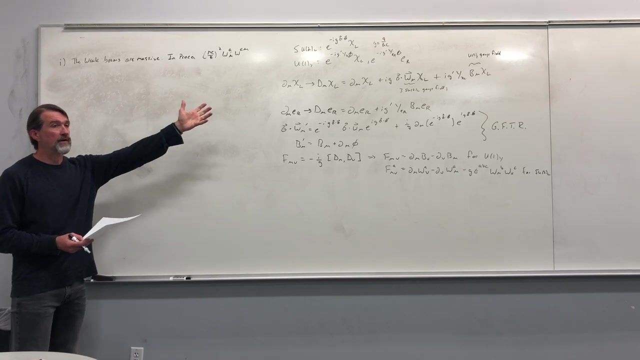 But remember, in the Proca-Lagrangian, if we had included this mass term, if we had included this mass term. this term is not invariant. OK, So we have a contradiction. We're trying to have this gauge symmetry based on a local gauge invariance. 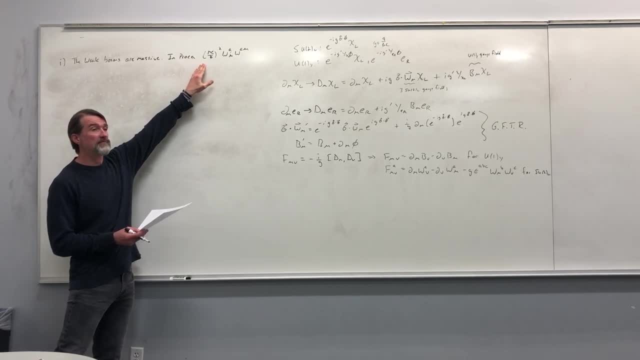 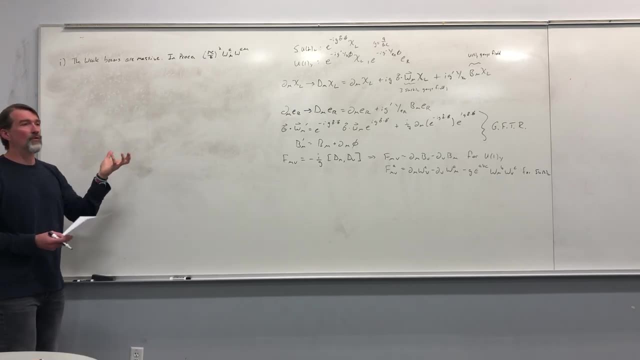 the construction of which requires the masses of the gauge bosons to be zero. OK, However, experimentally, we detect that these gauge bosons have mass. However, experimentally, we detect that these gauge bosons have mass. Therefore, either, there's no symmetry argument underlying it. 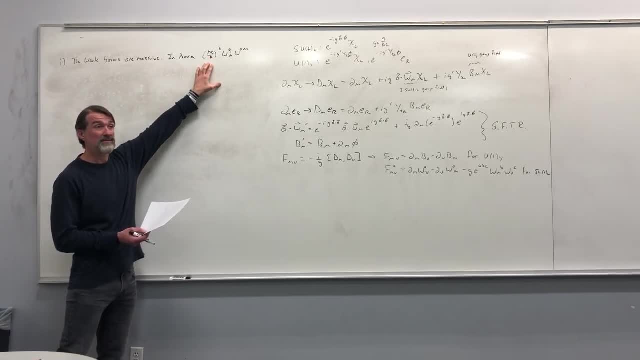 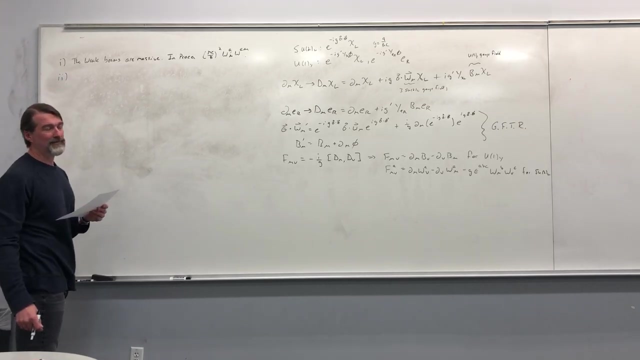 because the symmetry argument leads to zero mass prediction. but you're seeing the mass, Or there's some other fucker that's interfering in the story, I don't know. OK, All right, All right. Second problem: Bigger, Way bigger. 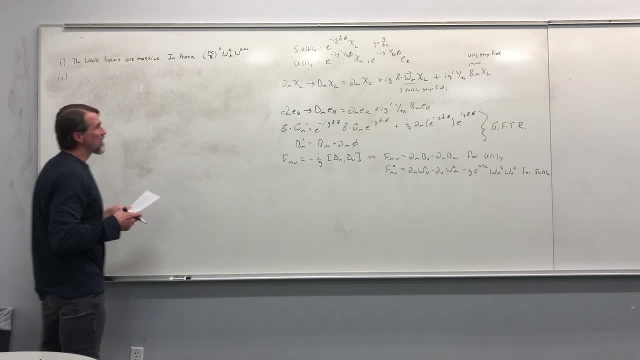 Way bigger. Remember that – it's gone, I've erased it, But anyway. Remember for matter – I'm talking about the stuff we're made of. Remember for matter – I'm talking about the stuff we're made of. Remember for matter – I'm talking about the stuff we're made of. 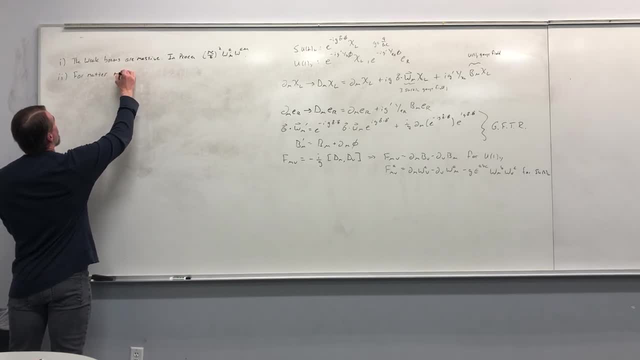 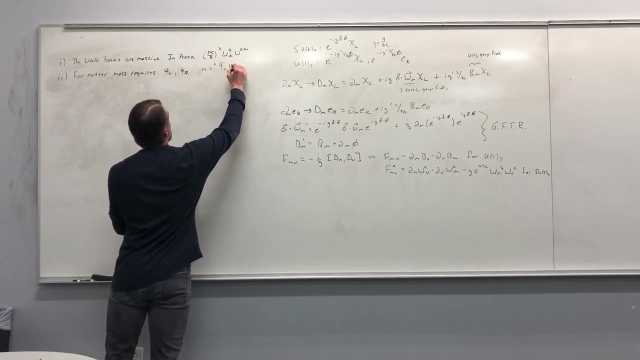 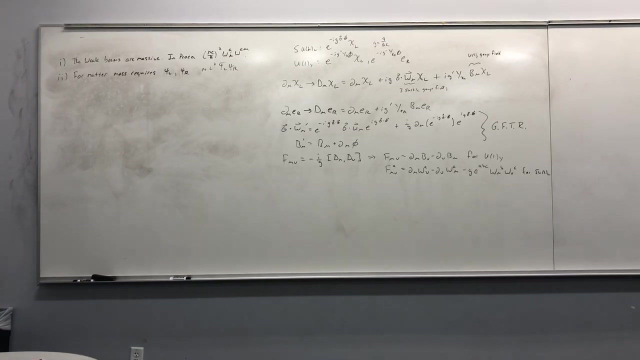 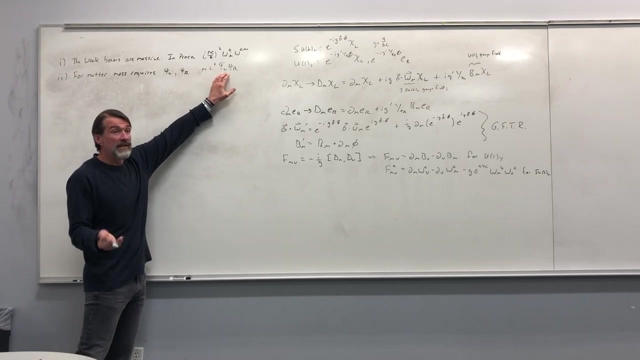 Mass requires psi left and psi right contributions. Okay, remember the term is mc squared, psi bar left, psi right, as an example. Well, that's fine, though Matter, you know matter- has mass, most of it does. So you just have the left and the right contributions, right. 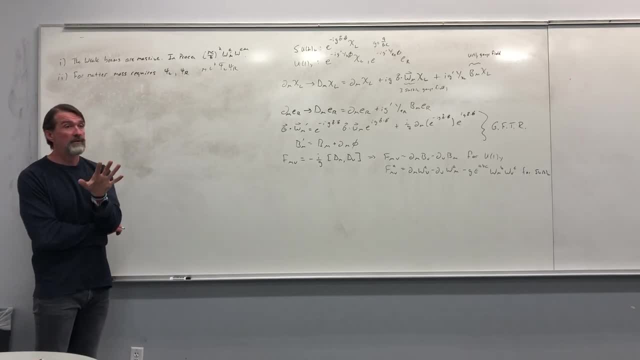 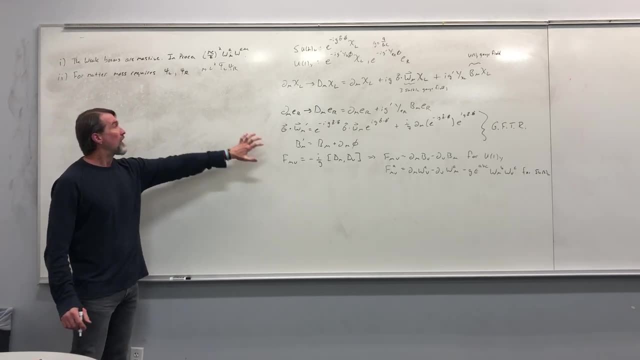 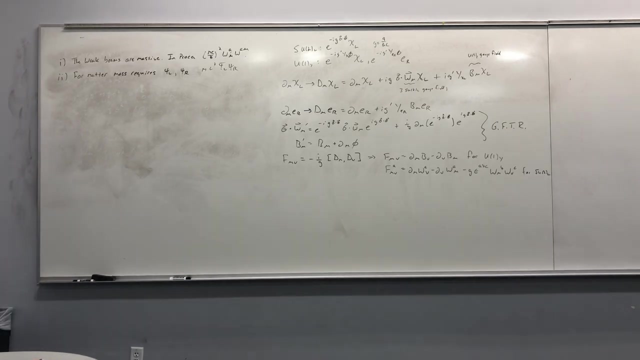 Make sense. Here's the problem. Before today, all of the symmetry transformations we've talked about, there was no left and right parts of the story. Today, however, there is the left versus the right version of the story, And the left symmetry is different than the right one. 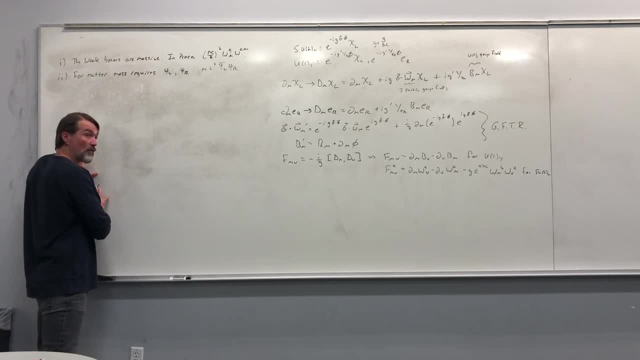 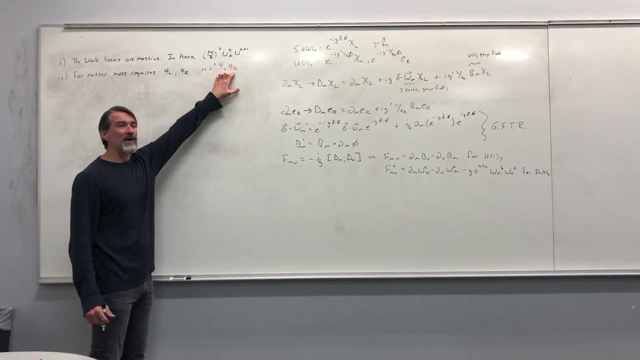 The left is su2 left, the right the other one is au1, which acts on both. So my question is: is this term right here invariant under su2 left? No, it's not Because you can fuck around with this, but you can't touch this with su2 left. 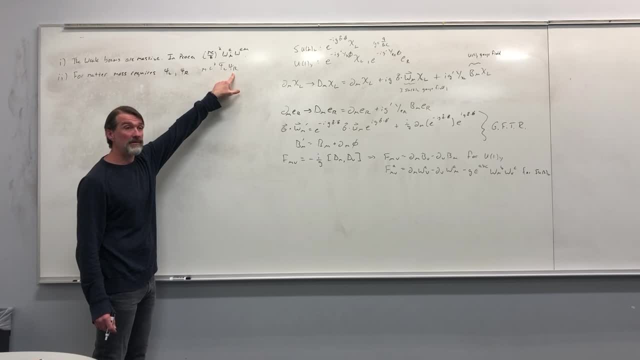 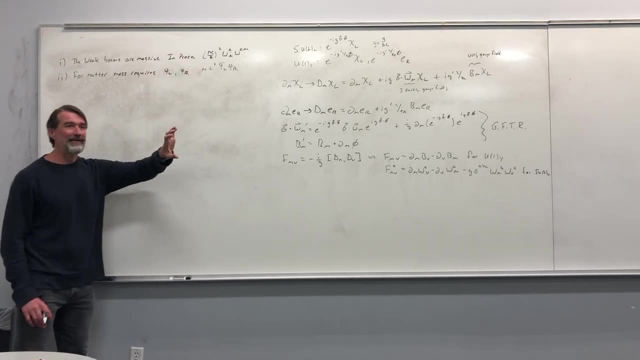 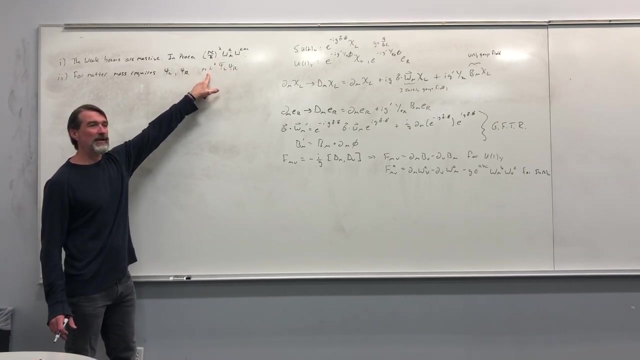 So you can take this and transform it into something which is not the same. So for su2 left to be a good symmetry of the theory, not only do the gauge bosons have to be massless, but every single matter particle must be massless. 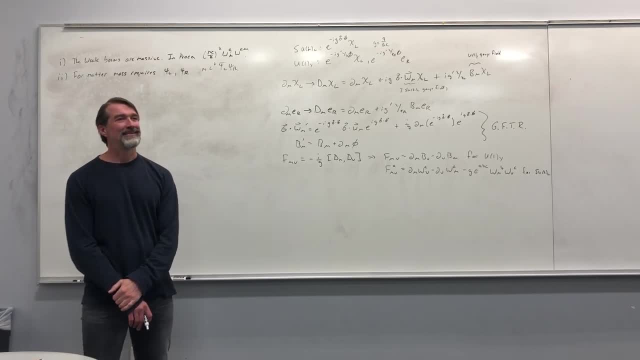 Well, let's think How many particles are massless? Three, The three neutrinos, Not the electron, the one on the top, one on the up down, strange top bottom quarks. So we have a problem. 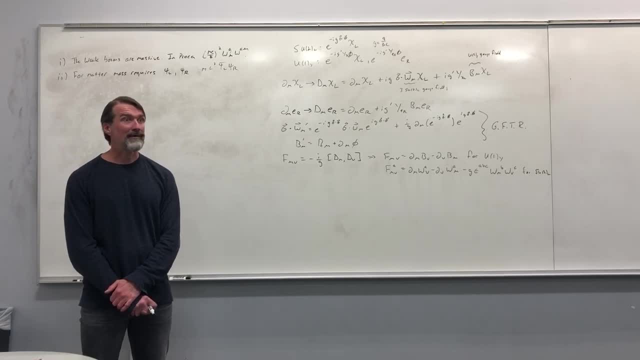 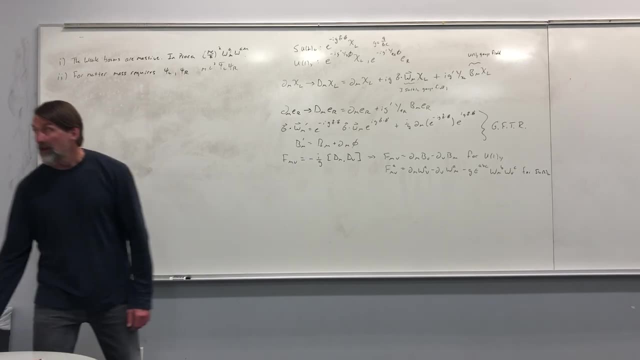 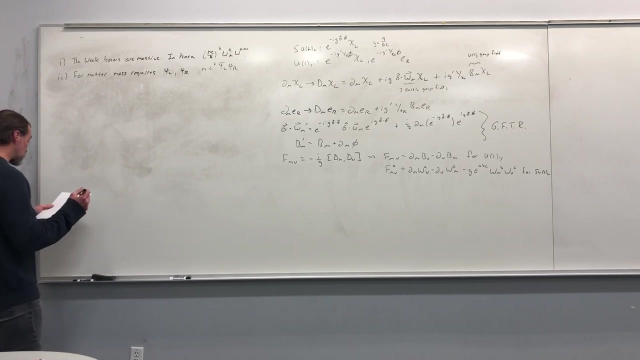 It's all about mass. It's all about mass. The Higgs mechanism is going to solve it. Okay, I'm going to go to that next time, but I'm going to finish this lecture with a quick discovery: Su2 left when we do the Higgs mechanism. 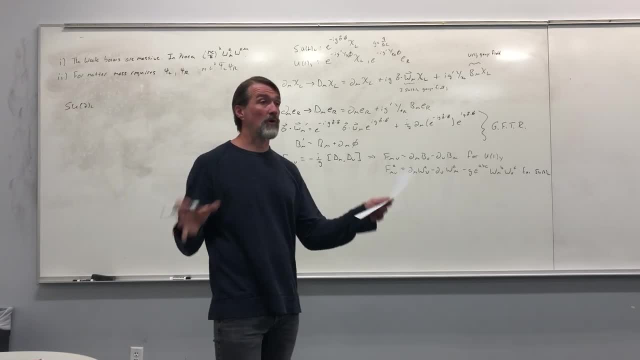 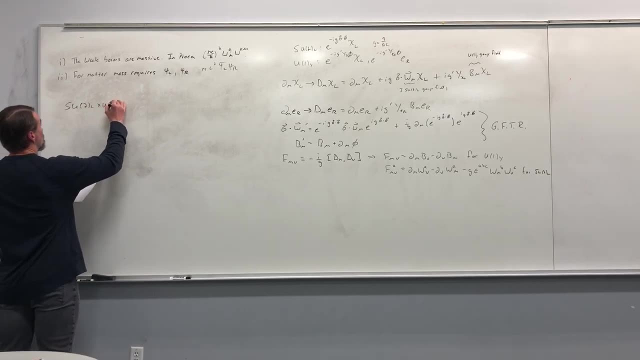 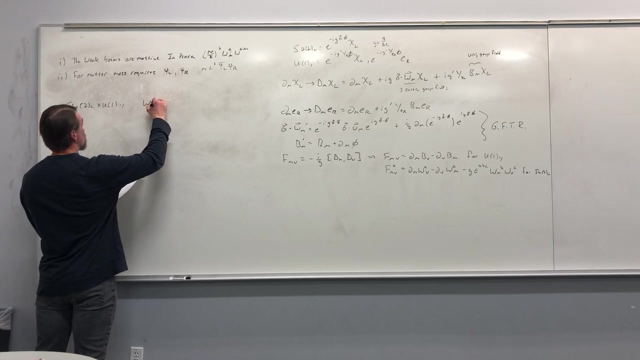 I don't think we're going to apply it directly to this example. We'll do a cartoon example, because applying it to this is a real headache. So I just want to go over a quick result. This thing has four generators. obviously It's got the w mu3, 3w plus minus mu. 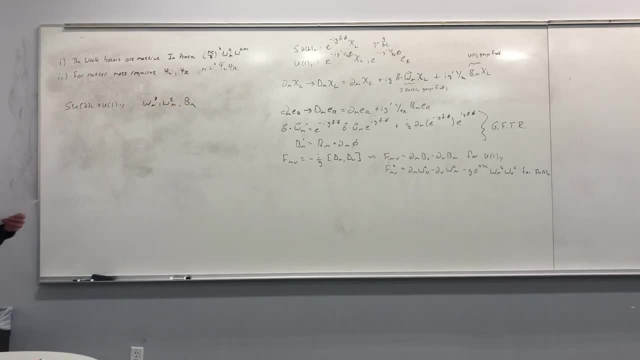 and then we have the b mu for the u1 hypercharge, And then what we're going to do is we're going to take this su2 left and we're going to break it down to u1 of electromagnetism. Okay, 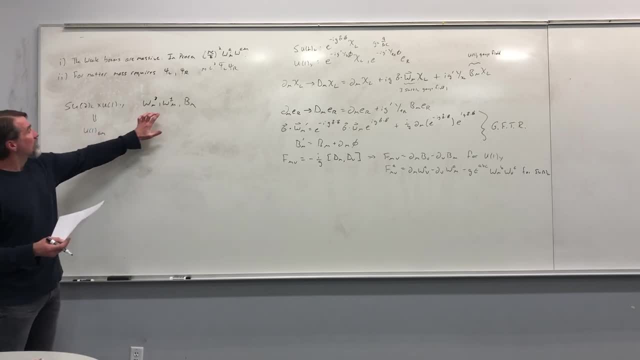 So when we break this down to u1 electromagnetism, we're going to have a single generator and a single associated gauge field corresponding to u1, E and M, And the question is: which of these four generators and associated gauge fields might it be? 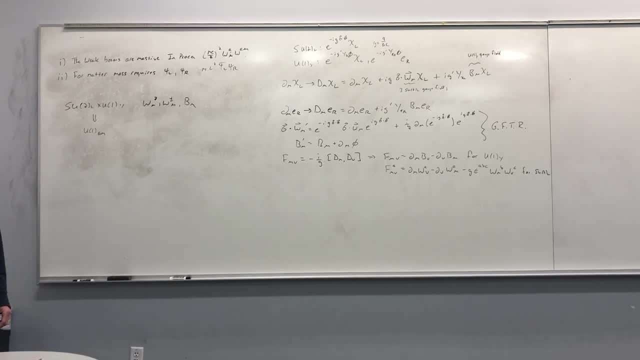 Any takers Say it again: Probably the plus minus one. Oh wait, that's two. Yeah, this is two, this is one, this is one. So this is for u1 hypercharge and these are for su2 left. 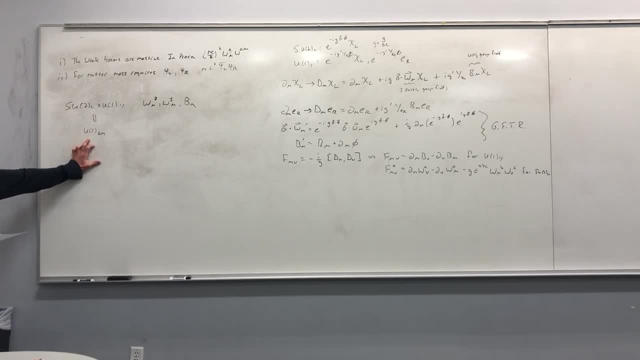 So which one do you think is going to be the associated gauge field for the electromagnetic u1?? It turns out that the gauge field associated with u1 electromagnetism, which is just the photon field- okay, coming from this story, it's actually going to be. 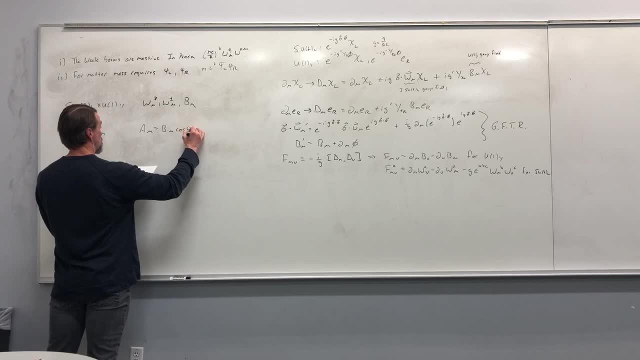 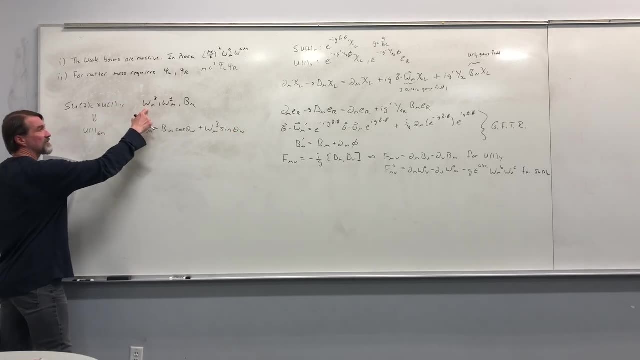 a mu is b mu cosine theta w plus omega mu3 sine theta w. It could only be a combination of this one and this one, because these are electrically neutral and we know photons don't have charge. These can't be part of the story. 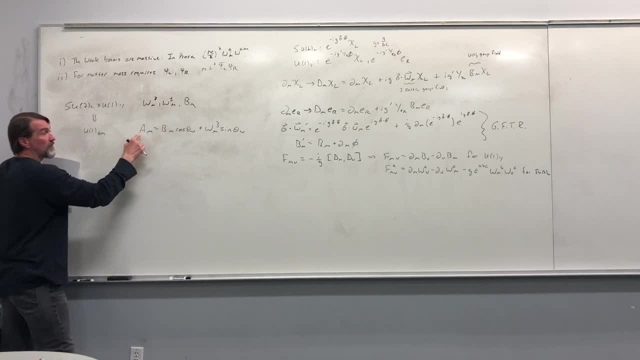 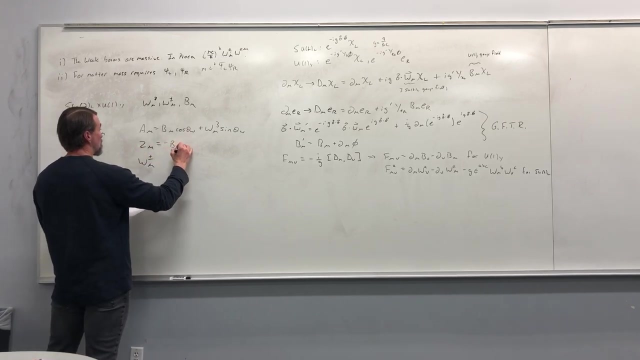 Okay, So the photon field, the gauge field associated with the photon, is just this linear combination of these two neutrals. And then it turns out that in the resulting story we basically have another neutral which corresponds to minus b, mu sine theta w, plus omega, mu3, cosine theta w. 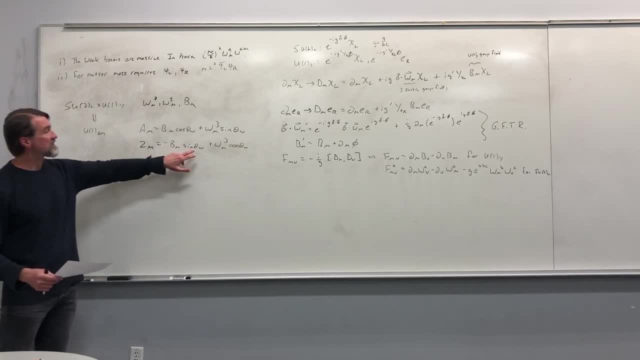 Okay, So these are just two independent linear combinations. The theta w is called the Weinberg angle, and that's the angle which is telling you how much these are mixing. Okay, And then the w plus and minus. they just descend into this story. 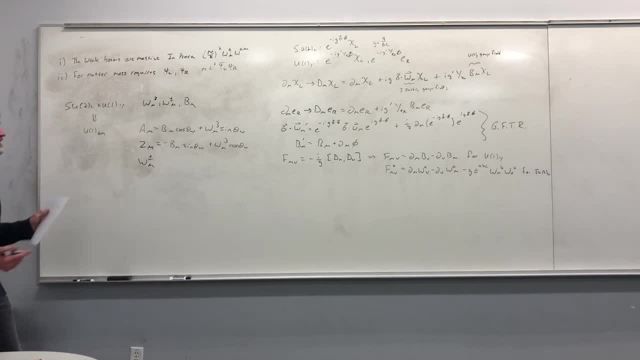 So what we're going to find when we're doing calculations is that we have the gauge field associated with electromagnetism. We have a neutral gauge field, which is part of this story, but it's not just part of this or this. 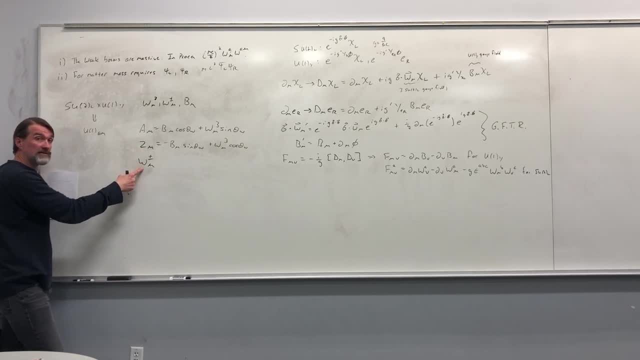 It's kind of a little bit of both. And then we have the plus and minus gauge fields. The three of these are massive. This one is massless. Obviously, the photon is massless. Okay, Now just one last really quick thing. 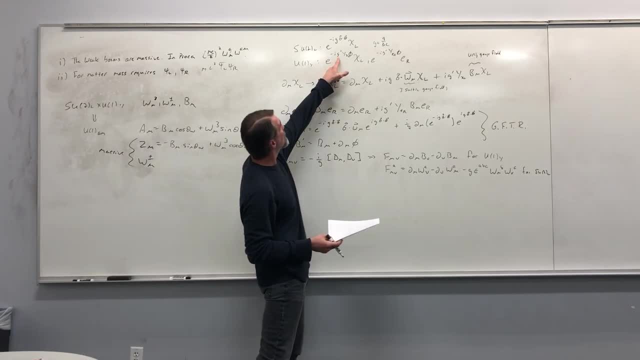 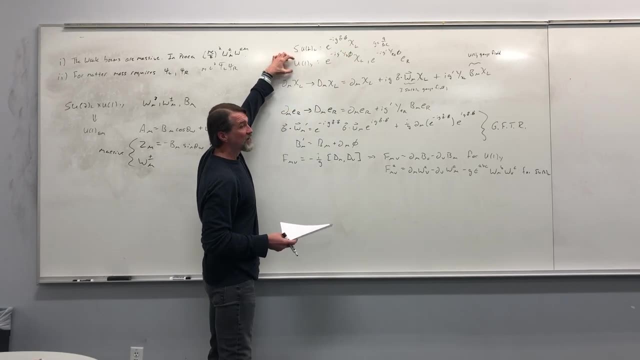 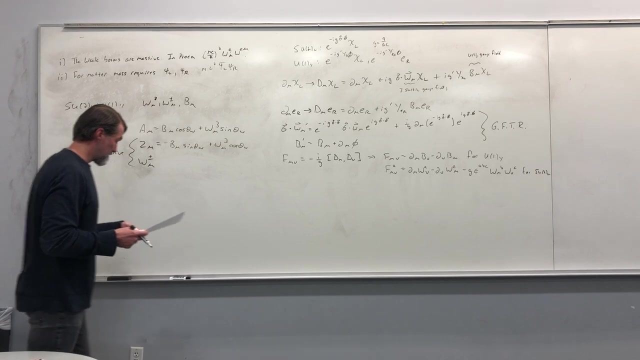 The fact that this had a coupling g prime and this had a coupling g would tell you that these two transformations are not unified. There's just two separate groups. It turns out g is related to g prime. Okay, In fact, what we can say is that g times sine of theta w. 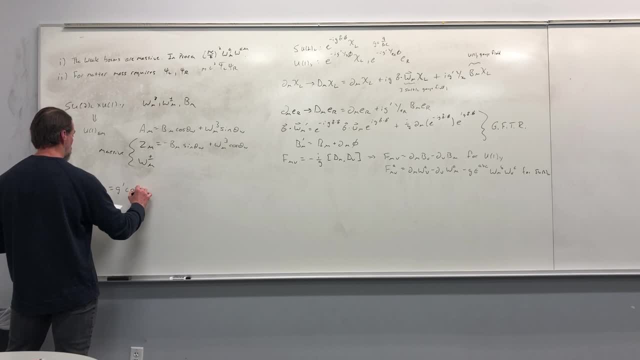 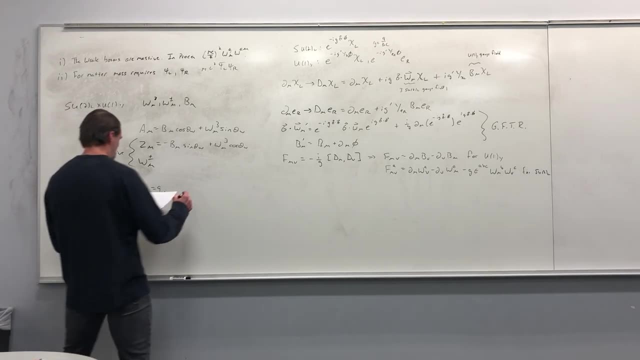 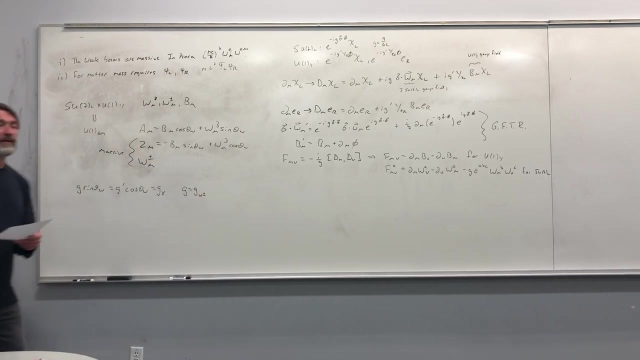 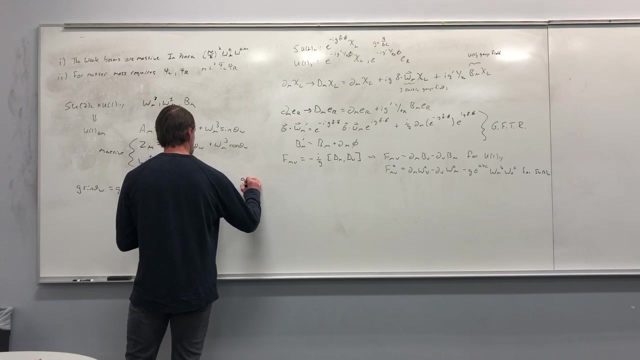 is equal to g prime times cosine theta. w, which is the coupling of the photon to electric matter. Okay, And then the g in the story is also the coupling to the plus and minus weak bosons, And then gz is g- gamma over sine theta, cosine theta. 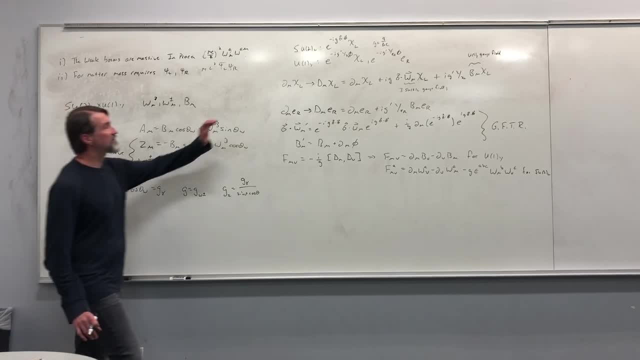 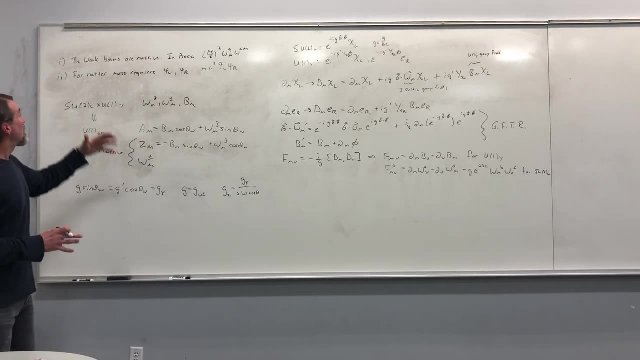 Okay. So all I'm trying to show you is that there was really and truthfully, only one underlying coupling in this entire story. That's why we call it a unified force. It's kind of weird, because if we write su2, actually let's do this. 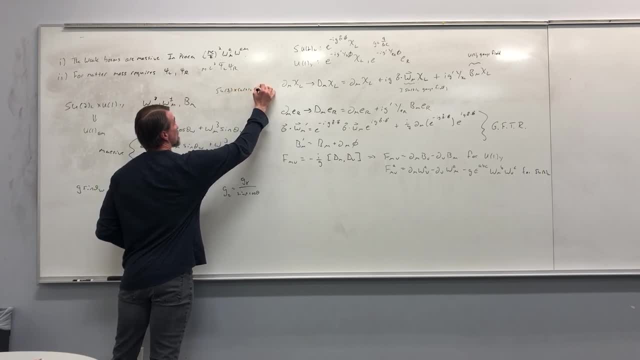 Let me say su3 cross, su2 left cross, u1 hypercharge, And I argue: this is not part of these forces, This is independent. It's because this has a coupling which is completely unrelated to these couplings And this group which, although it's a product of two groups, 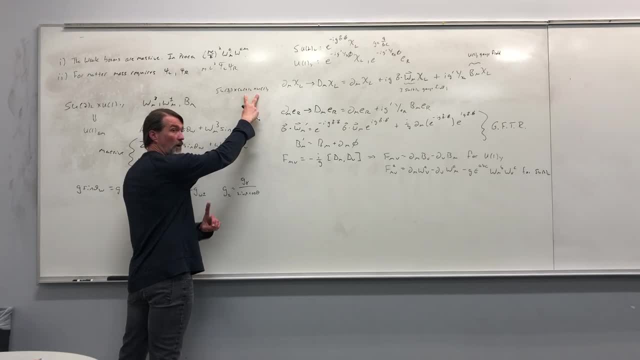 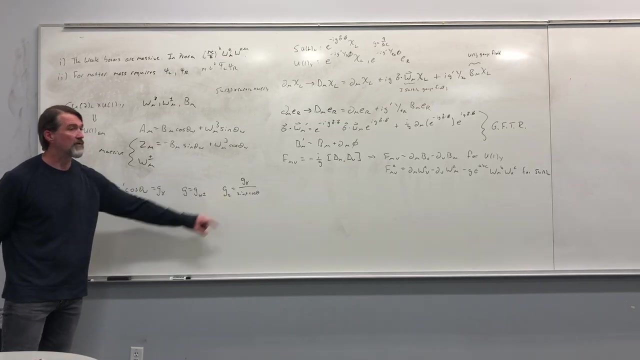 it only has one coupling, So there's really only one underlying interaction. It just has this weird symmetry form. Okay, Yes, What's the substitute for the last g, z? This is the coupling for the z component, So the g everywhere. you see it.